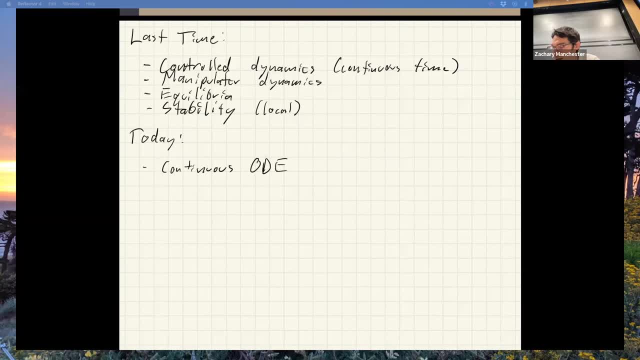 optimization with this stuff is figure out how to take those continuous time ODEs and map them into discrete time maps for simulating stuff and running things in a computer, right? So we'll call it discrete time simulation, say. By the way, I found it is extremely common for 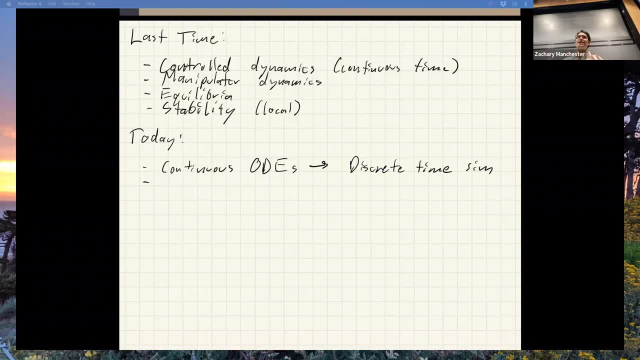 there to be among computer scientists. there's this hang up where people sort of like differentiate between the word model and the word simulator. These are the same thing And they will be. those words are interchangeable as far as we're concerned. in here, I think, like in the RL, 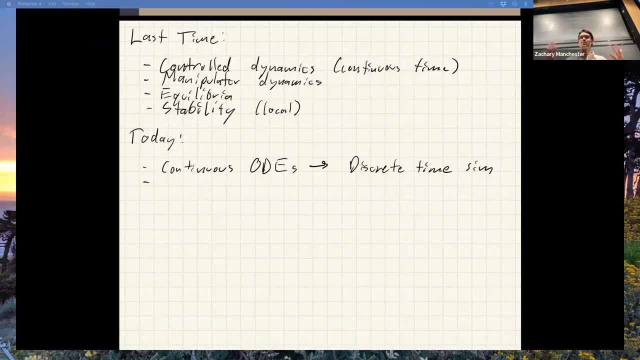 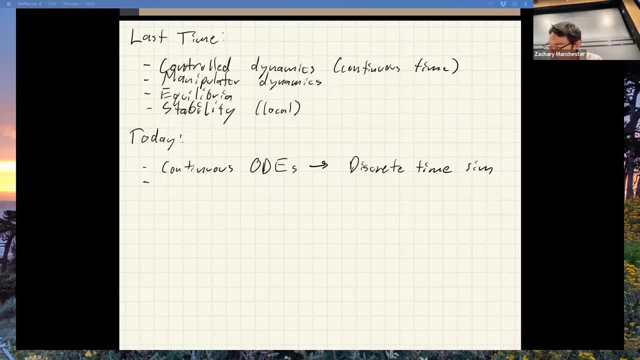 model and simulator are the same thing, Cool. And then we're going to do more stability stuff in discrete time and also as part of this discussion on discretizing ODEs and simulating them, Because there are demons lurking in there. If anyone has done this before, you'll know what. 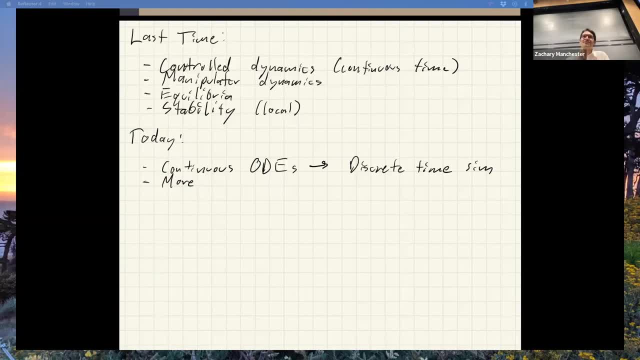 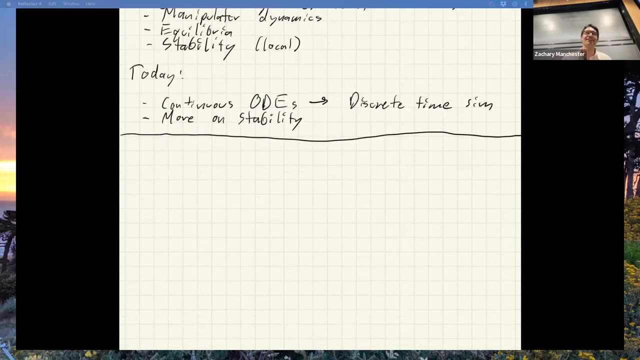 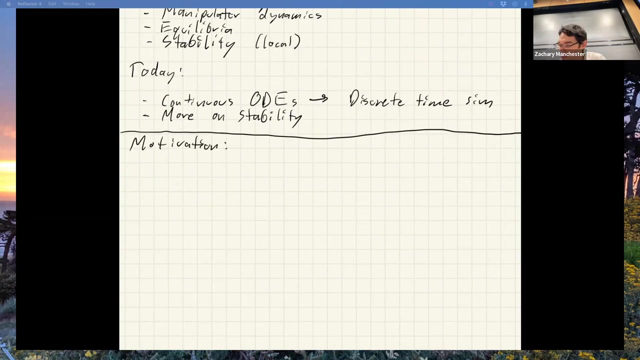 I'm talking about. We're going to pull the lid back on some of this and show you where the demons lurk today. Okay, they. and the punch line on that is: never trust your simulator, always be skeptical of your simulator. Alright, So so the kind of motivation for what we're going to talk about. 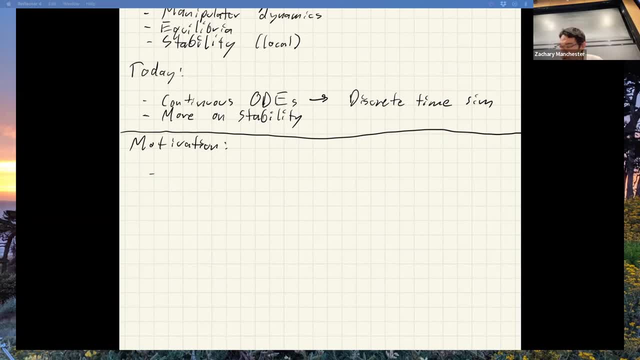 As everyone who's taken a course on differential equations will know, in general We cannot solve. X dot equals f of x for x of t. We can basically only do this for the very special case of linear differential equations. It's a non-linear ode which is everything interesting, from robots to spacecraft, to airplanes, to whatever you care about. 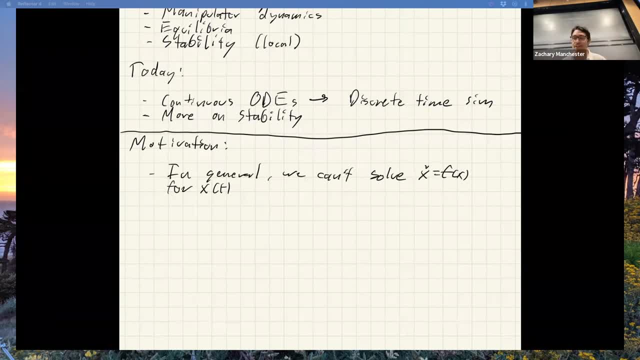 It's non-linear and there's no way of solving that thing analytically. So then we got to get it into a computer and also as part of that we need to. you know, computers can't deal with, you know, continuous things like continuous functions. 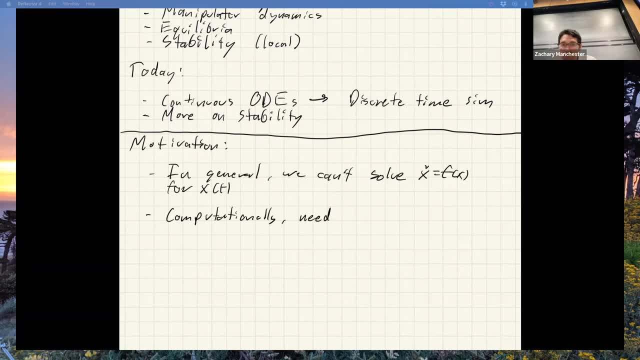 We need to represent this somehow with discrete values in a computer, right, And I just create values, I mean like discrete time steps or whatever right. we can't have this like infinite dimensional, continuous time thing in our computer right. Okay So, and then, as a kind of an aside, that is interesting that we will get into later, 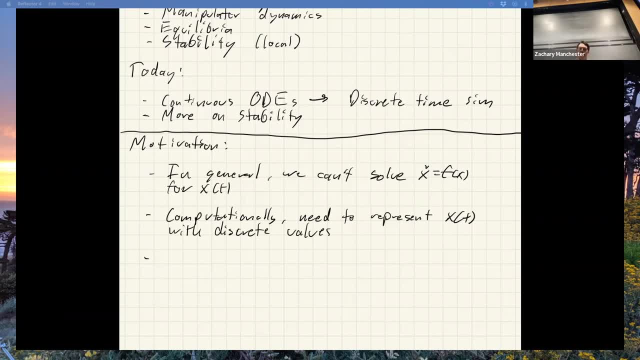 There's certain sense in which discrete time models or discrete time Mappings are actually like more general and connects can can express things that these continuous od's can't because of certain smoothness assumptions, just the very idea of a differential equation. This comes up when we get into, like contact dynamics where you have these discontinuous impact things. Those can't be written down as ODEs but they can be written down as sort of discrete time maps, which is kind of interesting. 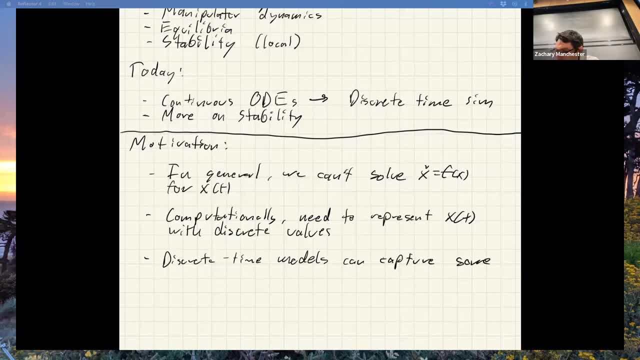 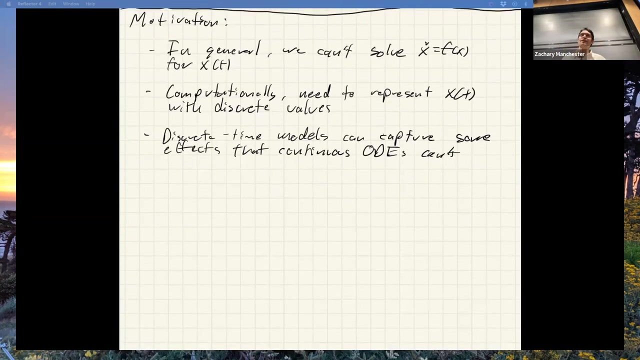 All right, Yeah, I mean that kind of goes along with the very idea of you know, impacts being non-differentiable, right? It's in the name: differential equation. So if the thing is, if x of t is non-differentiable, its derivative is not defined. I can't write down an ODE for it right at like a very basic level. 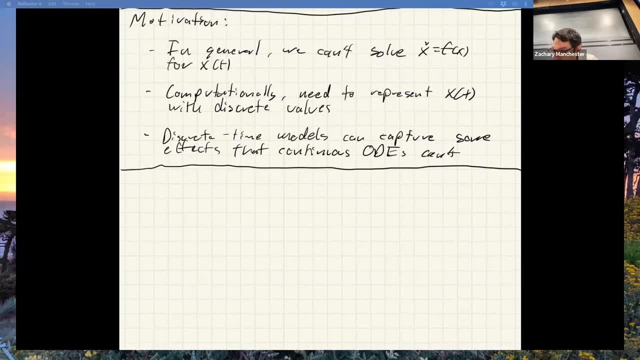 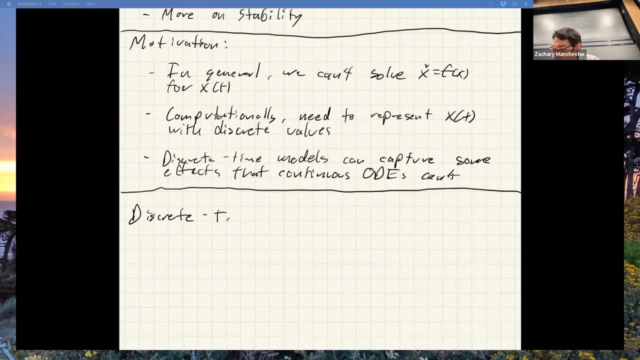 Okay cool. So discrete time stuff: Something bad happened. Okay, Discrete time dynamics. So the first thing is, there's kind of a few ways of writing these down. So we'll first talk about explicit discretizations or the kind of explicit form of these things. So that's where you have an equation for xk plus one. 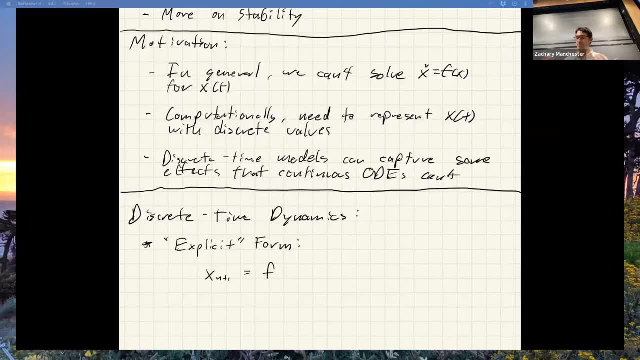 as a function of and so on. just for today, to differentiate between the continuous f that we talked about last time, we're going to put a little subscript d on this guy for discrete time. So we have xk uk, So these are right discrete times, So we have some time. step here: 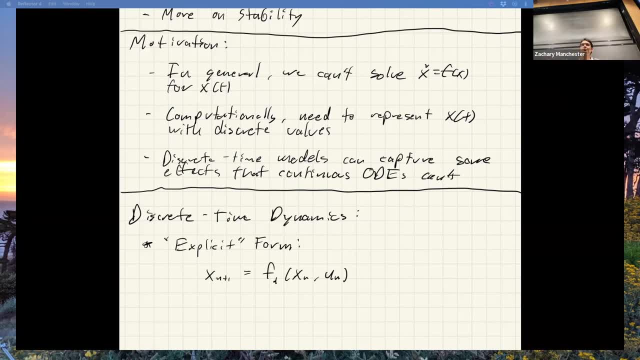 And we're going to have a function- f sub d, discrete f- that eats x at the current time, step u at the current time step and spits out x at the next time step right. So this is an explicit discrete time model. The d subscript will be discrete for today. 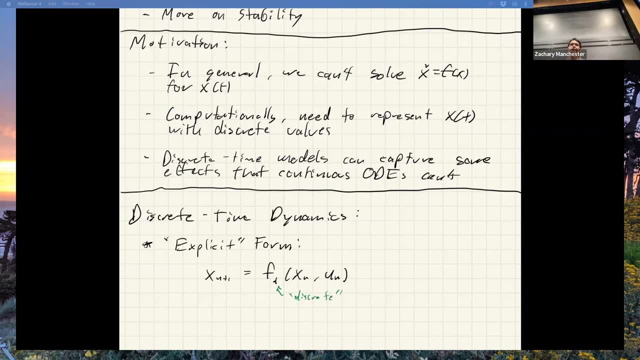 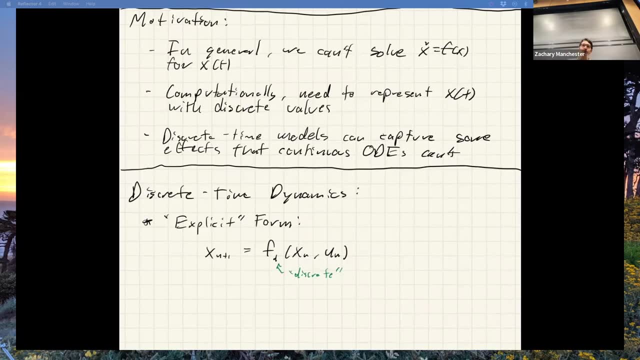 After today. we're not going to. Basically, everything will be discrete time after today, so we will drop a little d in the future. Okay, So that's. There are many, many ways of getting an explicit discretization like this. 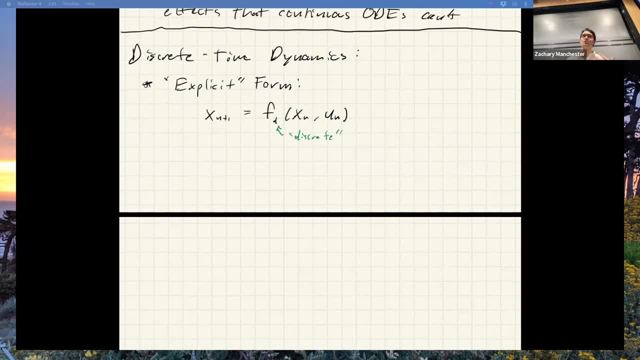 First thing we're going to talk about is the simplest one, which I'm sure pretty much everybody has seen before, which is explicit or forward Euler integration, Okay, Which looks like this: So you get xk, You just take the f, the continuous f, which gives you x dot, and you take a little step along the x dot direction of length h, which is your time step. So that looks like this: 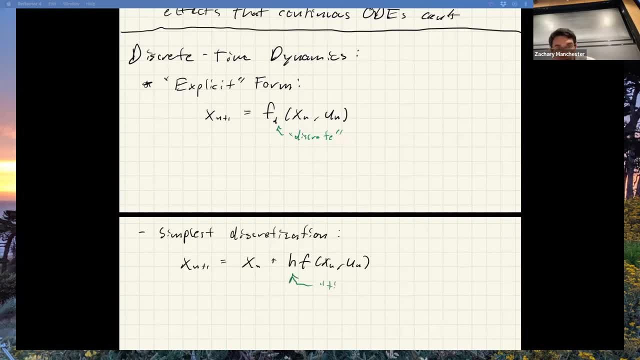 This h is your time step. I guess that doesn't need to be in quotes. And then, yeah, this whole thing is called. So this whole thing would be your fd now. and this is called forward: Euler, Who's done this before, Hopefully like everybody, right? Okay, cool. 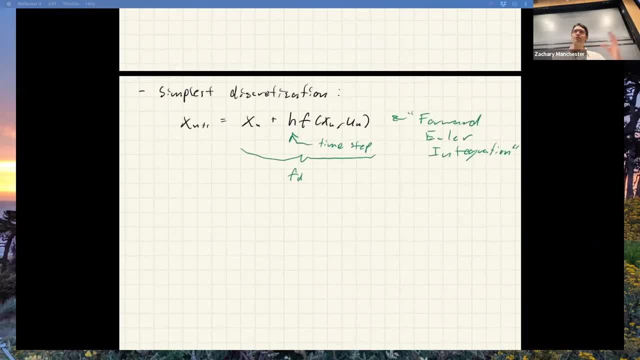 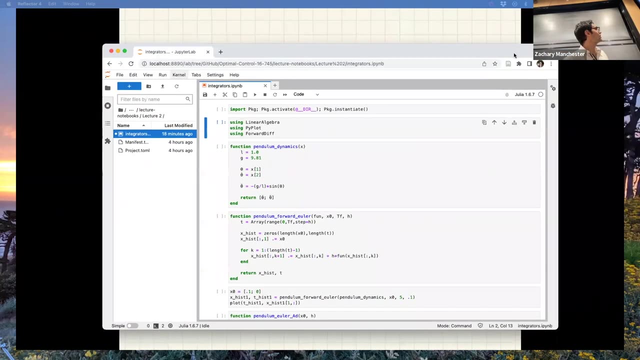 Okay, So, Okay. So what we're going to do now is do this on our favorite nonlinear system, the pendulum from last time. So let's go check that out and see what happens. Okay, here's our Jupyter notebook. 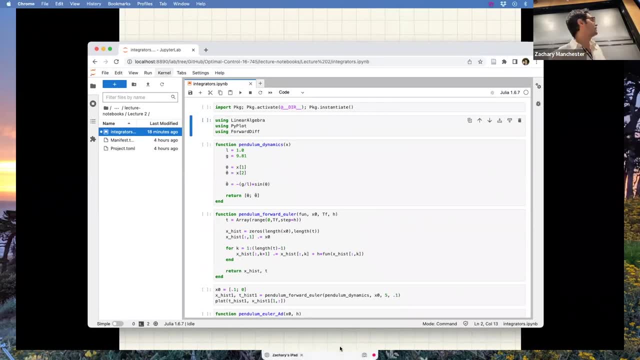 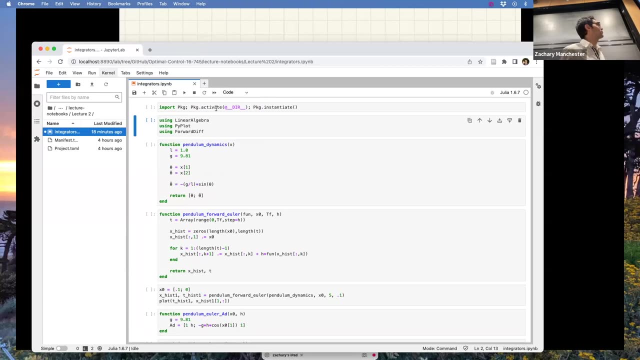 So I'm going to post code for all these things. I'll post these notebooks all the time. This is Julia. It looks pretty much like MATLAB. as long as you don't do anything fancy- and we will try to avoid doing fancy things- 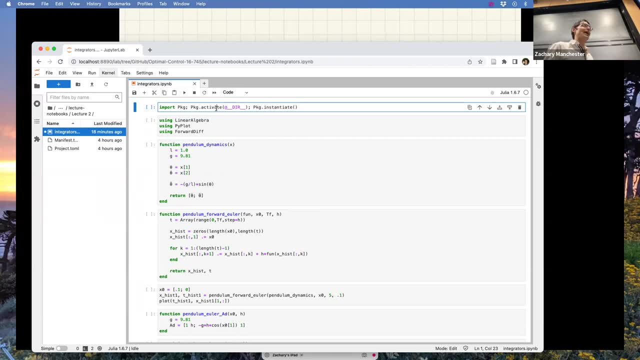 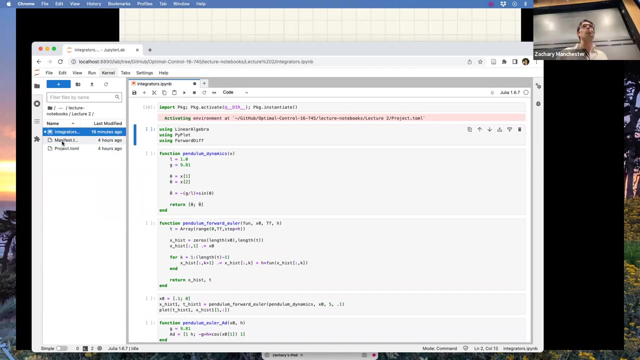 Things that it has that are better than MATLAB. it has a real package manager, which is amazing with like versions and stuff. So that's what that top line is. The top line is using the package manager to So these two files over here, this manifest file and project file. they have all the dependencies for the notebook with version numbers. 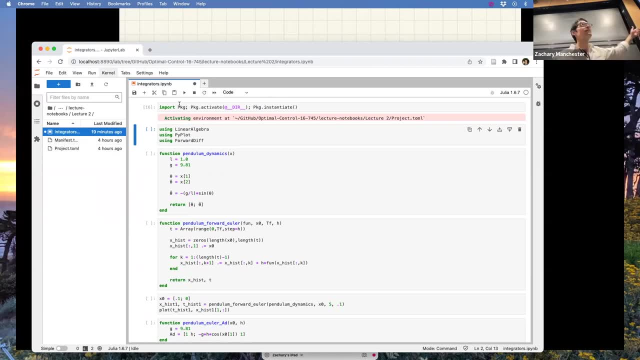 So I'm just going to post this all on there. When you call this first line, it's calling the package manager and it's telling it to install the exact same versions of all the dependencies that I'm using in this notebook. So there should be no problem. 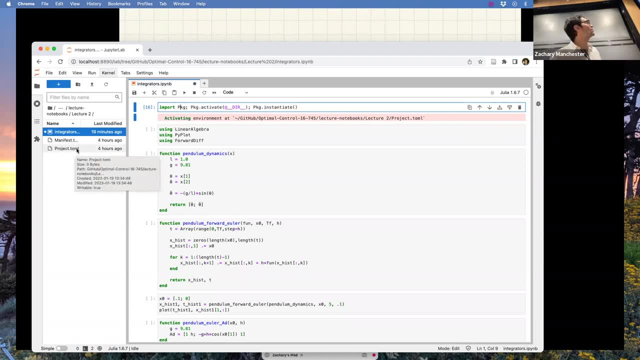 There should be zero compatibility issues for all of you, which is fantastic. The only thing I'll mention here, on the Julia side of things for the class this semester, we're using the long-term support release of Julia, which is 1.6.7.. 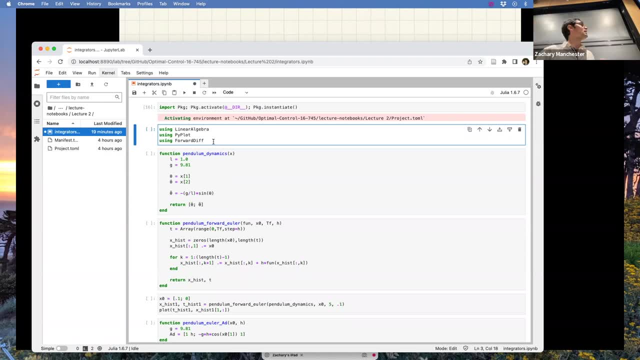 There's a newer version, which is 1.8.5, is the current release. We're going to use the long-term support version because there are fewer issues. If anyone has a Mac- M1 Mac or whatever- this version is x86, and it runs fine in Rosetta, which is what I'm doing. 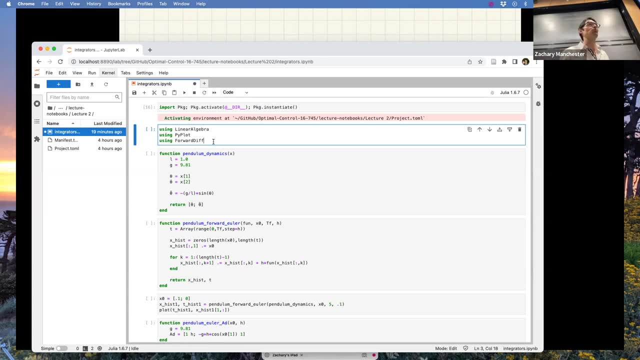 So you should have no problem. Just install the like standard x86 build. It'll work. Don't do anything weird, basically, and everything should be cool, which is why we're using the LTS release and whatever. We don't have issues. 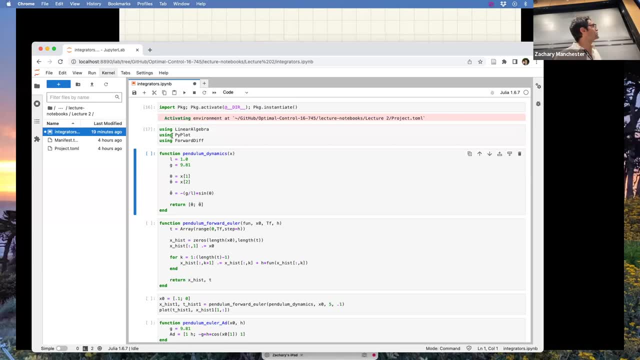 So yeah, this is just packages. I'm using Linear algebra is obvious. Pyplot is the exact same you know plotting library. It's matplotlib from Python, so it should be very familiar with most people. And then forward diff, which we'll use a ton in the class is automatic differentiation. 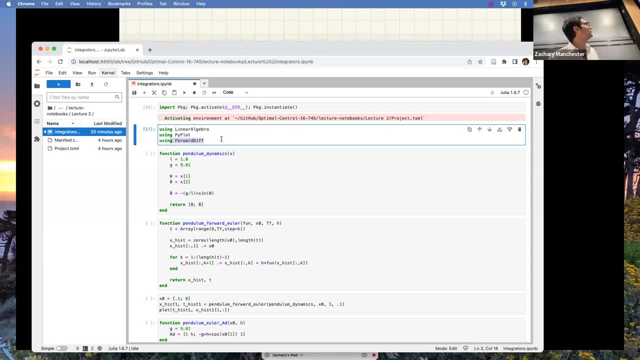 So I don't have to hand write derivatives, which is also fantastic. Yeah, Julia, So there will be homework zero. actually is going to basically cover how to use forward diff And some of these things in some amount of detail for you guys. 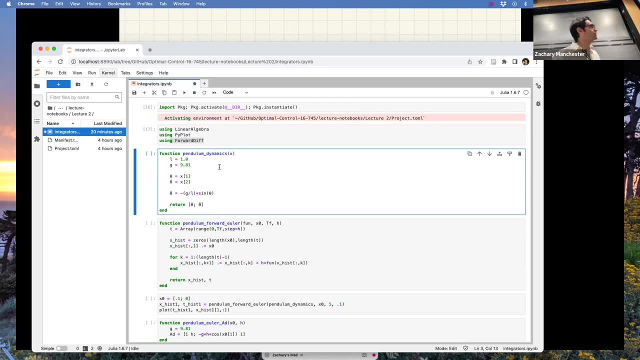 And that should be getting posted today Also. should be easy, OK. so here's our pendulum dynamics that we wrote down last time, with length equals one g 9.8, right, And that's it, right. Oh, we maybe didn't talk about this last time. 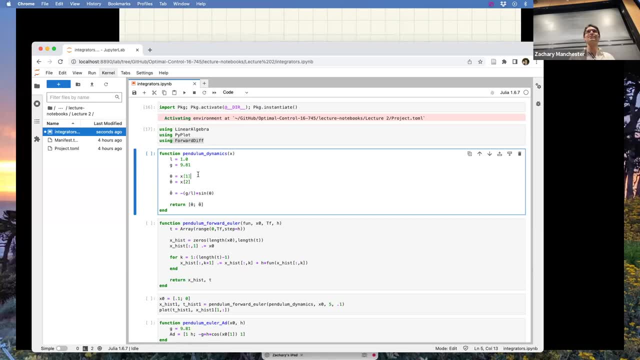 The mass cancels out in these equations and doesn't matter. Yeah, probably most of you have seen this, so I should have mentioned that, probably. But yeah, so here's what theta double dot is right, I have m, you know, ml squared, whatever. 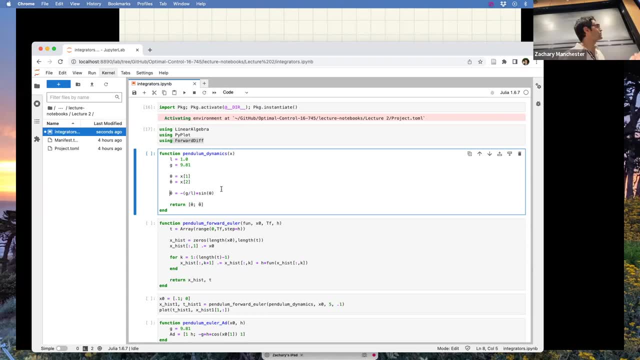 And If I divide through both sides, the m goes out away. right, The only things that matter are g and l, But this is just the dynamics you wrote down last time. right, Where the state is theta, theta, double dot. 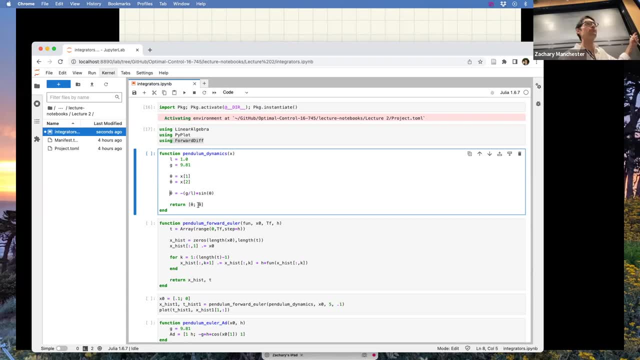 And this function returns x dot, which is theta dot, theta, double dot, right, Cool Yeah. How do you add this? Oh yeah, that's fun. So Julia natively supports like basically all of LaTeX, So I can just write theta. 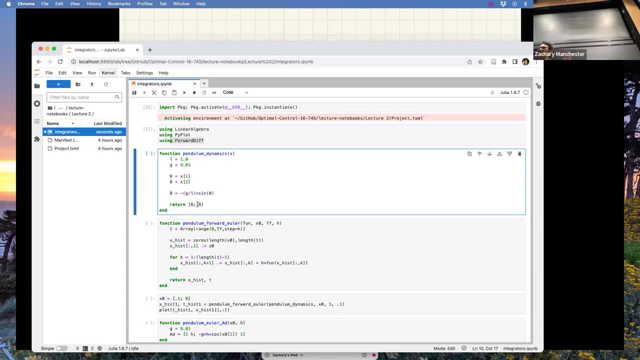 You write backslash theta, just like you would LaTeX and hit tab, and it does anything, Anything you want, which is pretty sweet. So you can write your code. It can look like your math, you can. So, yeah, like theta, dot is backslash theta, backslash dot tab. 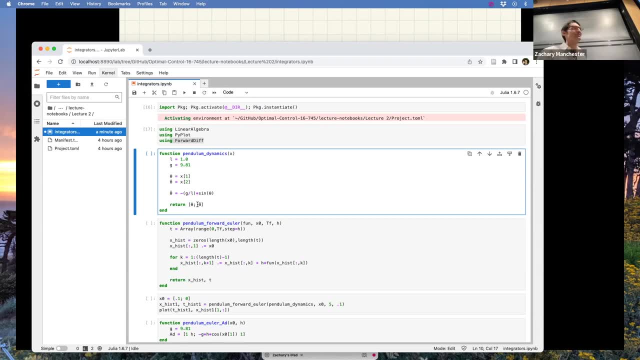 Yeah, renders the LaTeX, which is cool. You'll get the hang of it, It's not too hard, But otherwise, yeah, it basically looks like MATLAB, Like if you just write like. that's how I started getting into this. 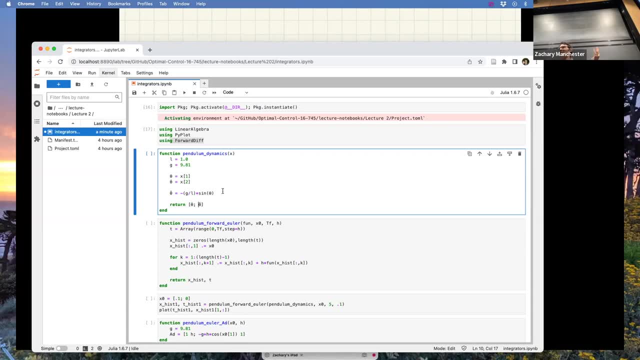 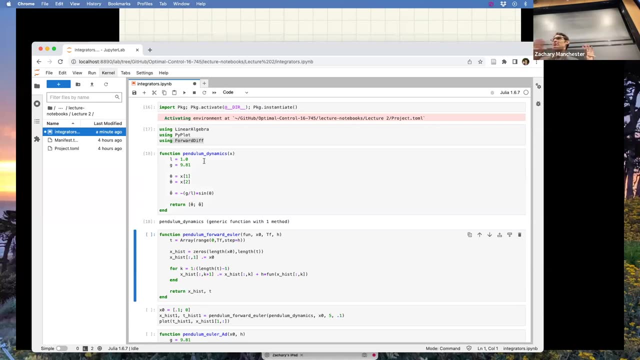 I literally copy pasted my MATLAB code and fixed the handful of errors. So if you know MATLAB, this is very, very easy. Okay, cool. So there's my dynamics again. This is my F, right F of X from last time. 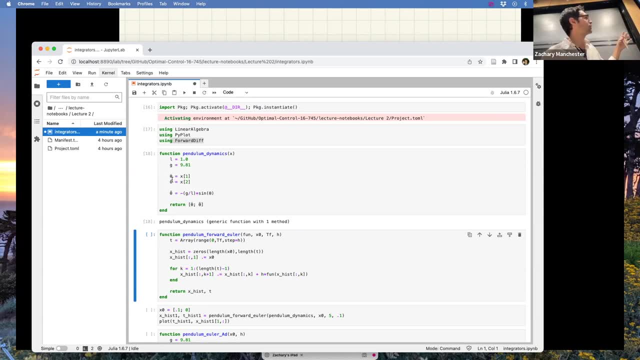 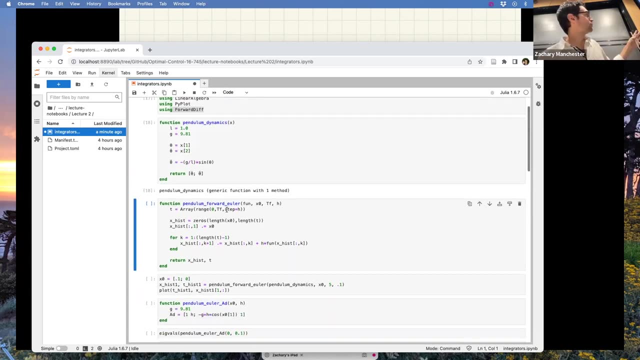 Continuous time: X here, X1.. I'm pulling out the theta and theta dot explicitly. I evaluate theta double dot And then x dot is theta dot, theta double dot, Cool, Okay, so here is the forward Euler integration that we just wrote down. 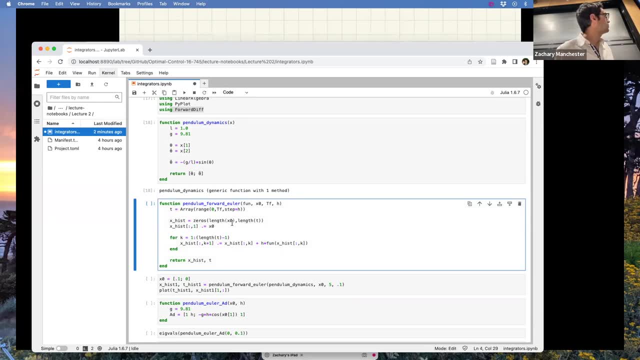 So I'm going to run this from: Okay, what's it doing? It's going through the loop here, right? And here's xk plus h. times f of xk is xk plus 1.. That's sort of what we've just talked about, right? 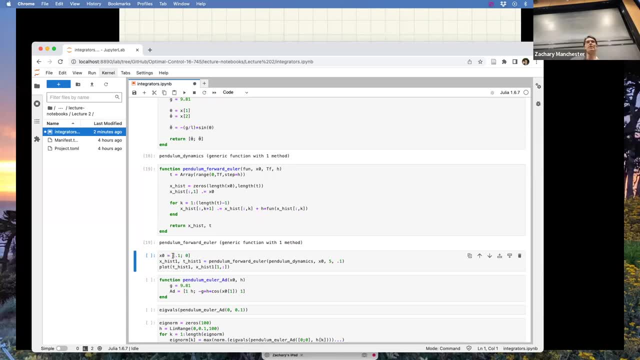 And now I'm going to go run this from an x knot that's like pretty close to the downward equilibrium right, 0.1 radian, So like a few degrees, you know, and I'm just going to let it swing passively under the dynamics and let's run it. 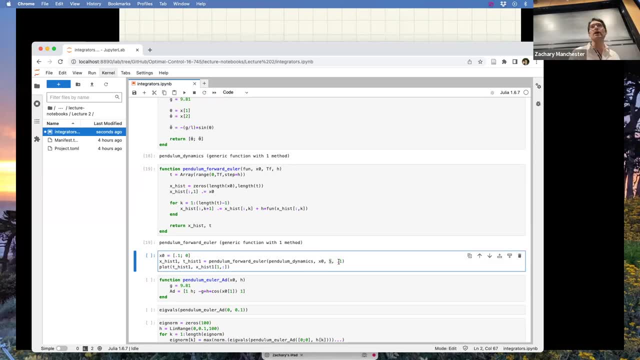 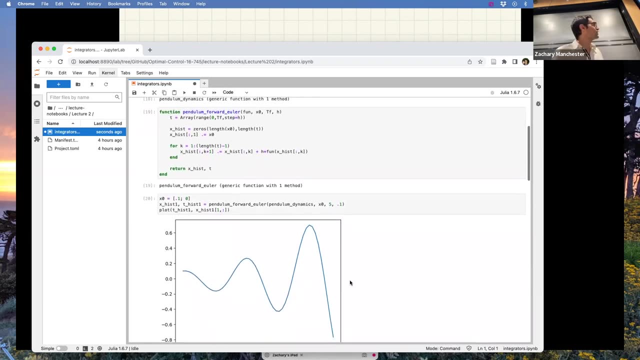 We're going to run it for five seconds with a time step of 0.1 seconds, like 10 hertz, And we're just going to see what happens, Okay, and then plot this: What's happening there? What should happen there? 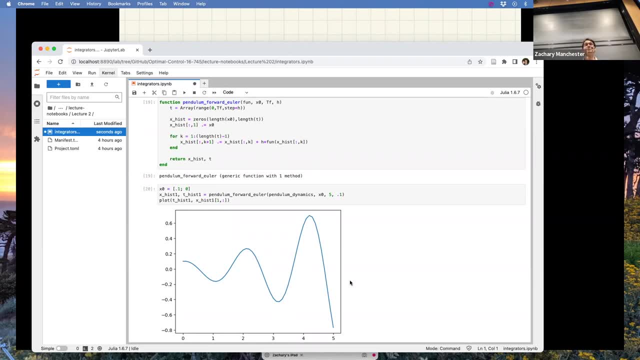 So there's no damping. So I wrote down, you know, just the original ODE, which should just intuitively- if there's no damping, there's no anything- It should just rock back and forth about that same initial angle forever right. 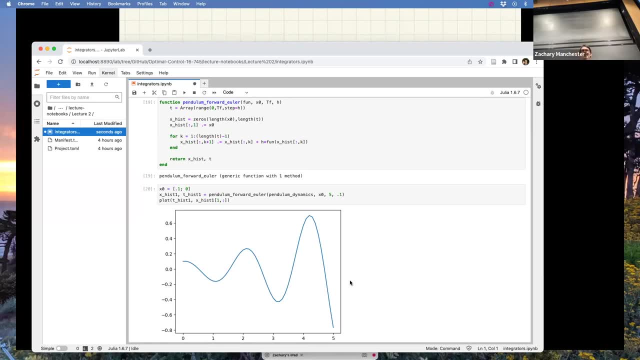 That's what it should do. What is it doing? It's getting bigger, right. It's blowing up. It's not damping, It's the opposite. right, You're getting energy increasing, right? I don't have any thoughts on what's going on here. 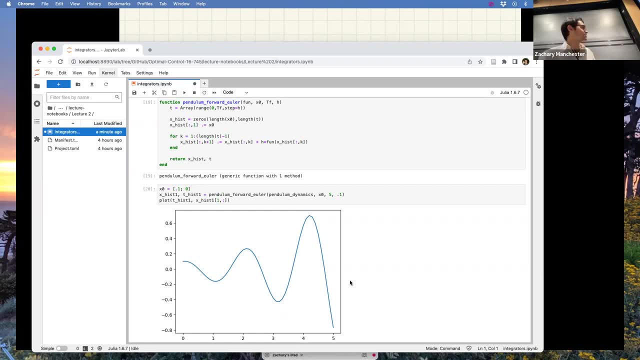 Yeah, that's a good Yeah. So this is very intuitive, right. So we're using some discretization, like it's definitely got some error associated with that approximation where we took a little step along. you know x dot, So maybe I need to make the time step bigger. 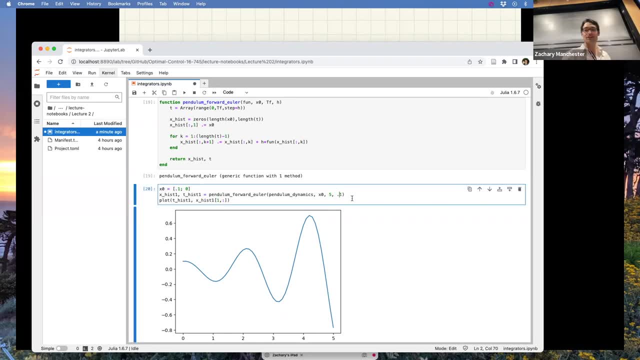 So let's try running it at 100 hertz instead of 10 hertz. That's a very like good idea. What happens there? It's a little better. Let's run this out for a longer amount of time though. 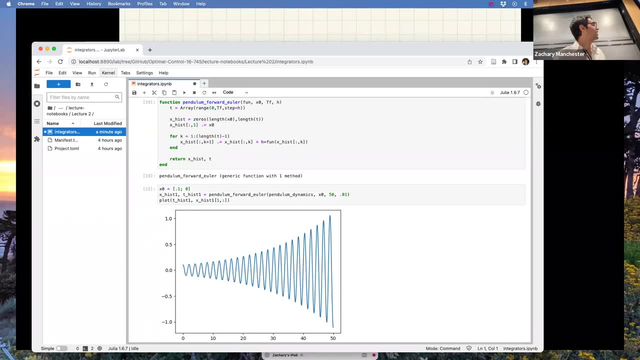 Let's run it for like 50 seconds instead of five. It still blows up. You don't have any other thoughts on this? Yeah Yeah, Error accumulation is like that's always going to happen, Absolutely. But there's something like a little extra weird going on here associated with this blow up, right? 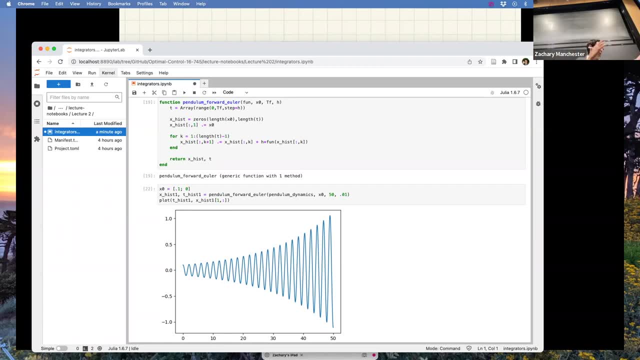 Because error accumulation, that could do anything right. And if the errors were random, you know you'd expect it to sort of average out to zero, right, Like if the errors were, say true, random, uniformly distributed, and you did this over time, you would get something, a random walk or, like you know, an average out in some sense. 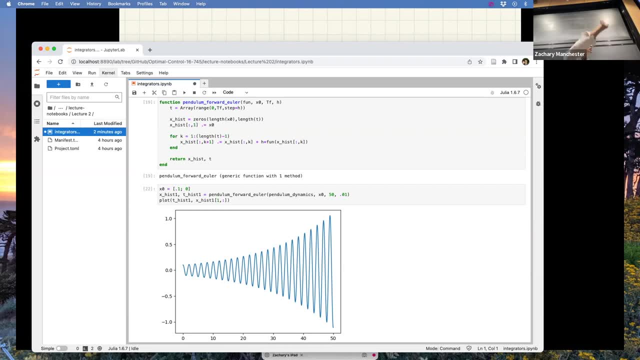 And that's not what happened. What's happening here? right, There's a very particular energy blow up behavior happening here that's associated with, like an instability, right, Yeah, What do you have? Well, it's so we're taking, you know, the tangent line to the slope. 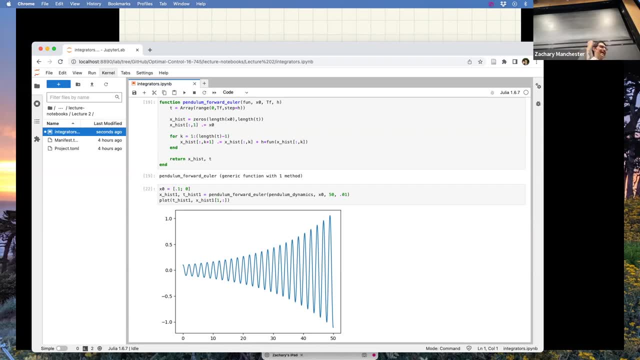 Yeah, always overshoot. That's exactly right. Excellent, Yeah, I was going to draw that little cartoon in a minute, but that's awesome. That's like the key insight, right? So there's a very, very peculiar interaction here between the natural dynamics of this system, which are oscillatory, and the fact that you're always taking a linear approximation of the 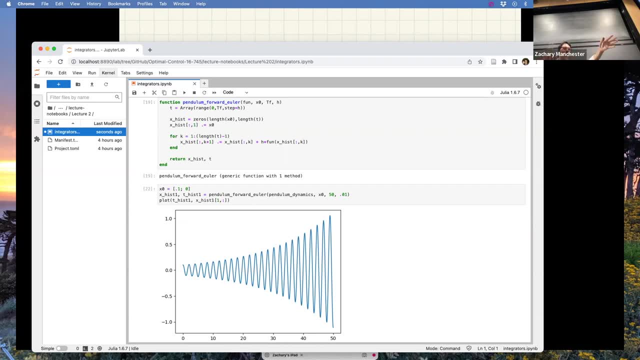 of the trajectory with this oiler integration. I'll draw the picture, Don't worry, You nailed it. Yeah, So you end up actually always overshooting right. So you can imagine my sign was going up and I take a linear approximation. 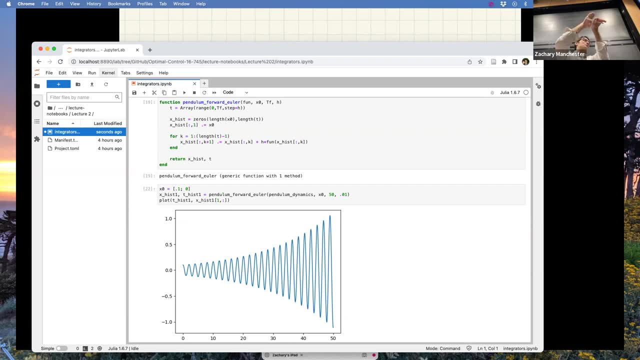 That linear approximation is going to always overshoot the sine curve, And so, as I keep going and doing this, I'm always overshooting at every dip of the sign right, Because the linear there's like a. you can write this down formally, but that's, that's the insight. 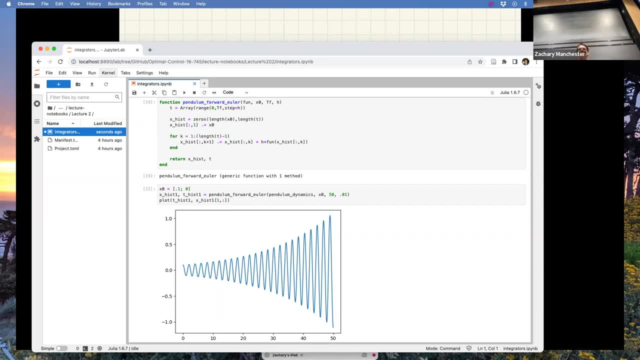 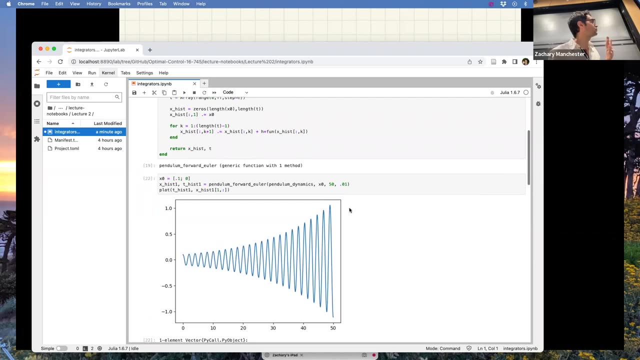 Yeah, Did anyone else have anything to add to this conversation? But yeah, awesome, There you go. Okay, cool, So let's go write down some math out and look at this. But yeah, so the key takeaway message is: it doesn't matter how small I make the time, step here. 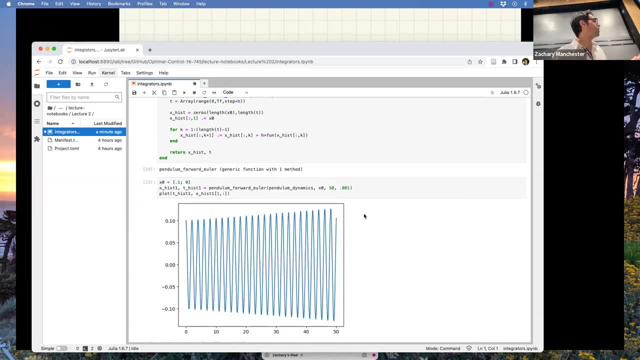 I can make it arbitrarily small. I can go to a thousand hertz, I can do whatever I want. Thousand hertz is still doing this right. All that happens is it basically delays the inevitable. It's going to push the blow up out farther in time. 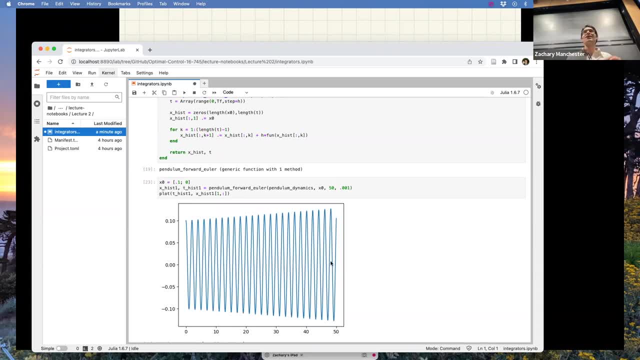 Yeah, Can't we remove the positive part of the eigenvalue? So yeah, there's something there. So what we're going to do now is go right down The eigenvalues of this thing And then think about that a little bit. 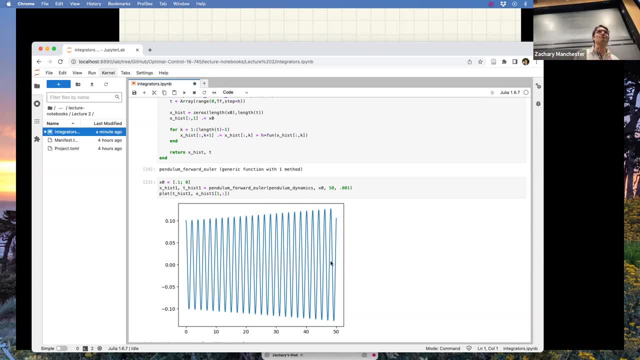 So not exactly, but we'll get to what you're, what's going on, in a little bit more detail. I'm like show you what to do. Any other questions about anyone with? try anything else here. You don't believe me, All right, cool. 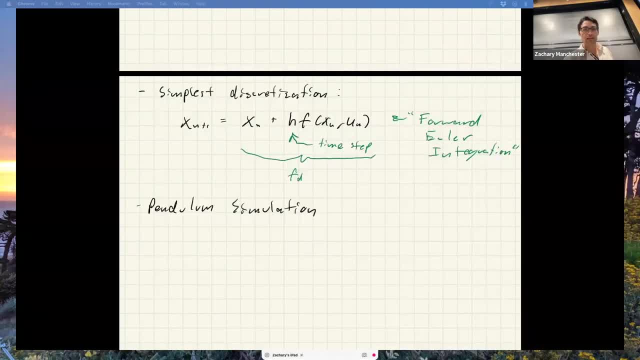 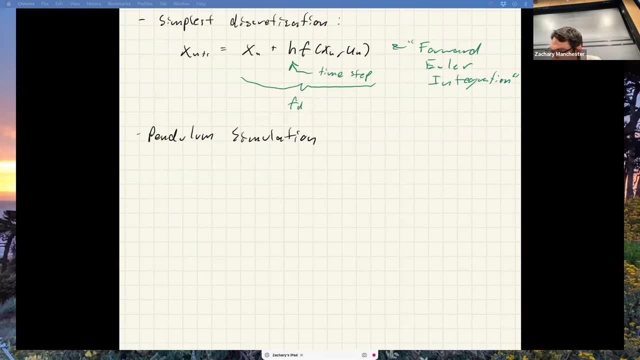 So we'll go back to the math for a minute. So what did we do? We did, you know, like L equals M equals one, We did H equals, you know, zero point one, zero point, zero one. You did kill a hertz, right. 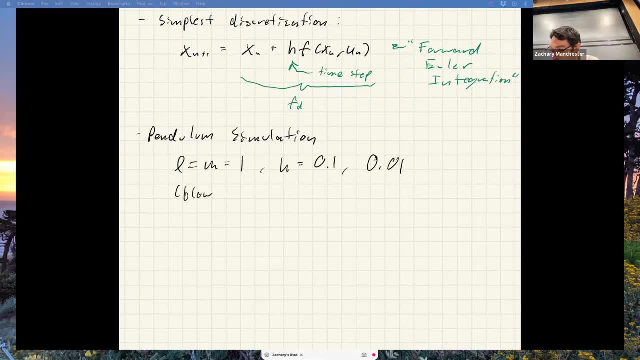 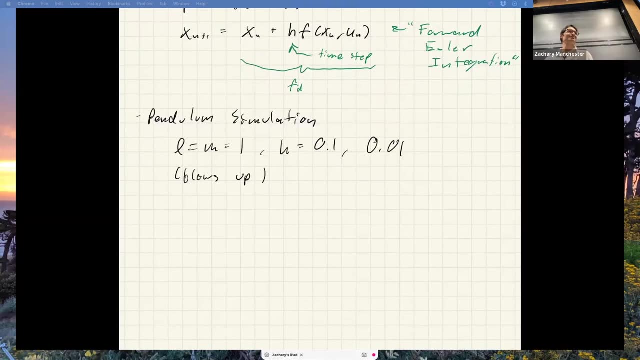 And it sort of always blows up, no matter what you do. And then we, kind of like you, actually nailed the intuitive answer to this, which no one has ever gotten before. So awesome, Have you seen this before, Or did you like just get that on this at some point? 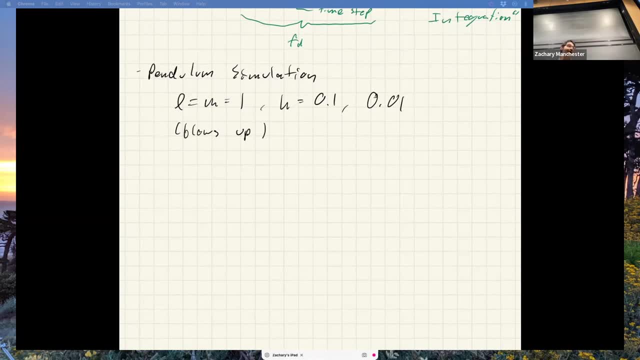 That's right. Programming for the simulator? Yeah, same thing. It's anything oscillatory. You'll get this actually For that exact reason. right, Like orbits? the same deal. It's a periodic orbit. Yeah, Okay, cool. 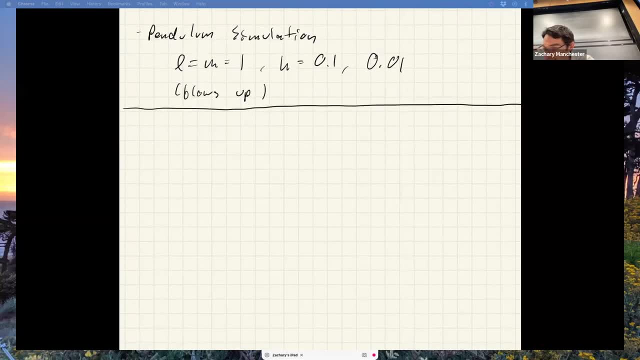 So let's talk about stability of discrete time systems. So remember- and I think that the overall message I'm trying to convey here is: be careful, because whatever your continuous is what the system does when you discretize it, weird things can happen. 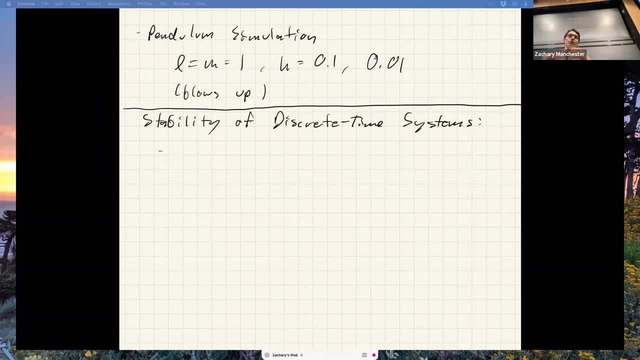 and the discretization can introduce like really gnarly systematic errors in the solutions that aren't physical, is the overall takeaway, But we'll get into some of the details. Okay, So from last time, in continuous time, we had this kind of eigenvalue result where we wanted the real parts of all the eigenvalues of the jigsaw. 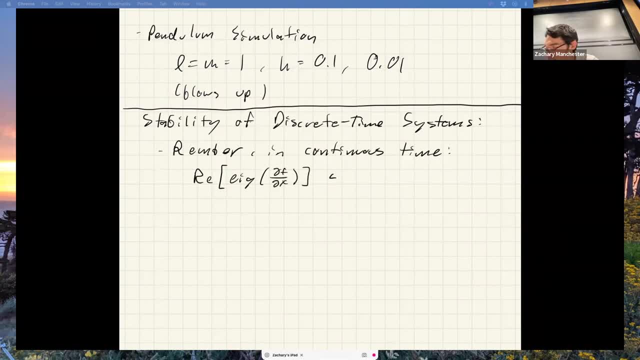 Jacobian matrix to have to be strictly negative to be stable, right, And we talked about this marginal stability case where it was exactly zero, which is actually the thing we've got here right- which implies sort of bounded oscillations. Okay, 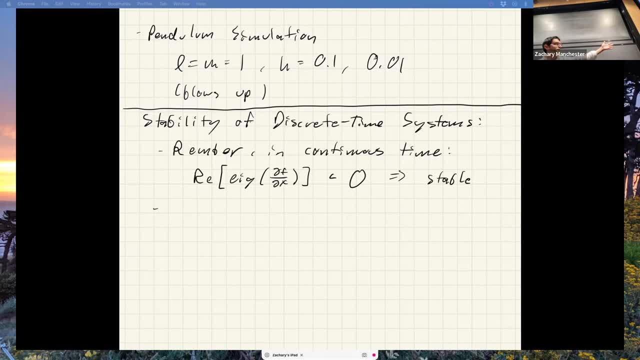 So let's think about what is happening in discrete time. So when I go simulate this thing in discrete time for a long time, right, If you think about what's actually happening there in terms of the dynamics, the discrete dynamics, it's really an iterated map. 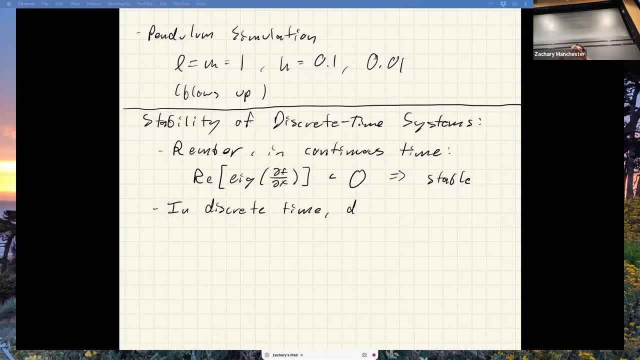 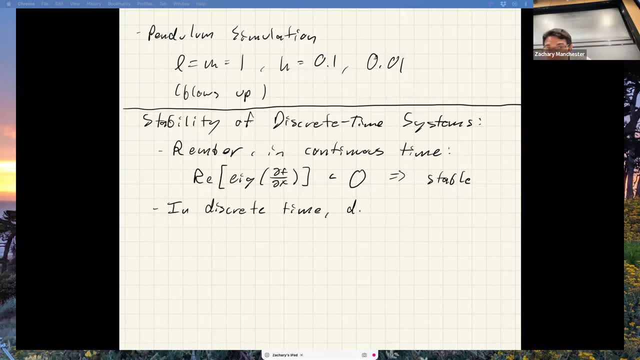 right, That's mapping me so many times steps in the future. So we got x, n is f of f of, f of blah, blah, blah, lots of Fs of like the initial conditions, right, Something like that. So if I think about that sort of 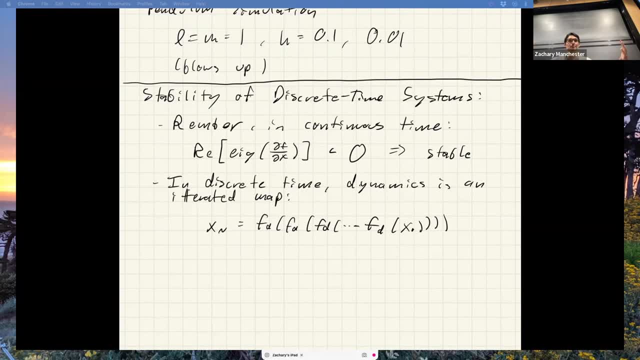 you know iterated map and I think about linearizing it. I get chain rule. I'm like back propping through that thing, right. So it's basically the Jacobian of FD times. you know, just iterated Through right. 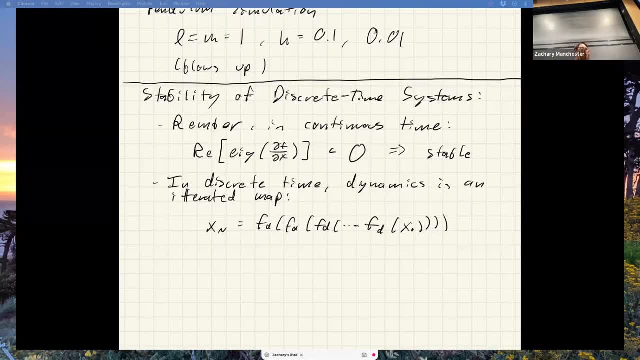 So if I take this, if I like linearize this about the initial condition x- not right about that initial point- then all the Jacobians are basically the same thing. If I'm doing it like at an equilibrium, So then it's just that one Jacobian just chained together. 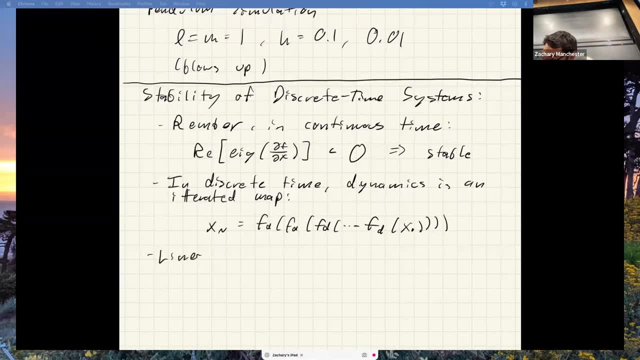 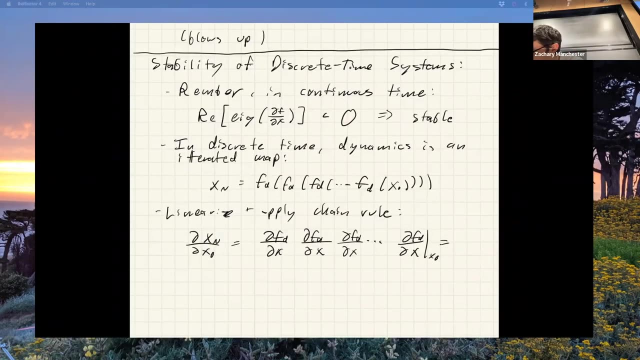 right, So we're going to do that. So partial x n, partial x not is really what we're after, right? So we're going to call the member. We called a, the partial f, partial x last time the dynamics Jacobian. 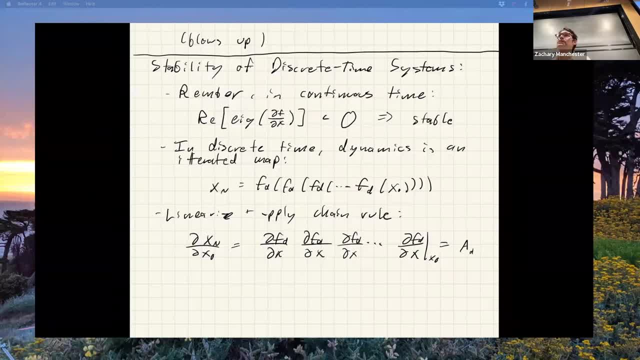 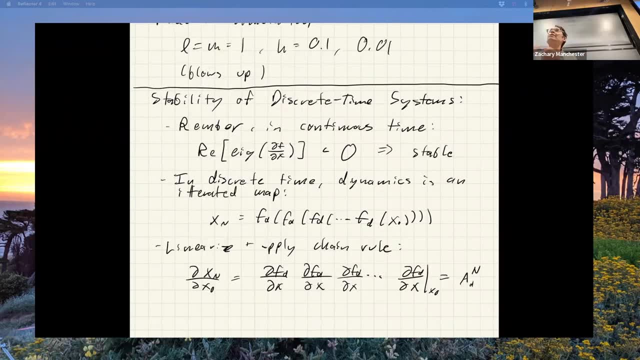 right. So this we're going to do for today: A sub D for discrete. So this is a sub D to the nth power, right? Just yep, So this okay. So if I want to simulate n steps of dynamics in discrete time, 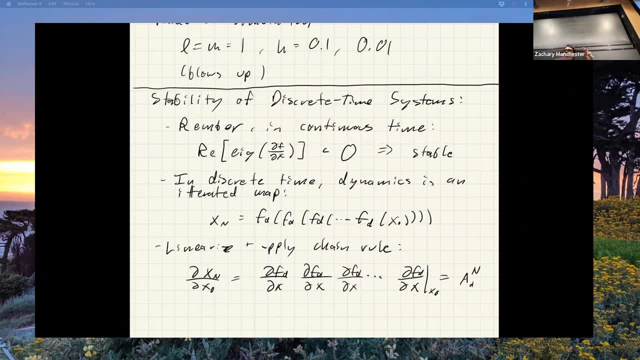 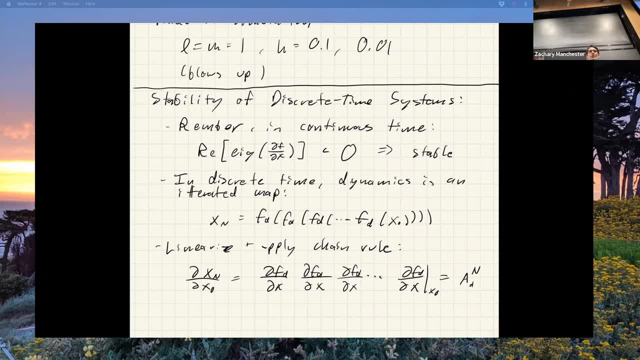 right N times for n times steps right. That makes sense. Cool. So then if I linearize through that, I just chain rule through all those function calls and then it ends up being: you know, chain rule, right. 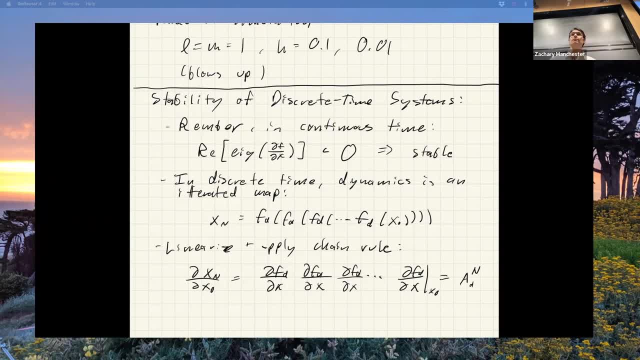 So this is like: just take Yeah. So what I'm going to do here is I'm going to linearize about an equilibrium point. So if x not is an equilibrium point, then it's just sitting there for all time, right At that equilibrium point. 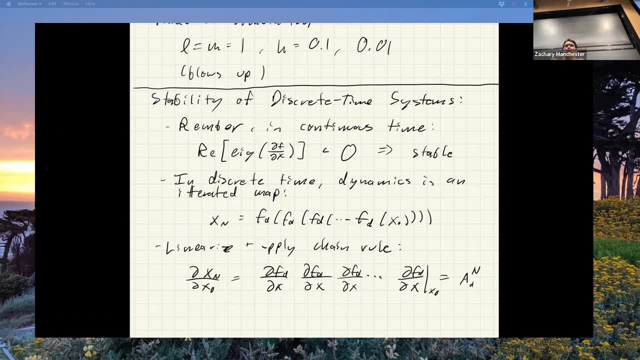 right. So it's a fixed point, stable, blah, blah, blah Like the think about so x not. here is like the pendulum hanging straight Down right. So if I call this n times, it's going to just sit there straight down because it's an equilibrium point. 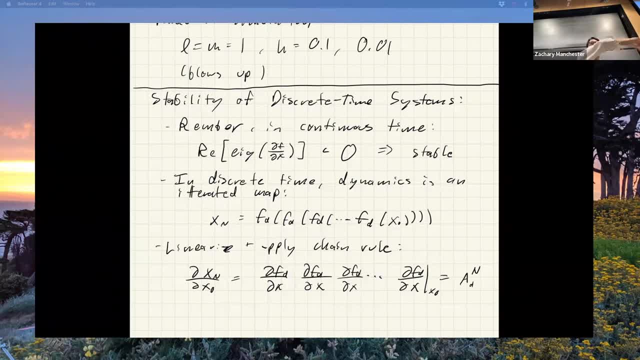 So then that x is the same for all of these n time steps. So then, therefore, the Jacobian is the same Jacobian for all in time steps. So then it's just 80, nth power, right? Does that make sense? 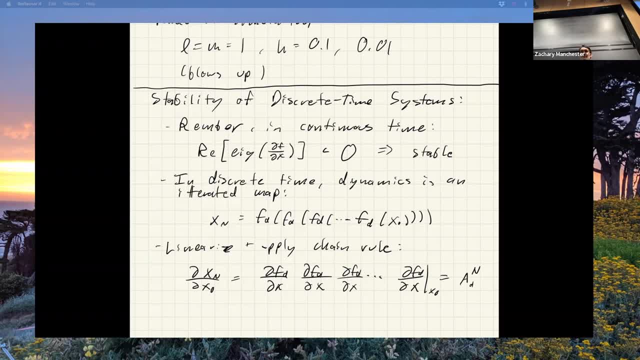 Is everyone clear on that? Any other questions about this? So this is this. you know, what I just wrote down is true always, but the where you, if it's not an equilibrium point, like I'm doing this about some trajectory or something where x is. 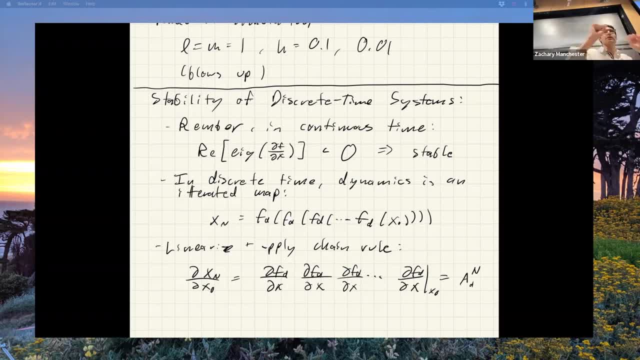 is changing it, then these Jacobians would each be evaluated at a different x, But the chain rule thing, you know, still applies. right, Okay, I'll get Yeah. So for right now we're talking about an equilibrium point. 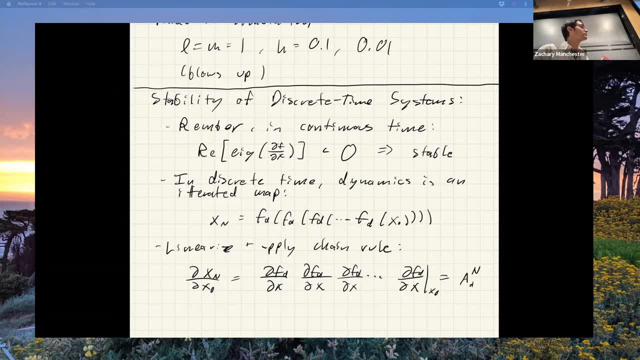 though The partial x partial is, shouldn't that perhaps be like partial x and partial x at x not? Yes, they're all evaluated at x, not in this case. No, I get that. I mean on the left hand side. 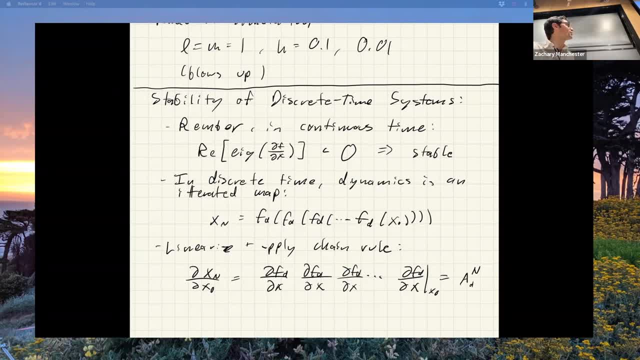 the left hand side? Yeah, I don't know. So what I'm trying to get out there is: I want partial of x, n with respect to x, not all the way on the right, I don't know. Yeah, I know the notation is a little weird. 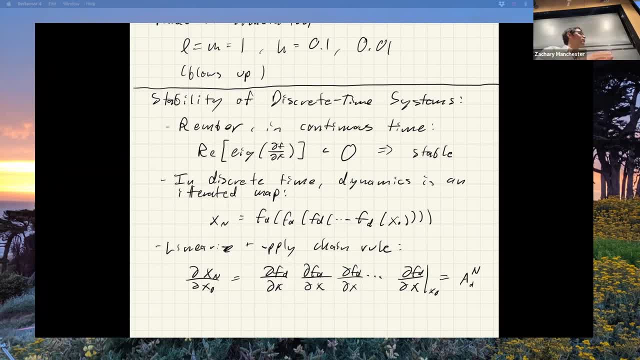 I'm open to suggestions, but is the idea clear, Like I'm really trying to take partial of the output of this with respect to the initial input on all the way on the right hand side. Yes, So this is the partial of the final state after n time steps with respect to the initial state at time zero. 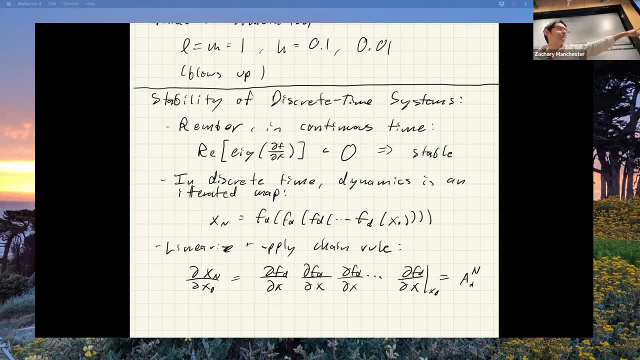 right, That's what that derivative is, And if I just go do that through that you know function composition- I just get chain rolled And because it's an equilibrium point, it's sitting there for all the time steps. So all the Jacobians are evaluated at the same x. 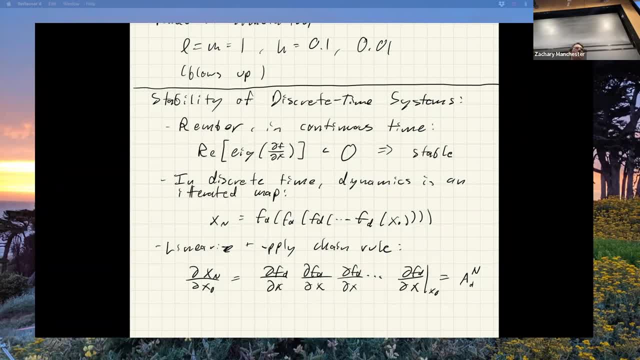 So that's just a to the end, right? Yeah, I mean it's well sorry. can you repeat that? Oh yeah, as you go across. Yes, but the point is here because it's an equal. So, in general, 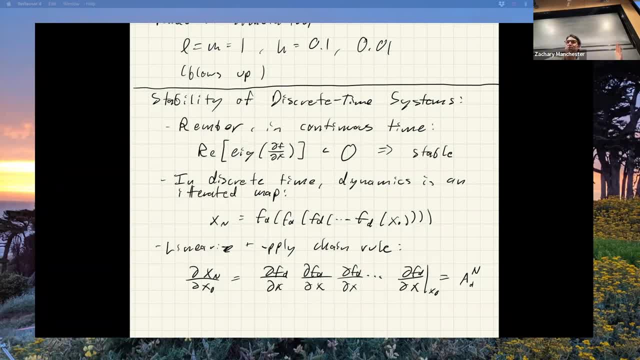 you're absolutely right, Like if this was moving around and it was a trajectory that I was linearizing about 100%. in this particular case, those x k's are the same for all k because it's an equilibrium point And so it's just going to sit there. 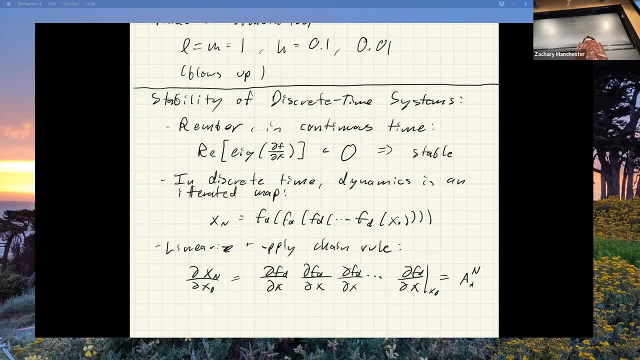 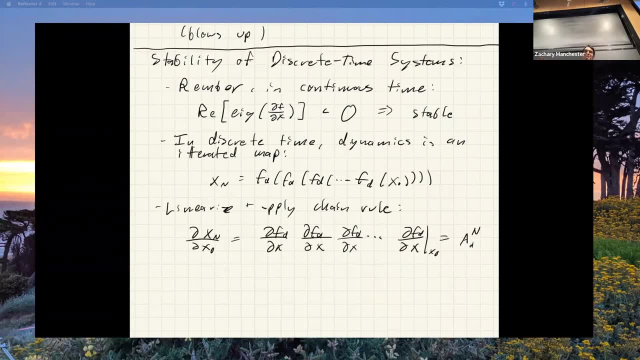 right, That makes sense. Yeah Yeah, I'm sorry if this is not clear. I got it. We got a little screwed up there, So hopefully this is clear. Definitely stop me and interrupt me if this isn't making sense to you. 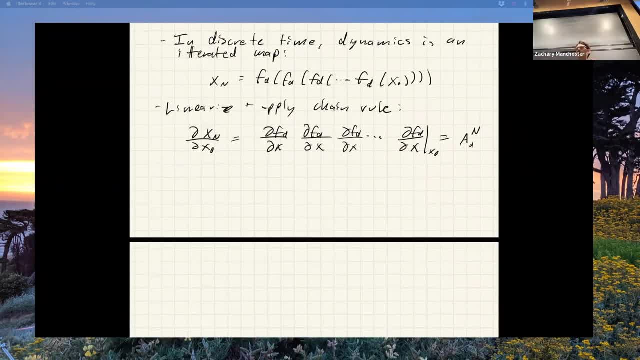 Okay, cool. So so is this clear to everybody now that what we're doing Awesome, Okay. so now we're going to make the assumption here, which is kind of trivial and not important actually that, but just for now, to make life easy. 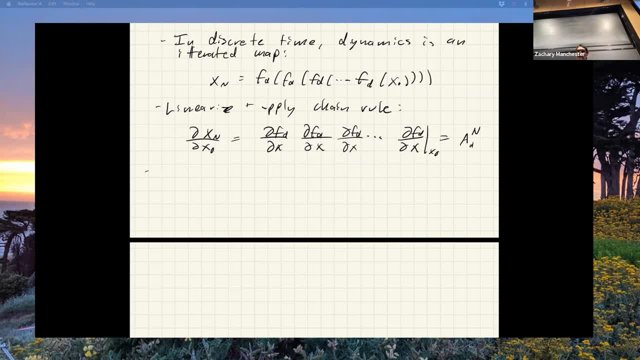 we're going to assume that we've set our coordinates up, So the equilibrium point is at: x equals 0 at the origin. It's trivial to shift this over by constant, So like we usually assume this. So in you know, x not equals 0, basically, at the origin. 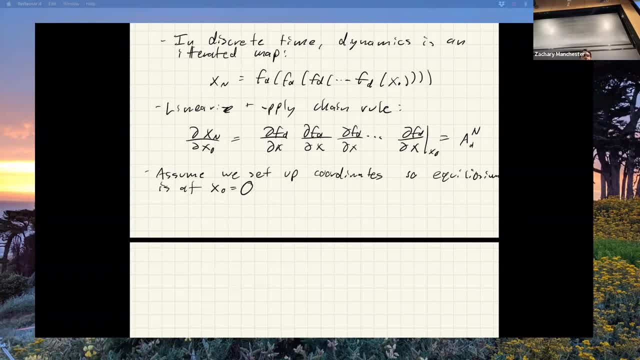 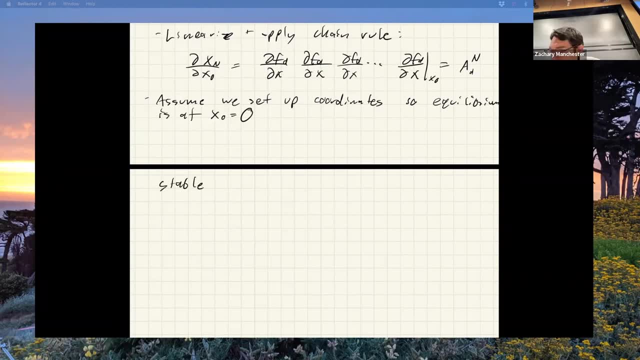 And so this is the case in the pendulum, in particular, right Theta equals 0. is this downward equilibrium? So we are in this situation already, And so, if we think about what it means to be stable, here we're talking about right in this case. 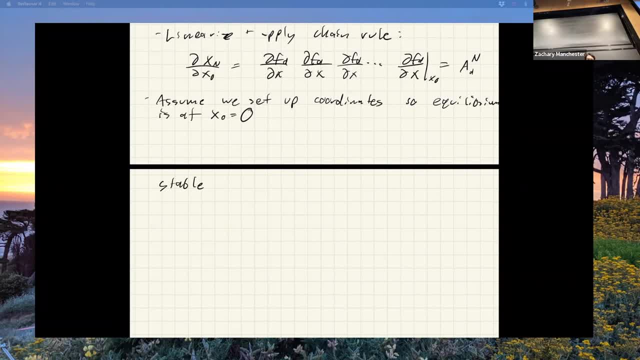 stability means, if I perturb this thing a little bit from x, not It, you know, as I take the number of time steps to infinity right As I run this simulation forward, for like many, many time steps, it should converge back to x. 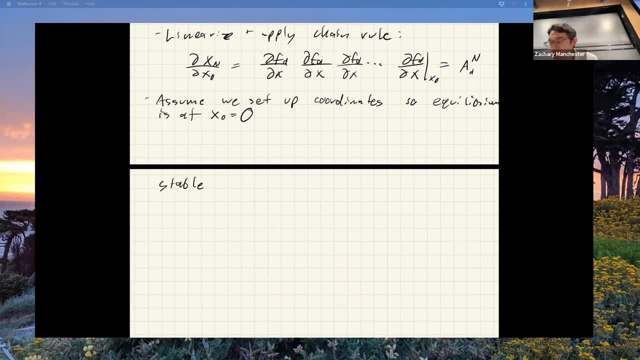 not, right? That makes sense to everybody. So if I think about the linearization, then what that's going to mean is any x not has to convert back to 0, right? So that's true for any x not. So let's write that down. 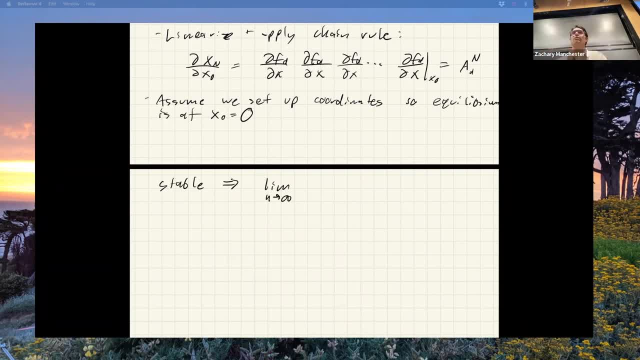 So I'm saying limit as k goes to infinity. I'm using the linearize that dynamics. It means a, this discrete time, a to the kth power times, x not has to equal 0 for all x, not right, Okay. 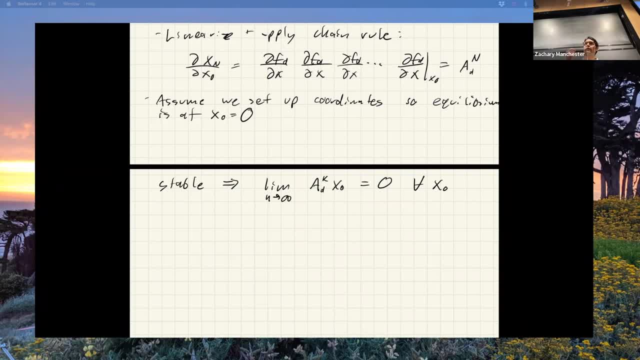 So if that has to be true for all x not. what can I say then about the a matrices? Yeah Yeah, Inside, strictly inside right Modules. So another way of saying this, though, a sort of dumber way of saying this: 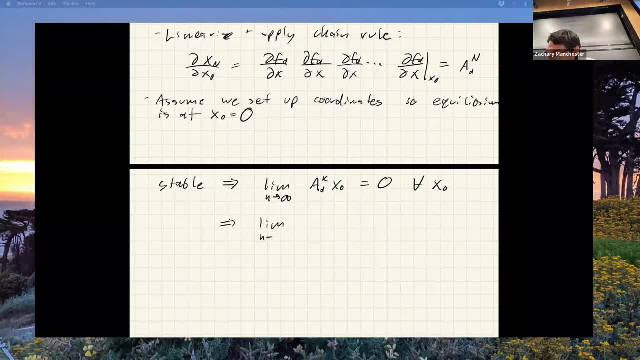 you know, for me is like a limit, as k goes to infinity of just the. a matrix right Has to equal 0. If it's got to be true for all x's, then it has to be true for the matrix That's multiplying x trivially. 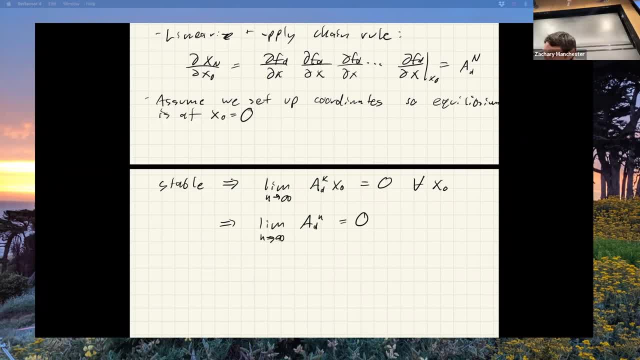 right. Okay, So for that to be true, then, like you, you nailed it right. Then, if this is always true, this says that the complex, complex modulus, or, like norm, right Of the eye, all the eigenvalues of this matrix have to be strictly less than one or inside. 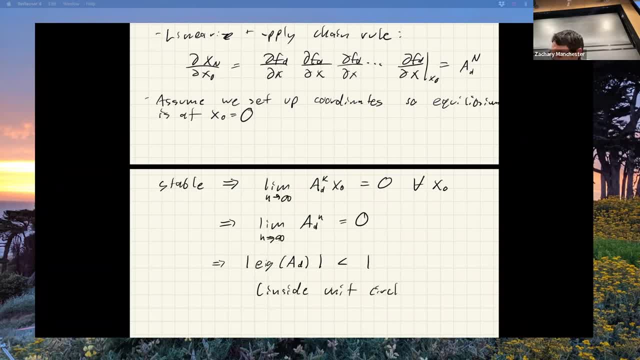 the unit circle in the complex plane. That makes sense. So yeah, intuition is just like. as I take that iteration out to infinity, I'm just multiplying those a matrices together, If that like has to go to 0 for any x. 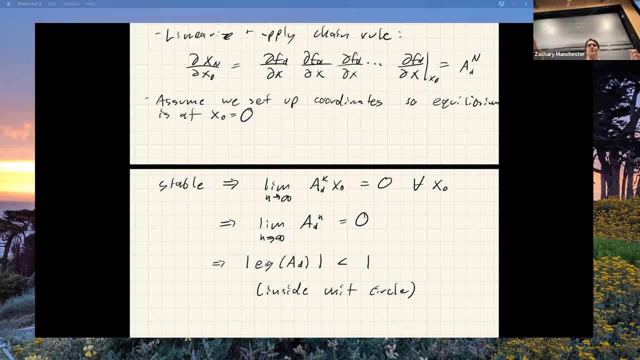 not has to go to 0 for the matrix, and the way that- another way of saying that, like a to the n, goes to 0 for large n, is that the eigenvalues? Yeah, yeah. So what ends up happening? if it's not the origin, is you. 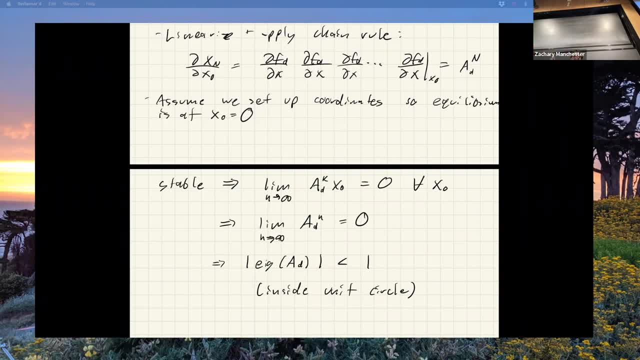 just get a constant in there, offsetting it, And so there the matrix condition actually is exactly the same. So what would end up being is like a to the x plus constant c, offset, you know, and so like the constant drops out when you like, do this. 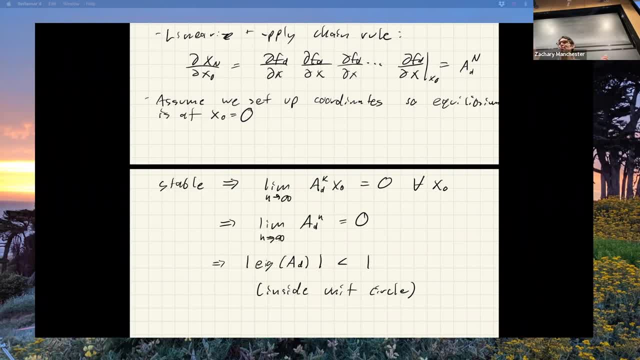 So it's still the condition on the matrix side And that is the same. Basically, we're here, We're just dropping this constant offset. That doesn't matter, It's kind of making it the origin Cool, Everybody cool with that. 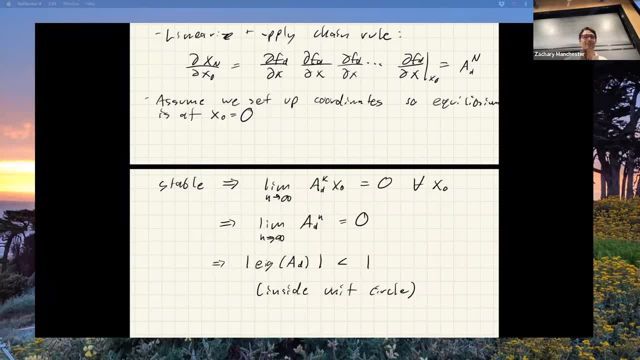 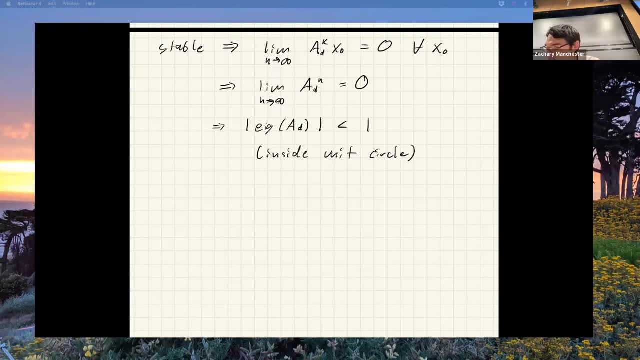 Any questions or thoughts on this? Okay, So now we're going to do is do this calculation for the pendulum with forward Euler. Okay, so, to be super explicit about this, here's what this looks like. right, X K plus 1 equals X K plus H times F of X K. 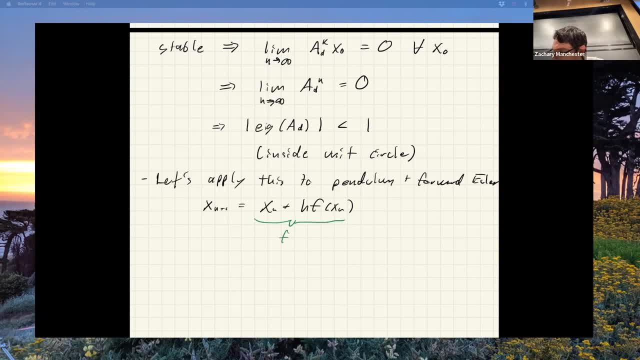 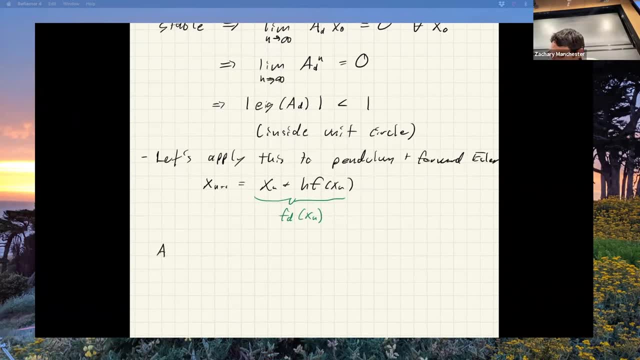 And this whole thing is our F D of X K. So now we're going to compute the Jacobian matrix. So this ad thing is partial of this F D with respect to X K. So I'm going to go ahead and just like linearize that thing. 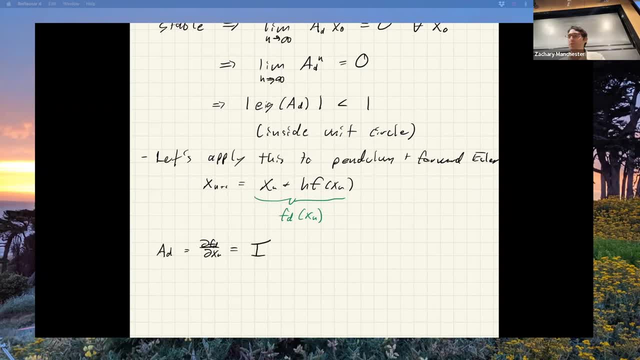 right, So that X, K is going to turn into an identity: partial X, partial X, right, And then the other part is going to be H times the original Jacobian. you know the original, a Jacobian right. The continuous dynamics. 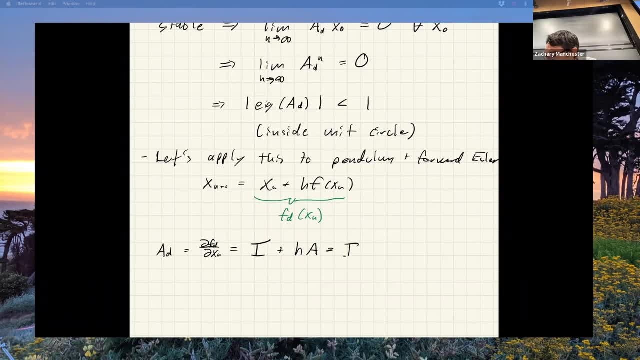 So if I kind of keep writing this out, expand it out a little bit, I'm gonna get I plus H times. We wrote this thing, I think, yesterday, which is easy to do: Q over L, cos theta zero should write this a little bit. 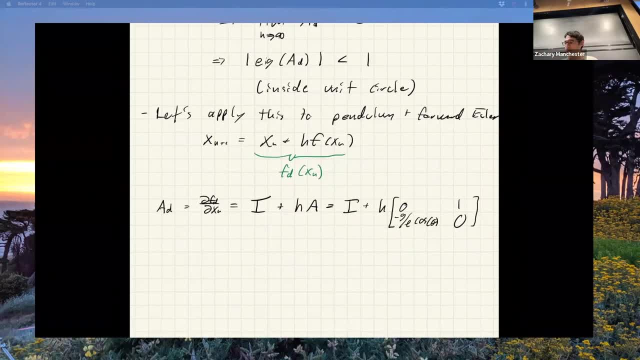 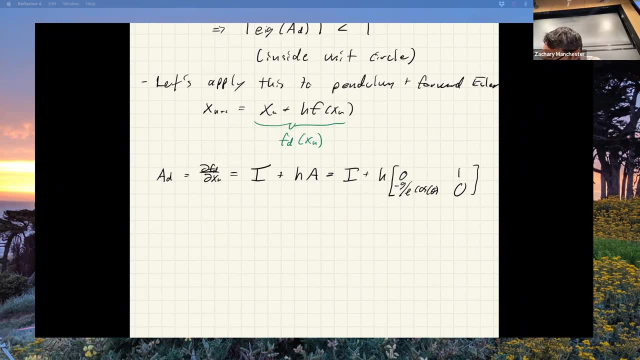 Cool, I'm cool with that. So I'm not going to sit here and like compute eigenvalues of this thing. We're going to use the computer to do it, I'll just write down. So if I, if I take the eigenvalues of this thing, 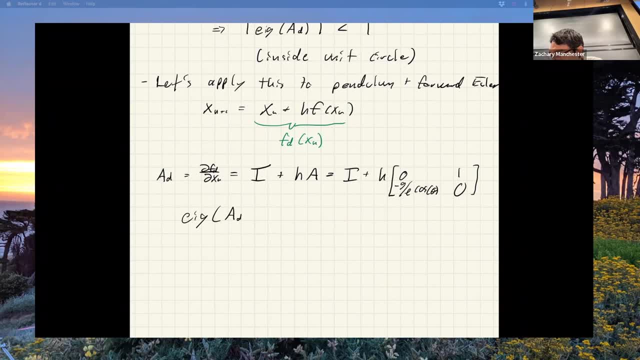 using the numbers we just used in this simulation. so we're going to linearize this about. we're going to plug in theta equals zero, So that coast is going to be a one, And we're going to use H equals point one. 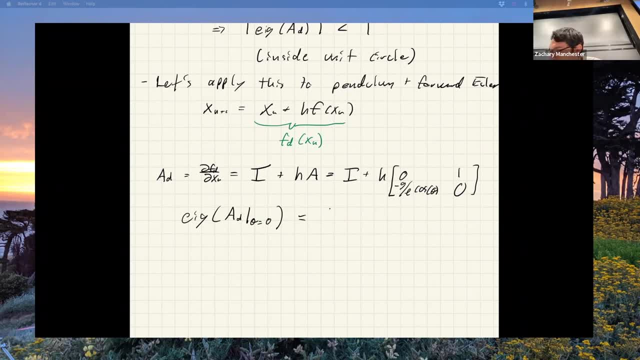 Say, you know the first thing we did. these eigenvalues are going to be one plus or minus zero point three, one three I, approximately. So what's the takeaway from this exercise then? This is most definitely unstable, right? So let's go. 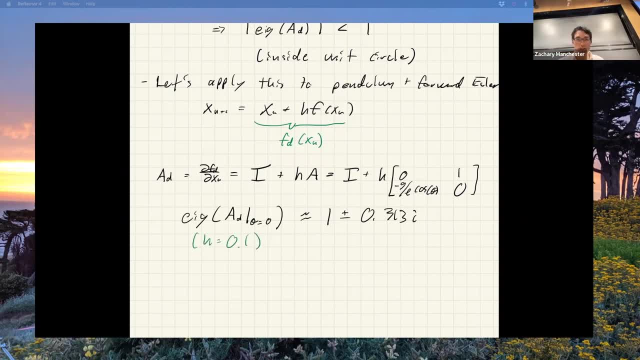 H equals zero point one. Okay, let's go look at this. So now we're gonna do some fun. We're going to go back to the The Jupiter notebook And pray that my computer doesn't barf again. Okay, so let's see. 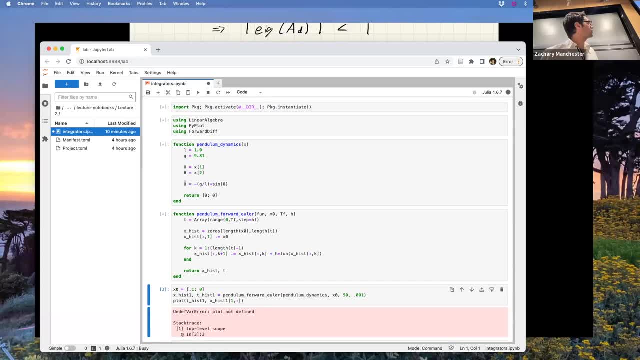 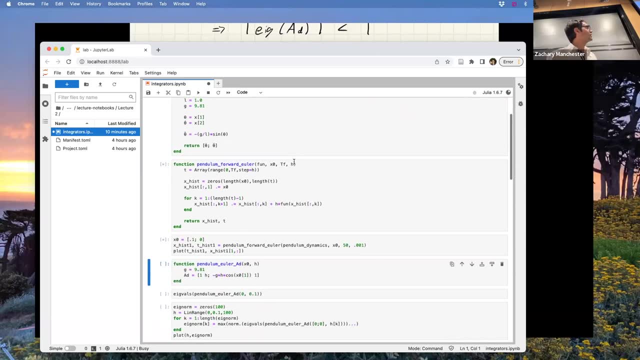 And I don't have to run a bunch of stuff again. So that crashed. Hopefully it still Works. It's going to think for a minute. I should have done this before while I was writing. Cool, Okay, so we're back to this. 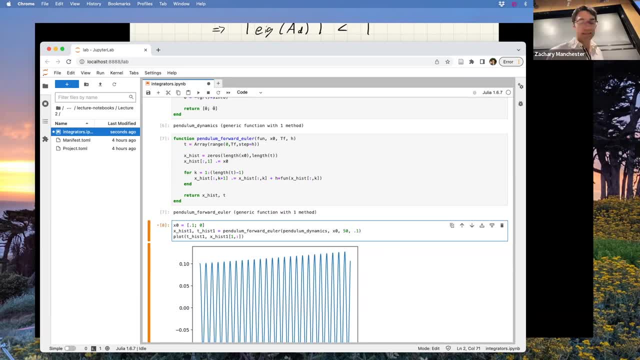 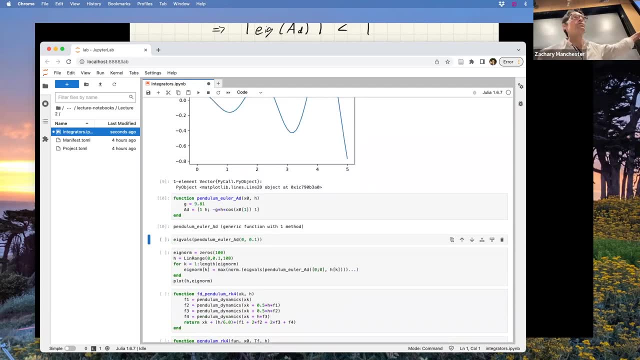 Let's, let's go put it back to like the 10 Hertz version, Just to check my math Five seconds, Otherwise it just looks stupid, Cool, Cool, Okay. so here's my discrete time, Jacobian, that I just wrote down. 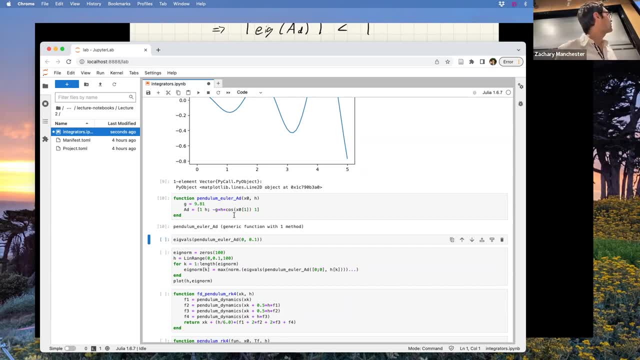 Everyone agree that I did that right. You're doing super down, Think I did that right, Cool. And then I'm just going to take the eigenvalues of that thing Evaluated at time. step is zero, point one and at. 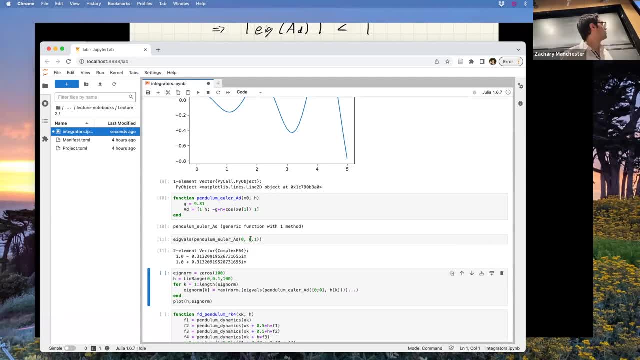 you know, fate equals zero, right? So that's what we wrote down. So, um and yeah, what else we do? We'd like you know hundred, Hertz, We can check it. you know, the thing gets closer and closer. 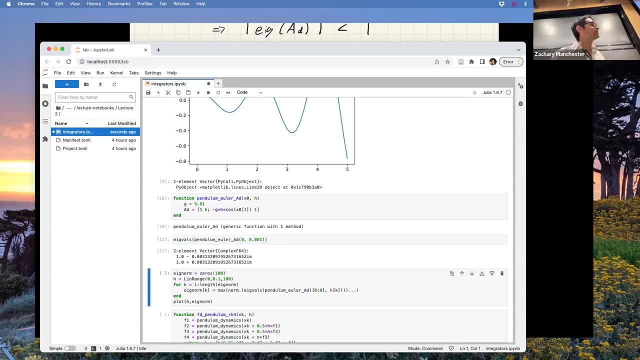 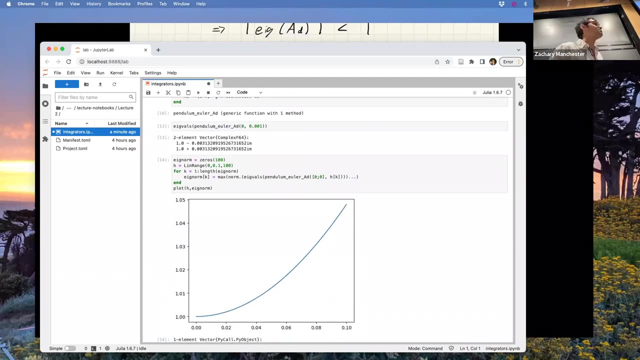 right, Thousand Hertz, But it's still always bigger than one. So let's plot this. So what I'm gonna do right now is plot these eigenvalues, Their modules, as a function of H. Why very age? And what ends up happening here is that it asymptotically approaches modulus one as H goes to infinity. 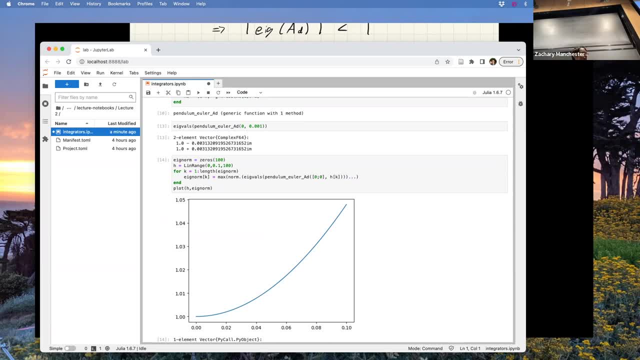 But it never actually gets there. So the message here is that if I'm using Ford Euler to simulate a pendulum, which is like a trivially simple system that we all kind of are familiar with, it will always blow up, No matter what you do. 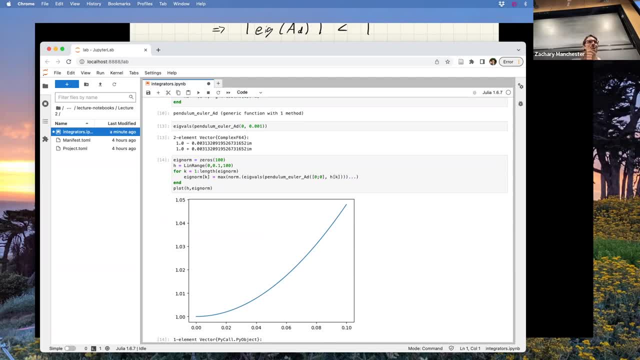 no matter what finite time step you take, it will always blow up. There is no. no, it is beyond redemption. Anyone have any thoughts about this? questions Want to try anything else, So takeaway of the day: don't use Ford Euler. 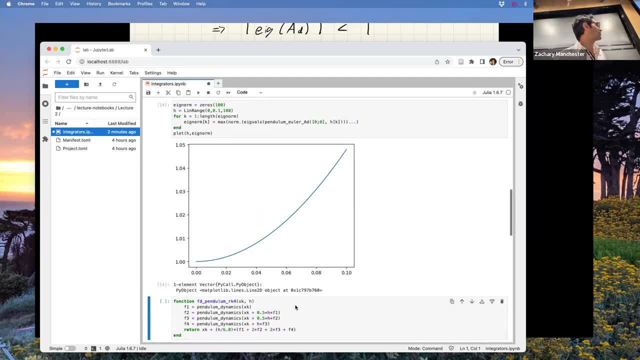 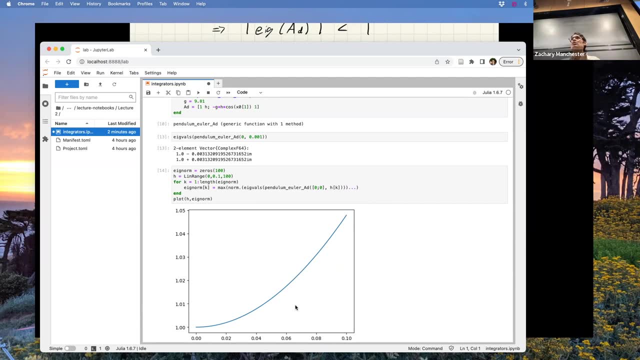 It is bad for you. It's a bad thing. What else? Okay, yeah, cool, Any questions? Yeah, So this is basically doing that. Well, so the linearization is making that small angle approximation thing right, But yeah. 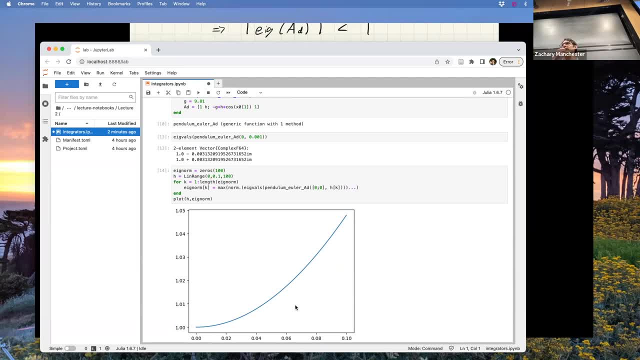 this particular blow up thing. this is kind of like an energy thing, right, There's like energy being added to the system and it's a particular quirk of the Ford Euler integration. And, yeah, let's go draw that picture. But you told us about 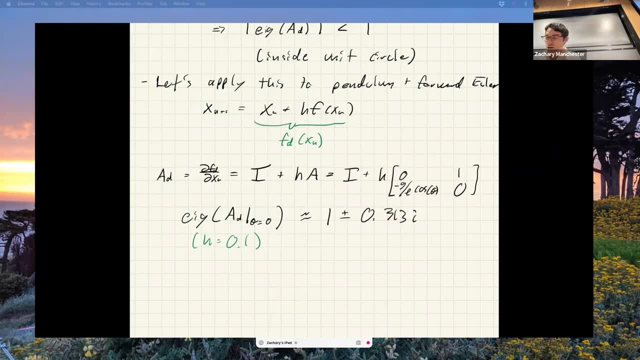 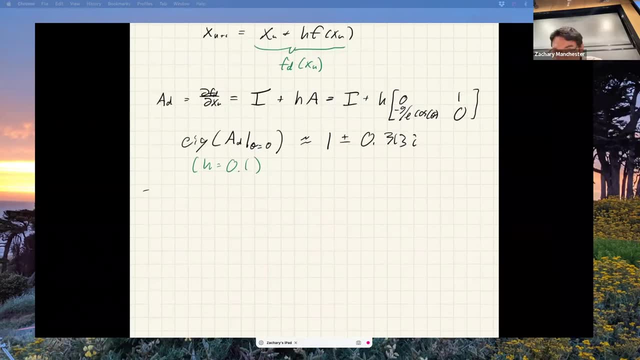 So where did I? Yeah, let's do this. It's still working, Hooray. So what did we just do? We did this thing He did versus H And yeah, basically only like asymptotically approaches being stable. 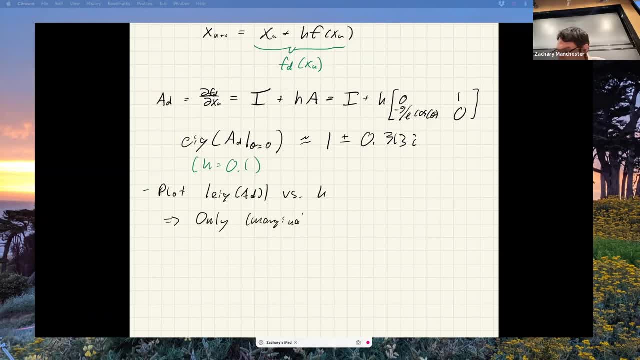 So that's not great, And let's see the. the intuition here from, like a physical perspective is, if I kind of think about what's going on, the solutions to this are wiggly sine curves And when I do the like, the Euler approximation. 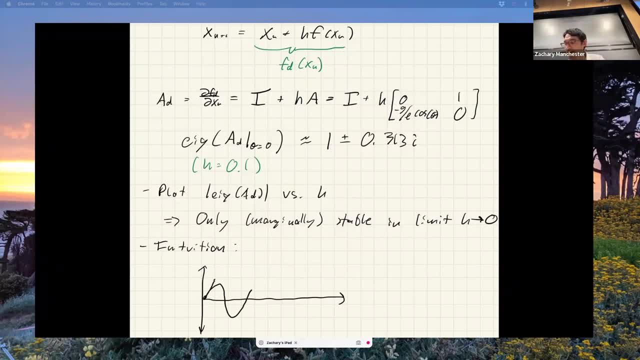 I'm taking like a tangent to this guy going up here and then like doing it again, right. So like I'm basically always kind of doomed to overshoot this guy. when it switches direction, Okay, cool. Well, that's not a great vaccine picture. 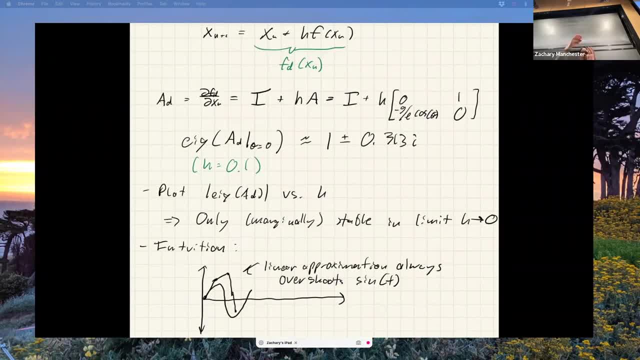 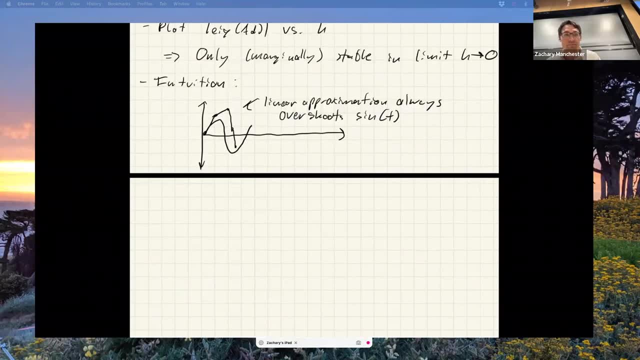 but does that make sense? Everybody like: basically, the sine curves down the lines going to always overshoot, and it's going to do it again when the sine curves up at the other side. Okay, so take away. message of the day. Let's see. 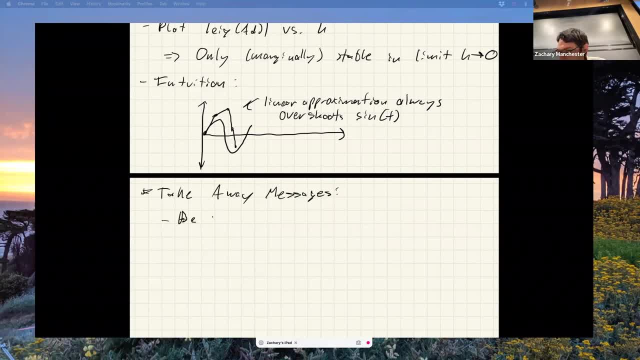 Always be careful when discretizing ODEs. Don't trust anybody. Don't trust your simulator, You know. don't trust me. Sanity check. So what? Yeah, what do you guys think Like, if you, if I, you know? 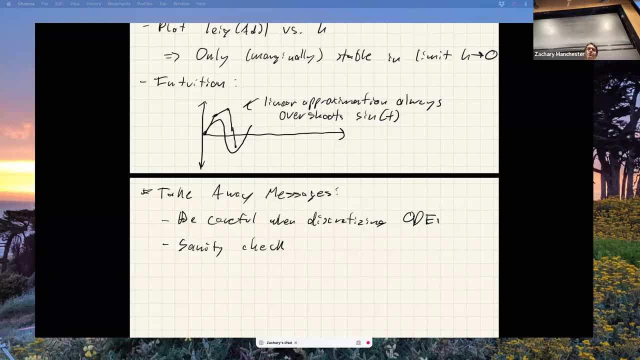 hand you a simulator like what are good things to send and check this kind of stuff to, like you know, can you Perfect? Yeah, What would you do? Yeah, Yeah, it's a classic one That's very good. 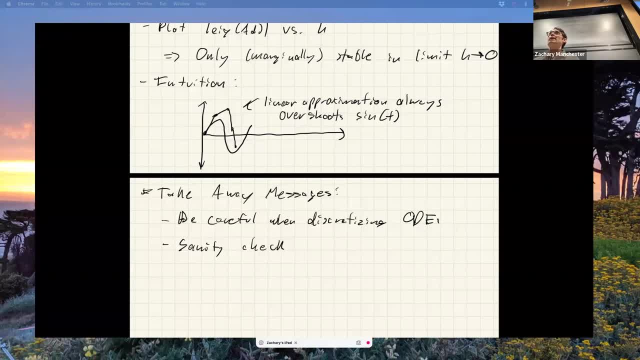 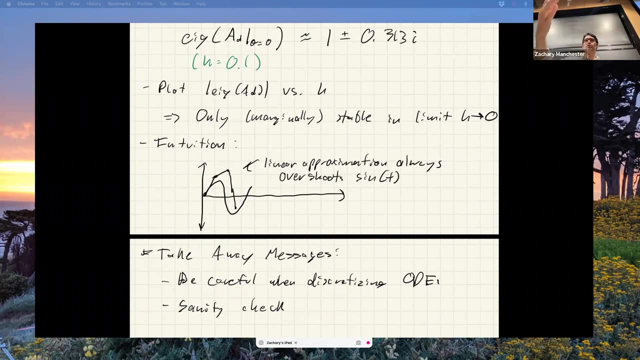 Anybody else have thoughts? Yeah, Oh, sorry. No, I'm saying that here. this thing only approaches marginal stability, like modulus one in the limit, as the time step goes to zero. That was that plot. Let's put this back up. 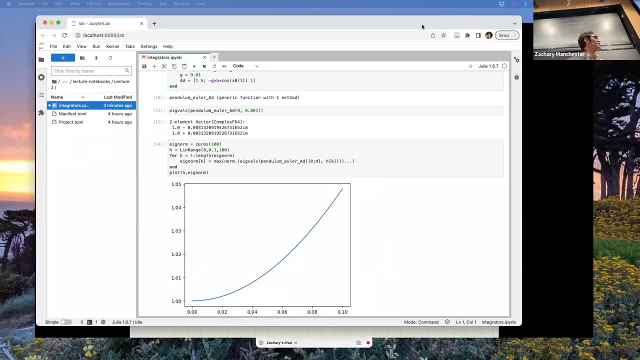 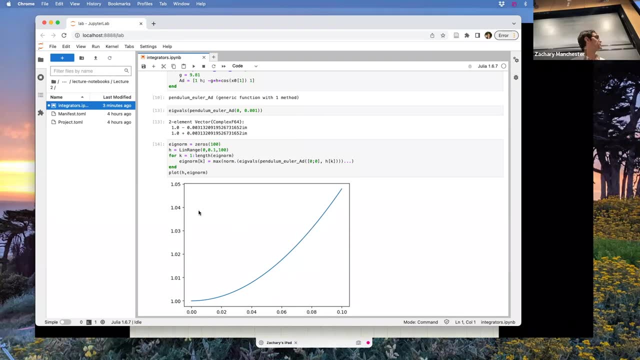 This plot right. So this is the modulus of the eigenvalues plotted versus H. So this is H on the bottom time step And then this is that that eigenvalue right And maybe marginal stability is H equals one or not H. 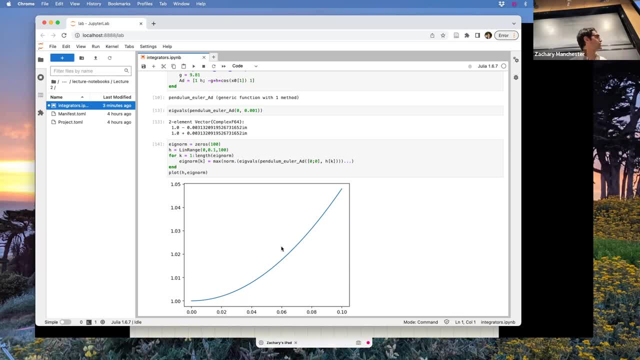 Sorry, eigenvalue is one right which is over here. So what's happening is this: this thing's approaching that marginal stable, you know, eigenvalue modulus one in the limit as H goes to zero. So that's what I'm saying. 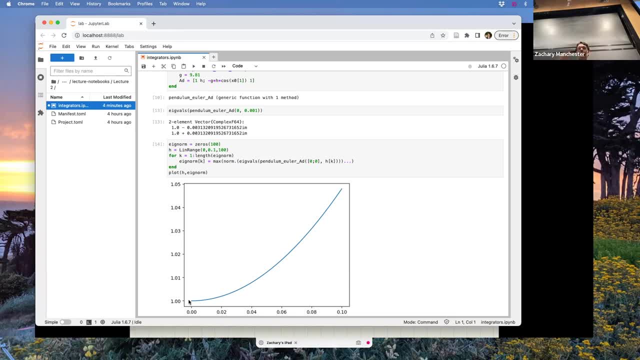 That makes sense. So, yeah, you're right. Yeah, you want the eigenvalue to go to one here. You want it to be one, right? For that means it's oscillating, And I'm saying it only gets there in the limit of H, goes to zero. 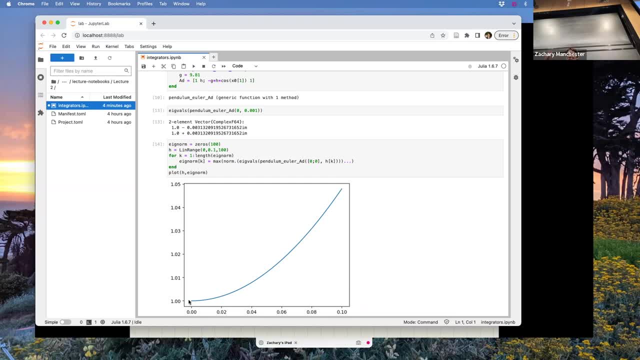 So with Euler integration, for any finite H bigger than zero- which is what you need to simulate it- it's going to blow up, no matter what. It's just a matter of how many times steps before it blows up. Yeah, cool, Is that everybody else? 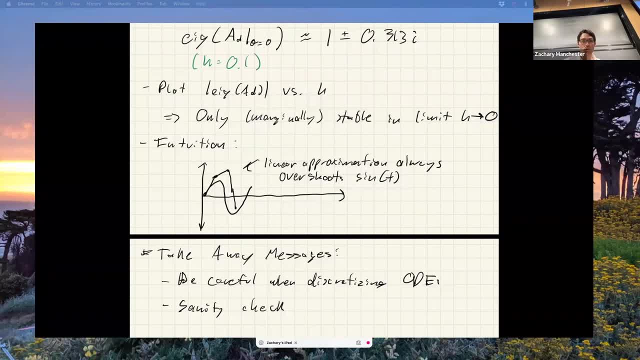 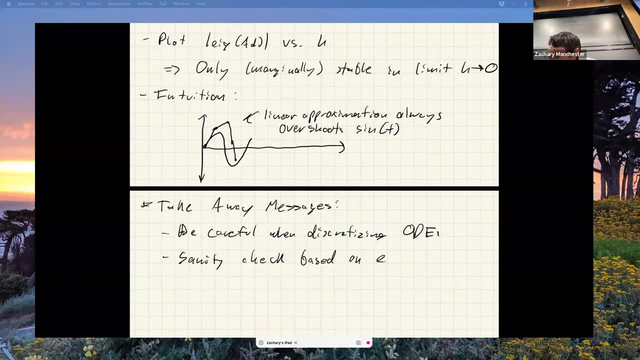 Okay, so sanity checking, Good things to do, Yeah, So yeah, check energy. Another one would be like momentum, right. So basically, like you know, if you check energy, right, if it's a conservative system, that should stay pretty much constant. 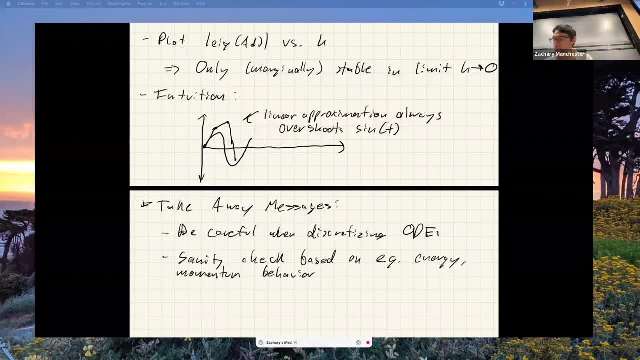 If it's got, you know, if it's a damp system, that should decrease, et cetera. right, Basically, you know, try looking at these kind of quantities and like qualitatively, you know, you know what should they be doing. 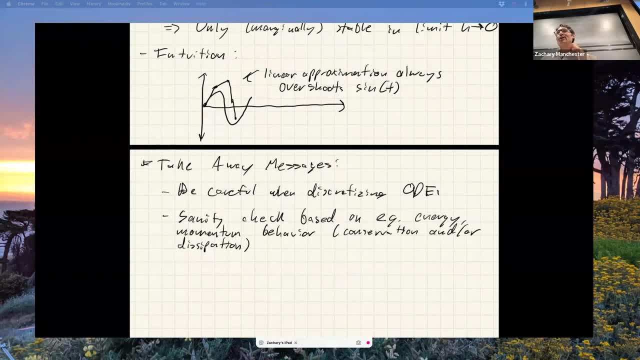 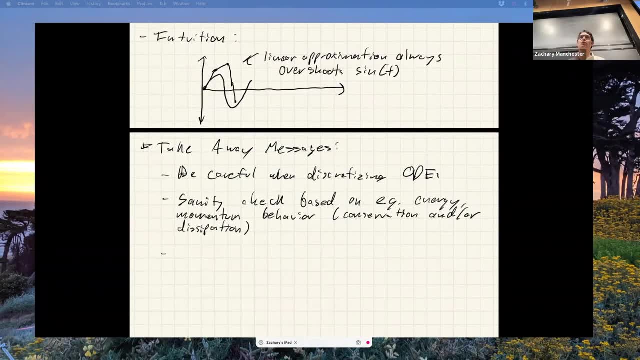 And then, what do they actually do? in the numerical simulation, You'll find that very, very often the simulators do the wrong thing. Things go in the wrong direction, And that's something you really want to be careful about, Like you want to make sure your results are qualitatively correct. 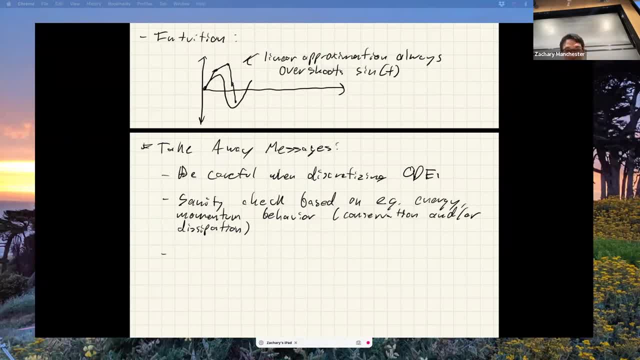 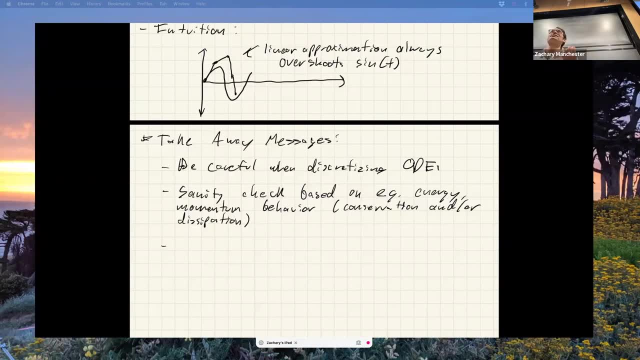 Like: and if it's damped, energy should be going down in the simulator, basically. And then the main, main one is: there's basically never a good reason to use Ford Euler integration. It's super common. It's frustratingly common in robotics and like RL blah. 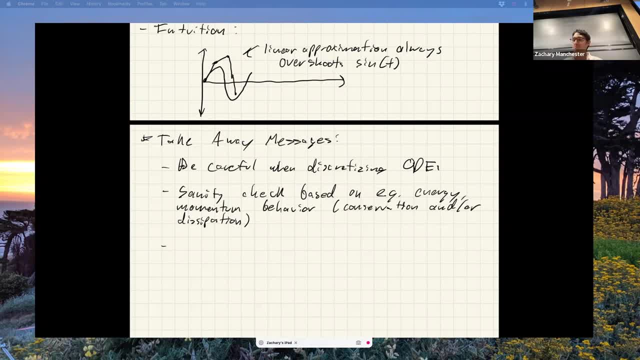 blah, blah, opening iGEM kind of stuff. but there's really no good reason for this. It's basically just laziness, or you don't know any better, and I'm telling you about it now, so you know better now. So don't do it. 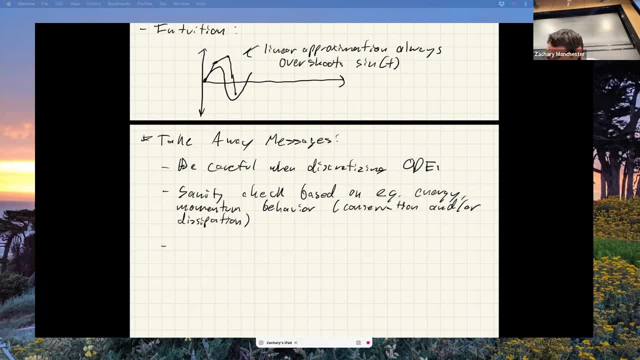 If you do this on your project, I'll be very mad at you. Yeah, Okay. so now if your simulator is based on forward order, so like you can read the docs or or like just try this kind of stuff, right, Do these sanity check exercises simulate a pendulum? 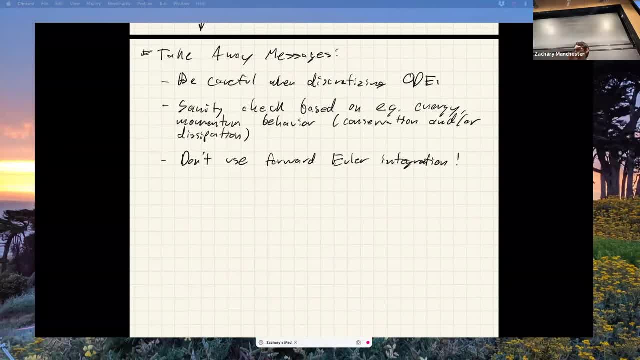 What happens? That kind of thing right. But yeah, like most of these, you can read the docs and you know, understand what they're doing to some extent under the hood, or read the papers like all the comp, like bullet, We joke. 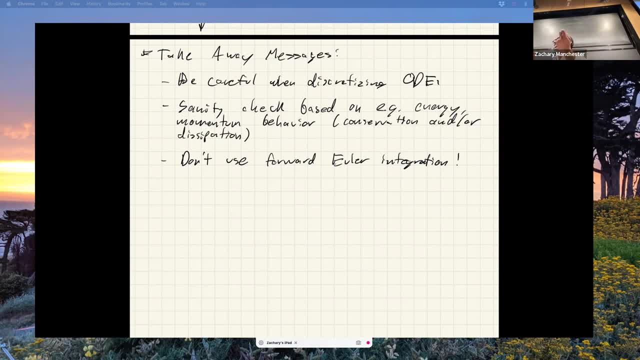 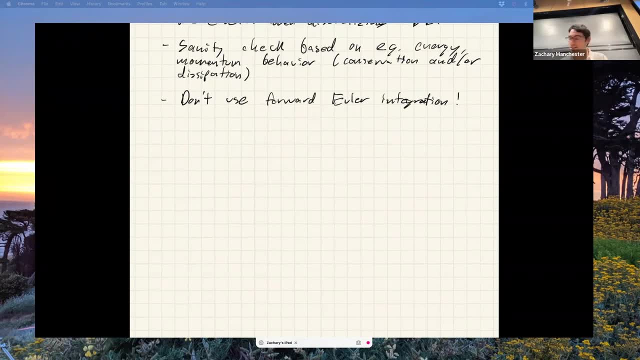 All these things all have good docs, and often there's options for what kind of integrator you use in the in the simulator options. Okay, so what should you do instead? Now let's talk about that. There's a couple things we'll talk about. 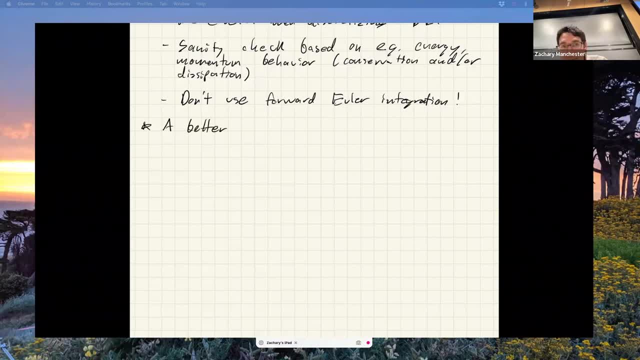 So the first one is sort of probably also most of you know about. So, still talking about me, We talked about explicit. We're still talking about explicit integrator or simulator or whatever We're going to do. fourth order: Runge-Kutta. 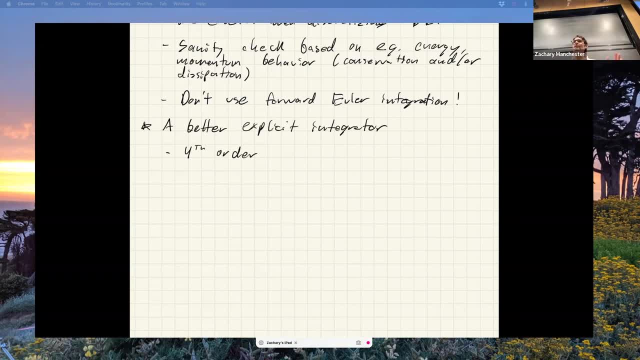 which is the sort of industry standard who's used RK for, like most people, Excellent. Basically, this is the first thing you should try in almost all cases. There's definitely places where this barfs, So you shouldn't like. this is not a blanket- always do this. 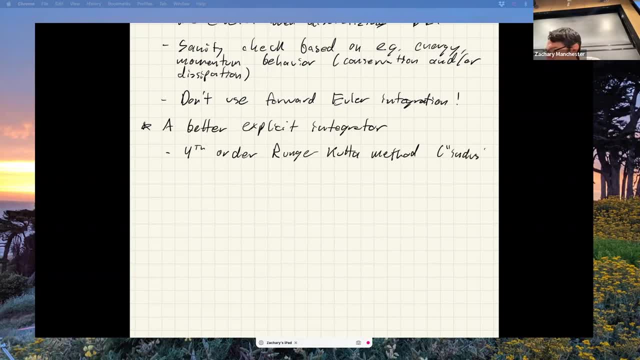 but it's generally the first thing to try. Okay, so the intuition, sort of like general idea for what's going on with this is: remember with with oiler, We were fitting a line right Using the derivative At that time step. 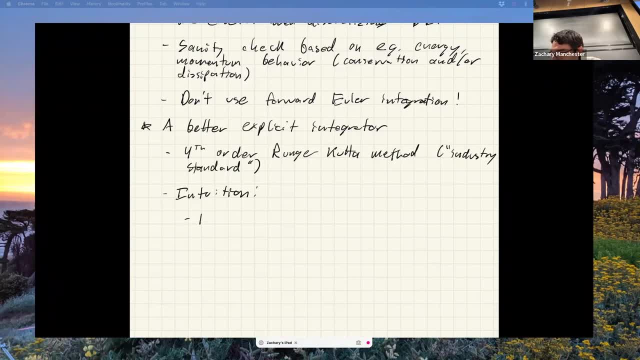 we fit a line, We go along the line. Does anyone know what RK four does? instead, Anybody speak up It. it's a line, goes along the line, recalculates some stuff, goes back along the line and does that. So that's what it looks like. 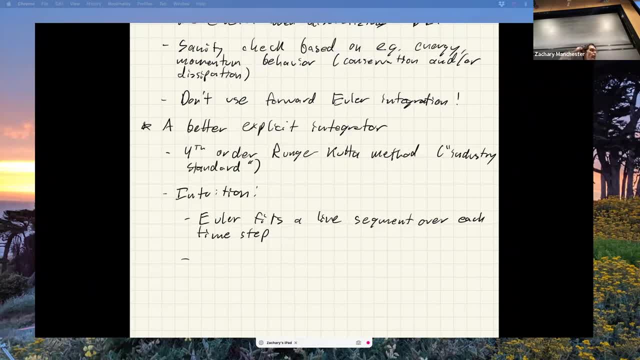 you know, but there's actually a really simple what it's actually doing. If you like, look at. if you derive it, it's fitting a cubic swine. So all those function of how many function calls are there in RK four, Four. 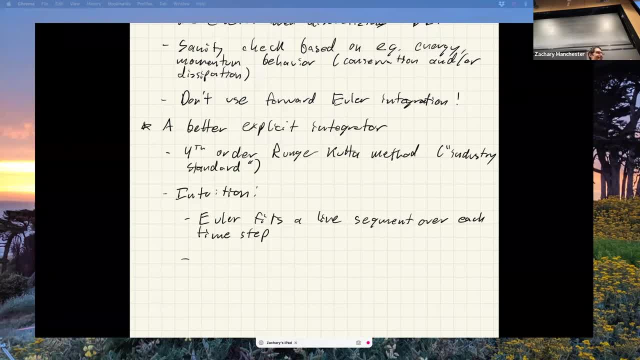 Yeah, So how many, how many points do you need to fit a cubic? That's so, it's literally fitting a cubic spline, And that's how you derive it actually. So yeah, I don't know, That's fun fact, But yeah. 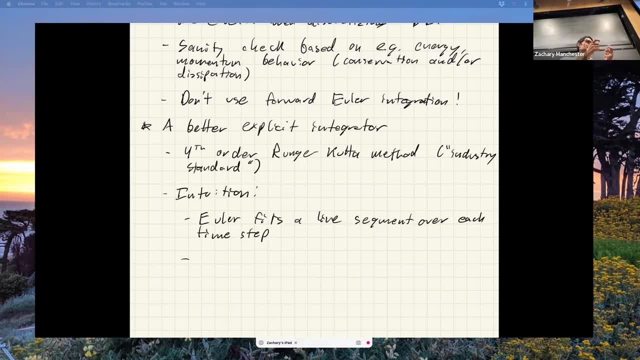 it looks super weird, You know. it looks like you're going forward backward. Really, what that's coming from is actually just running a cubic spline down and trying to fit it with X Dots with four different values. There's actually, it's not unique. 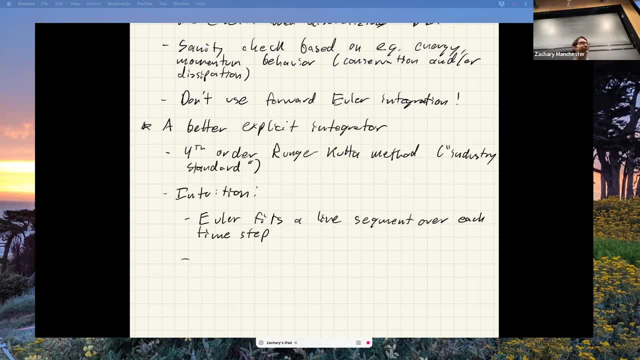 There's actually a bunch of, there's an infinity of RK four rules You could write down because you can evaluate those points kind of anywhere right And still uniquely fit the spline. So there's actually two classic RK fours on the Wikipedia page. 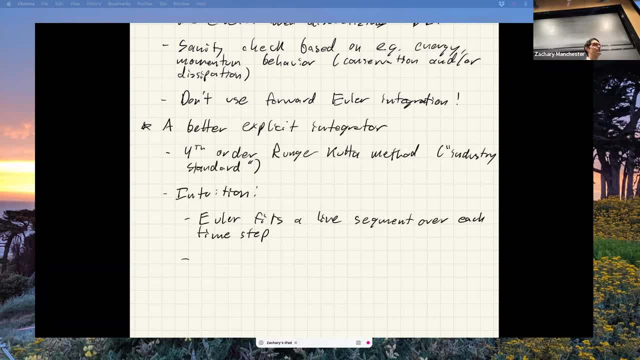 but there's, there's an actual infinite number of possible RK. four rules Change the weights and where you evaluate F right, Because in the standard one you evaluated it like X, K plus a half, basically twice, And at the initial point, at the end point. 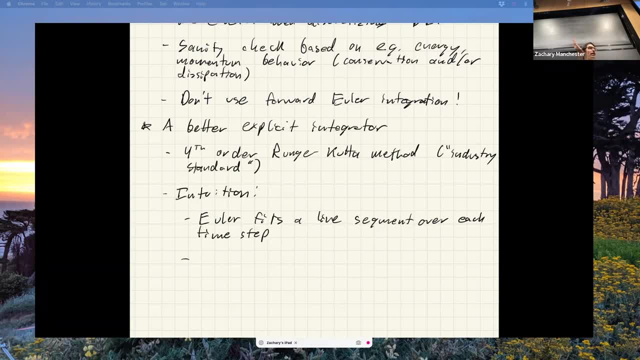 you could have. in principle, you could evaluate it anywhere on the interval right And like all kinds of different ways. So there's like a sort of full infinity of possible versions of that. Yeah, Yep, It's a long conversation. 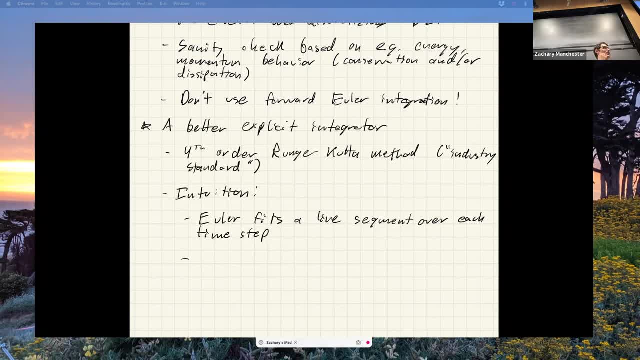 Basically. there's this notion- This is probably too long to like do here, We can talk after. there's this notion You may have heard of, called stiff ODS. Have you heard of this before? Anybody heard of this idea before? 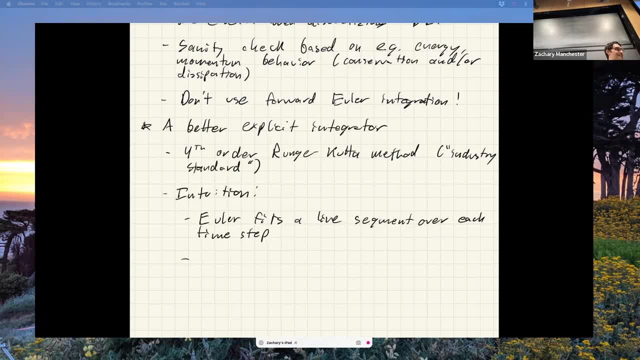 So stiff ODS like generally corresponds to things with like high stiffness from like a mechanical kind of perspective, like really high stiffness constants or damping constants or whatever in your ODS somewhere. Basically, yeah, RK four or, in fact, any explicit 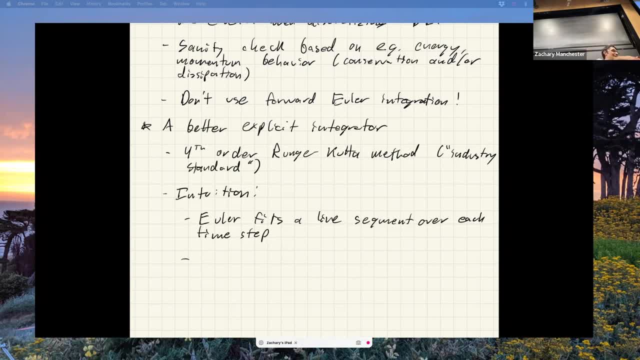 This is why we talked about explicit. We're going to talk about implicit integration rules next. Basically, you can prove mathematically that any explicit Runge-Kutta method, any, any RK method that's explicit like that, will barf on a stiff system there. 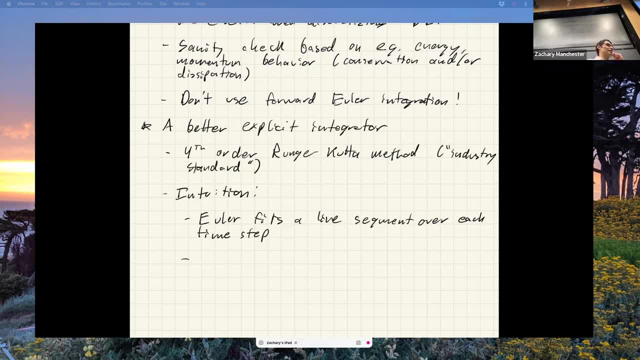 They, they have certain. there's like a, this notion of stability that we're kind of talking about here, that we're kind of dancing around. You can actually, You can actually prove that any explicit integrator is not what's called a stable Basically. 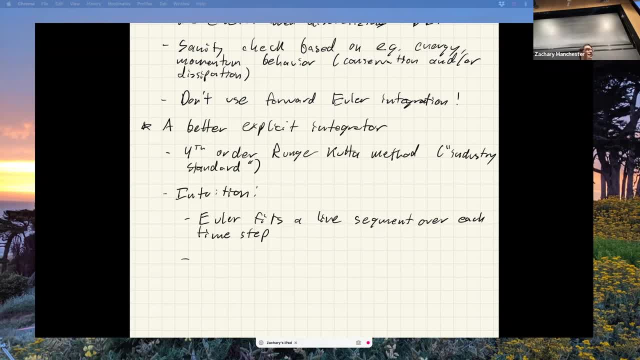 there's certain stability properties that you can't have an explicit method, and so for a sufficiently stiff system it's going to barf and blow up on you kind of no matter what. but for relatively benign things, RK four is like pretty much the the go-to. 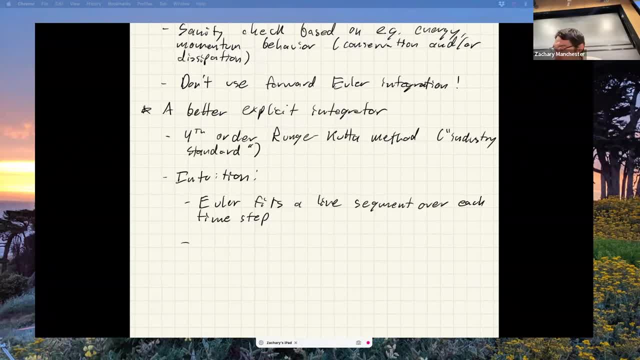 Okay, have you talked about that? But I'm going to try to keep trucking here. So yeah, RK four, which many of you seen before and probably used a lot, is just fitting a cubic spline and so kind of like, obviously, fitting a cubic spline versus fitting a line. 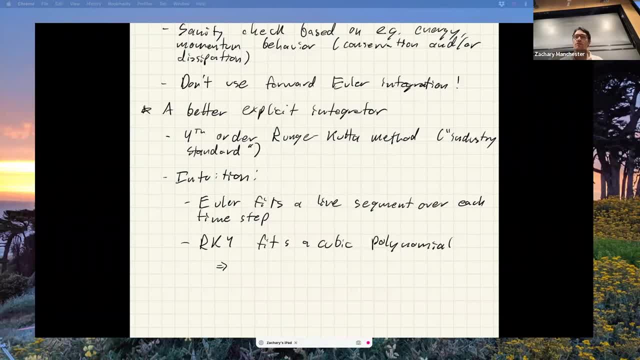 You can get much. It's much more expressive. You can like have a much better fit to the true underlying solution. so you get much better accuracy. It's also obviously four X more expensive to evaluate a step with it right, But it turns out the the win in accuracy is way more than four X. 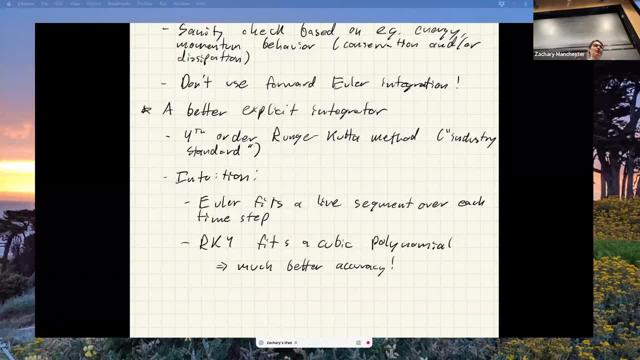 The win is like to the fourth power. So, like it turns out, the win in terms of accuracy dramatically outweighs the compute computational cost of. like the. it's basically a constant more expensive, but it's like a high power, more accurate, right, So it's. it's always worth it. 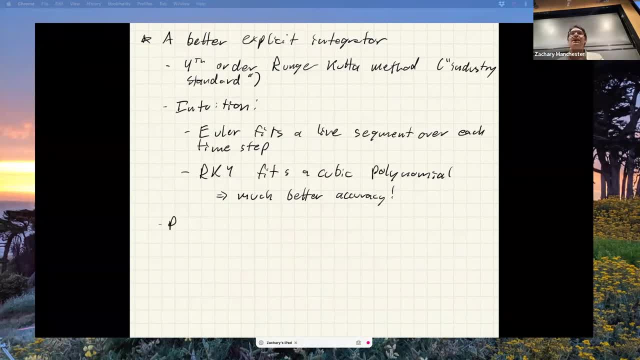 Okay, so this, we're not going to drive this because it's actually a huge pain, but you've- most of you done it before. I'm going to just kind of write this: It's a pseudo code for it, and then we'll like do the real code, basically. 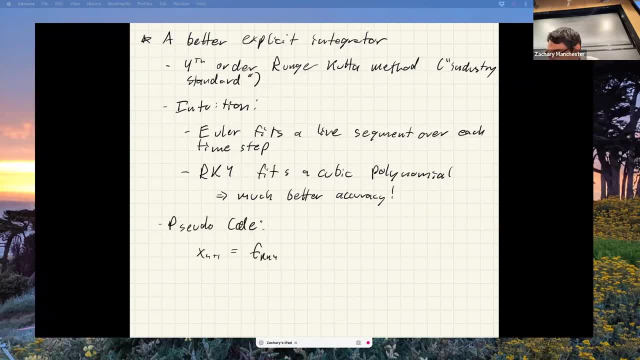 looks like this. We'll call this F? Rk Four. That's sort of terrible handwriting, Apologies. So here's. this is like there's a lot of. this is kind of a standard way to write this down with these little Ks. 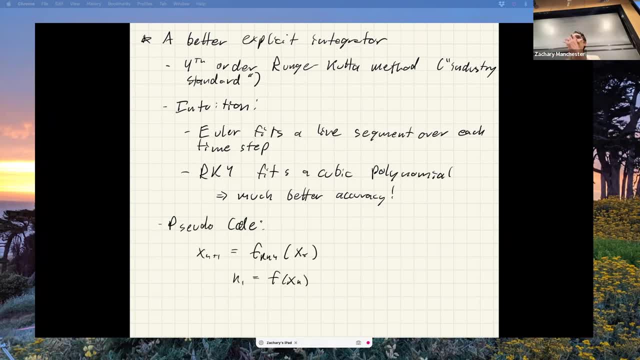 Basically, you evaluate F at the current spot, then you take a half step of oiler- Actually, so you do like H over two, K one- and then you do another half step of oiler, but using K two, and then you do a full step. 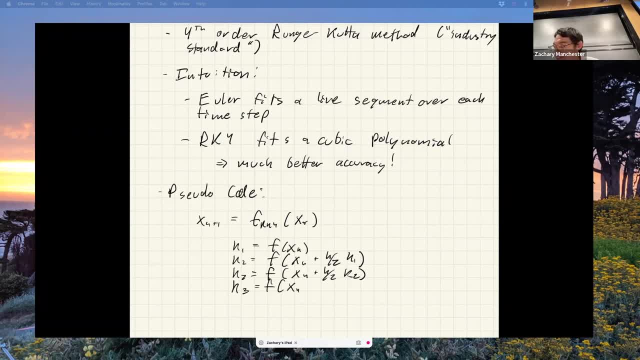 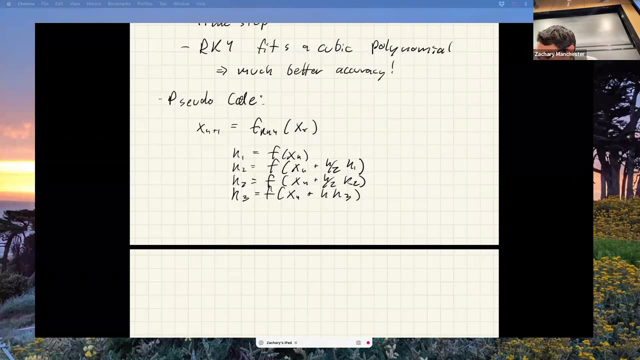 with. this looks super weird and makes no intuitive sense, But where it comes from is basically writing down the spline and then saying: you know, I want to fit the spline kind of thing right, And then, at the end of the day, the actual 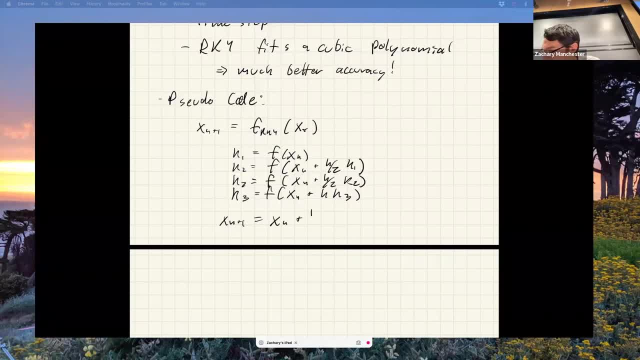 the actual solution to this is the following: Has anyone seen Simpson's rule? Find a chance, Let me know what that is. Yeah, Does this look like Simpson's rule? It is the same thing, which is, where does Simpson's rule come from? 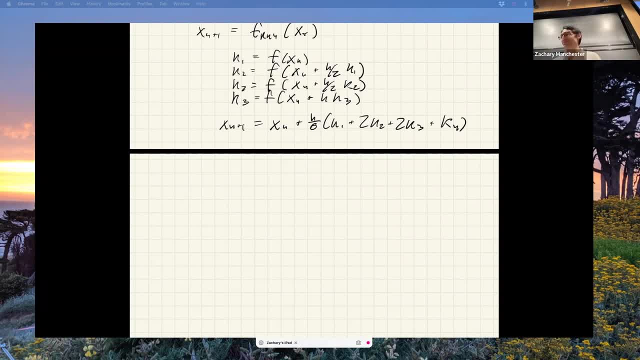 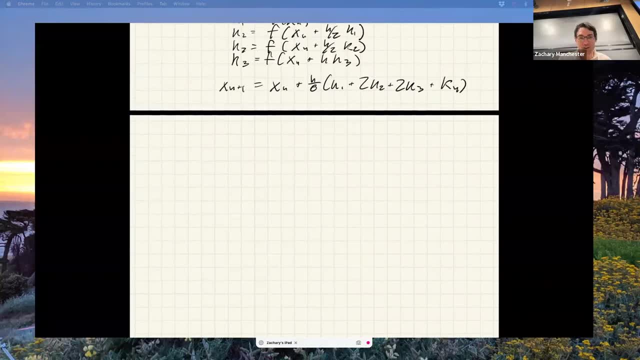 It's evaluating integral using a cubic spline, which is where this comes from. right, It's the same. They are capable and Simpson's rule is the same thing. Okay, fun fact, What else we got here? Okay, so now we're gonna do the pendulum thing again. 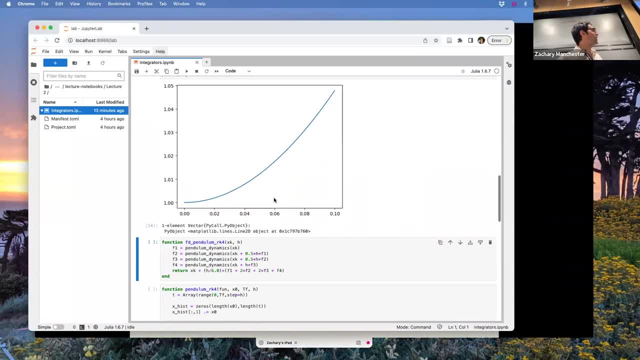 but with RK four we'll do the same stuff and like: take a critical look. Okay, so here's RK four that I just wrote down. So you know code four. Yeah, that's what I just wrote, right Cool? 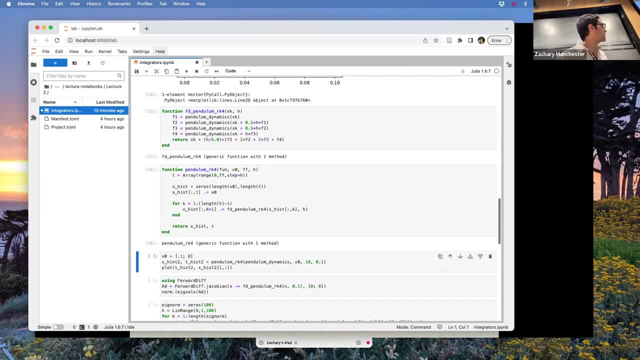 And so we'll do the pendulum simulation thing again. This is just calling it for a bunch of time steps. same kind of stuff. We'll do 10 seconds at 10 Hertz, I guess Same initial conditions as last time. 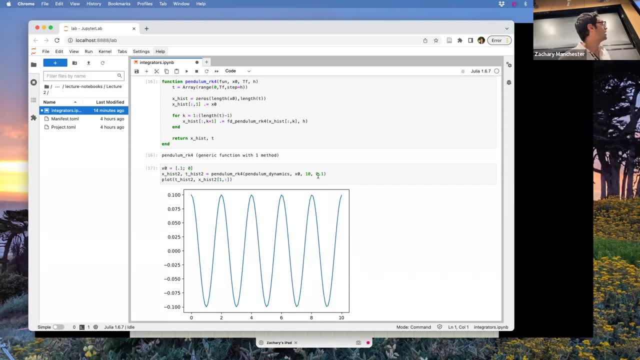 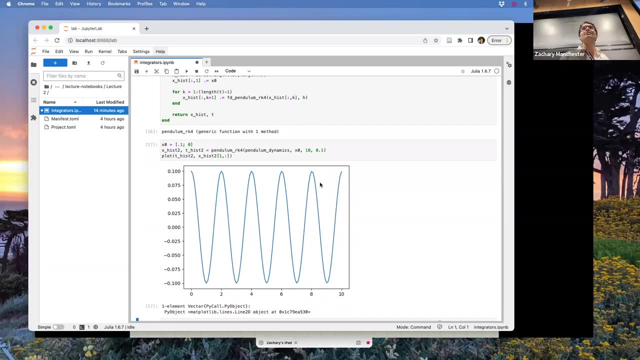 right, That looks pretty good. Hey, how about that? In fact, I can take like even bigger time steps and it's still pretty much rock solid. You want me to try anything? Okay, sure, So it's slightly damped actually. 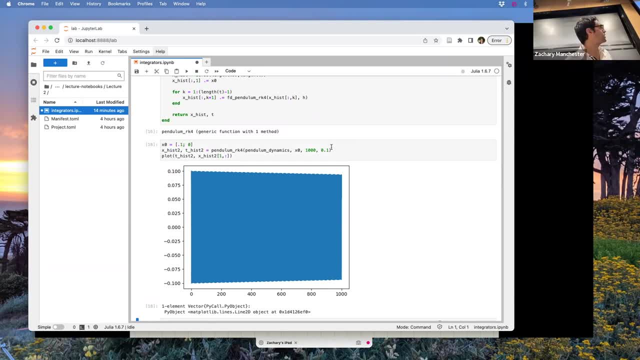 right, But it's pretty good And if I take like slightly smaller time steps, you know it'll basically look perfect. So if I went to like for sure you know 100 Hertz, totally, you know stable. 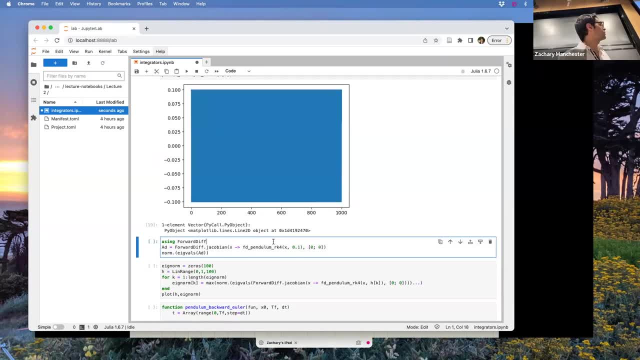 right, Like what it's supposed to look like, right. That's pretty great. So what we're going to do now is: I'm not going to handwrite the Jacobian at this like I did last time, because it's a lot more annoying. 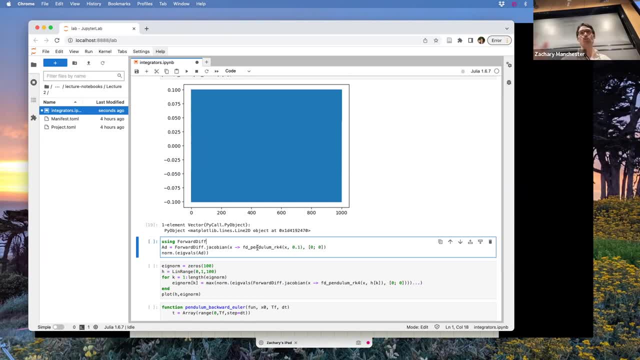 We're going to use four diff to get the Jacobian. This is what it looks like It's being on homework zero. It's super shape work. But yeah, the fact that auto-diffing is built into Julia, it's pretty great. 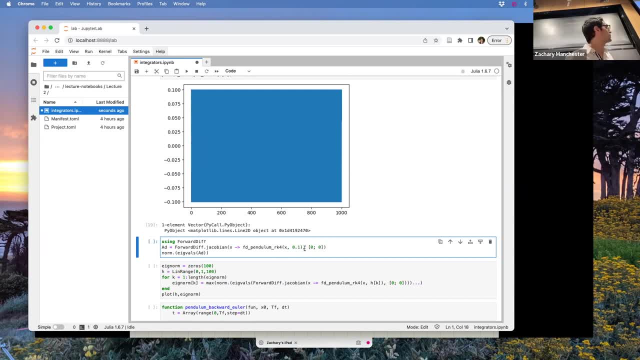 So we're going to do the four diff thing and I'm just going to give you that, that RK4 step right, And we'll do the 10 Hertz sample right, Say, and we're going to check those eigenvalues. 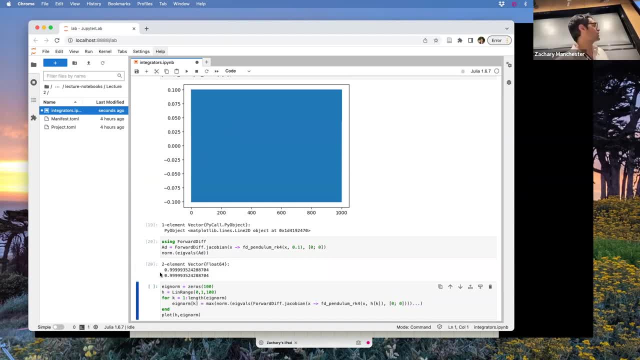 Remember they're supposed to be one, right? So look, that matches what we expect out to like five decimal places, right, That's pretty good, And you can tell actually from here it's slightly less than one, So it's slightly damped actually. 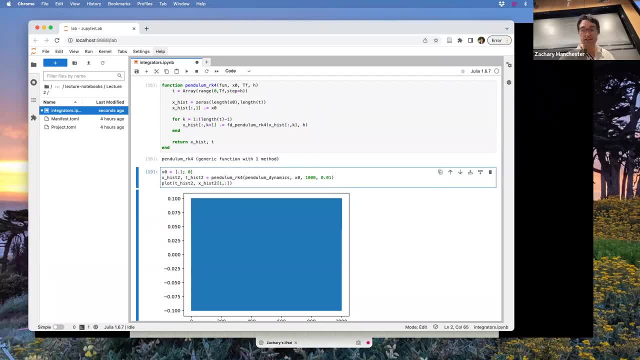 which exactly matches the behavior we saw up here, right? So if I put this back to 10 Hertz it's a little damp, right, But it's out at the fifth decimal, So it only shows up after like a thousand seconds, or. 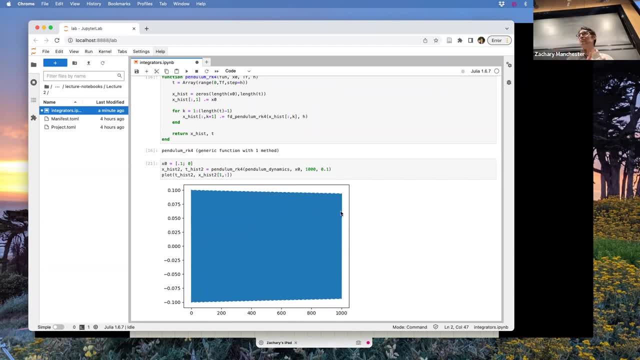 whatever, right, Pretty good. Any thoughts? questions: Want me to try anything weird? Yeah, just like floating points. but no, they're not. They're coming from the underlying, like cubics one bit right there. So they're not. 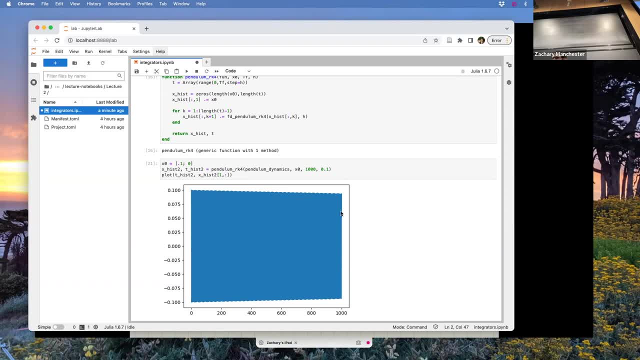 this isn't like floating point around off error, right, We're way like, way, sort of before that. This is actually like associated with this, like discretization that I've done to the dynamics. right, The cubic spine fit the rk4 thing. 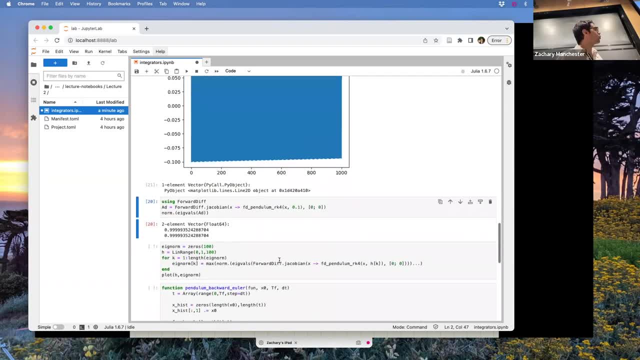 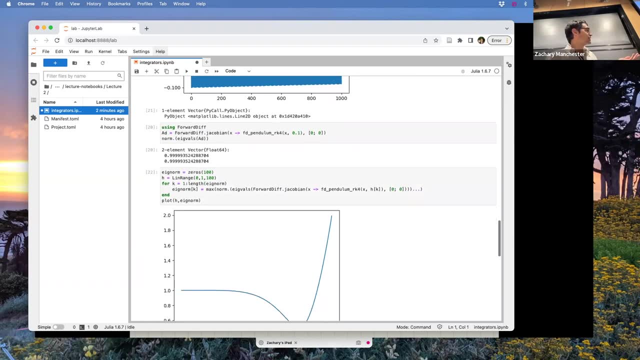 blah, blah, blah. Yeah, Okay, cool. So that's this. So we're going to make the same eigenvalue plot as a function of H and see what that looks like. This is kind of fun, So check this out. 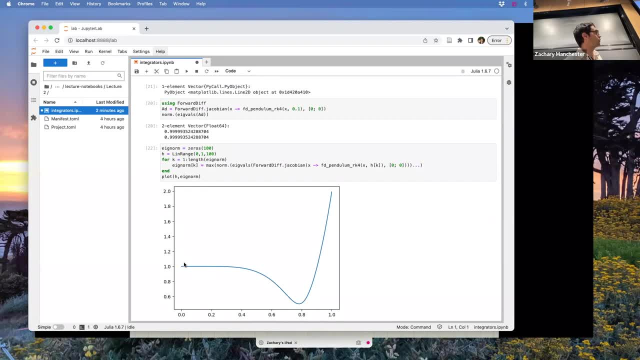 It's supposed to be one, right? So for sufficiently small age, like around 10 Hertz, you know, even up to like, this is like five Hertz, right? So even five Hertz, it's still pretty good. 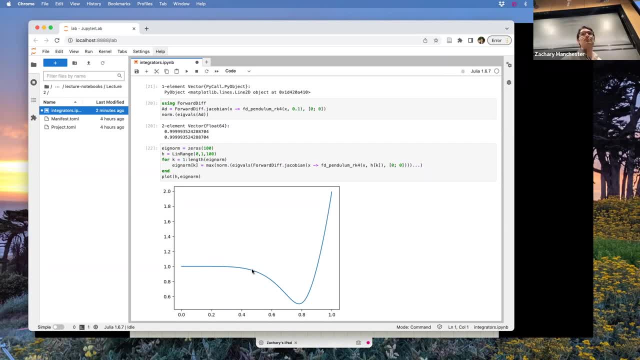 But then, you see, as I make the time steps bigger, it starts to become damped, artificially damp. So we're now we're losing energy Artificially, And then, if I go even bigger, it sort of turns around and now it's adding energy and blowing. 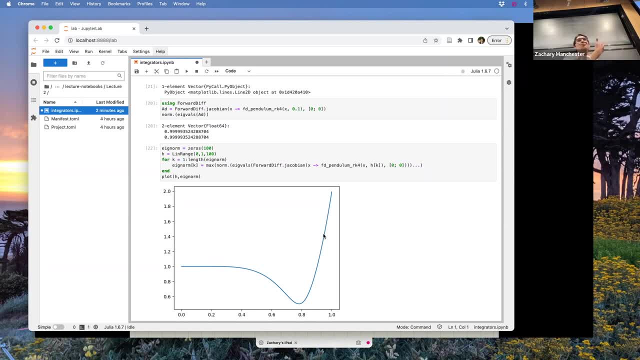 up like we saw with oily. That's super weird And like I don't know. there'd be no way to kind of predict this from you know first person. We just try it, but kind of cool. They don't want me to try some of these things. 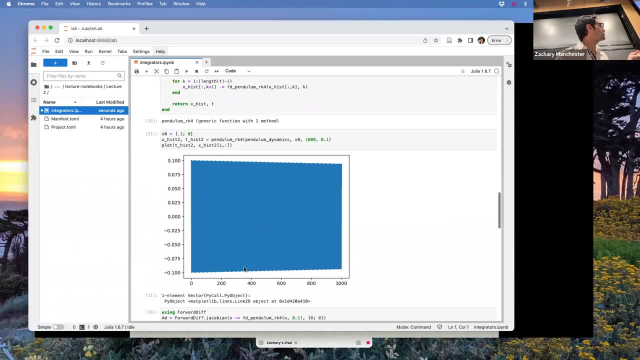 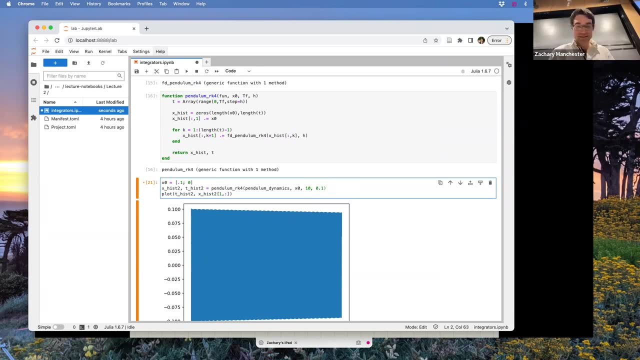 We can try. I don't know, We can try point for something that might not be so gross. See what happens, Maybe 10 seconds, So it doesn't go insane on us. So yeah, now it's like, but also, 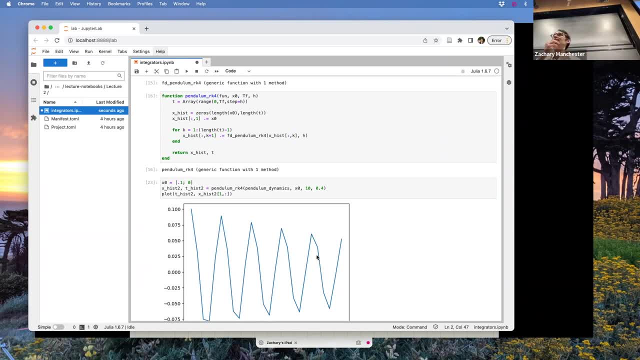 you know we're starting to run up against, like Nyquist, Sampling problems. right, It's super course. Yeah, 100% Yeah. So what really matters here is sort of like the ratio of like the natural frequencies to the integrator step size. 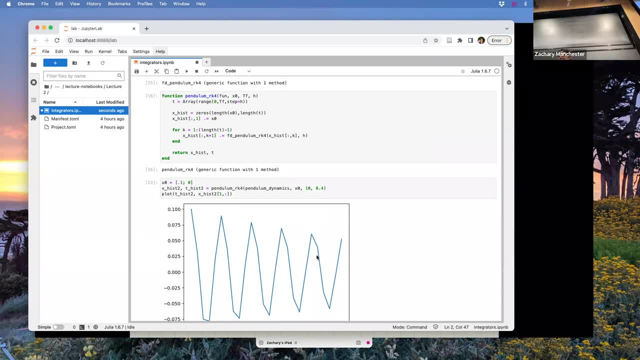 right. So if I want to change the length of the pendulum and made the natural frequency of the pendulum like 10 times faster, all of this would get compressed by a factor of 10, right, I have to sample 10 X faster to capture the dynamics. 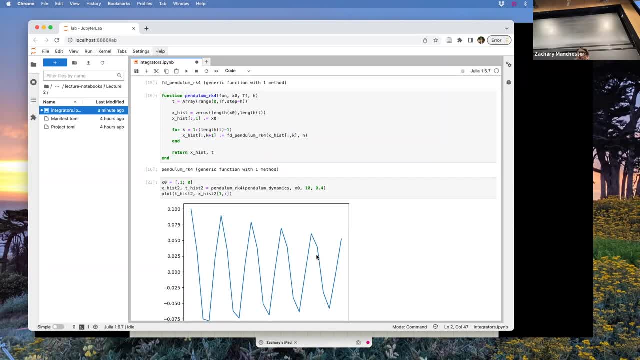 It's really yeah, you nailed it. It's basically what matters here is, like the integrator Step size relative to the frequency content in the solutions right In the dynamics. Yeah, And then the like the Nyquist frequency aliasing stuff has to be added. 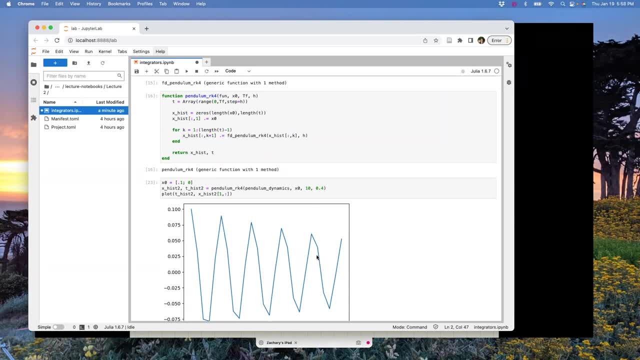 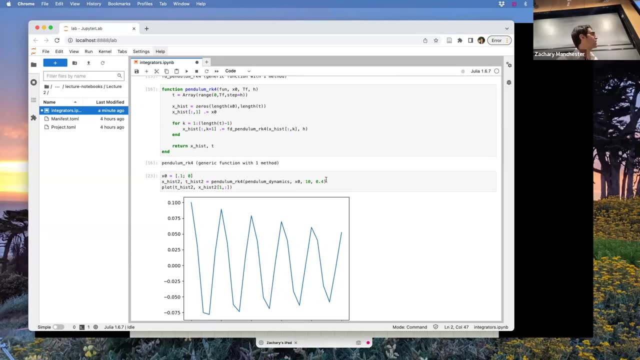 on to that RK for error plot. It's like, yeah, so that's actually sort of a separate issue and it turns out right because you're fitting a cubic, you actually can under sample here So and still get accurate solutions right. So you're not actually just remember. 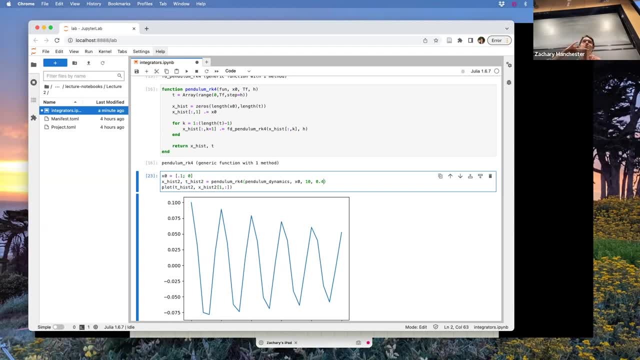 right I'm actually doing for function evaluations per RK Step. So I'm actually like not quite like if I did this, you know, if I made this H large enough that I wasn't quite at Nyquist, I'm actually still okay here. 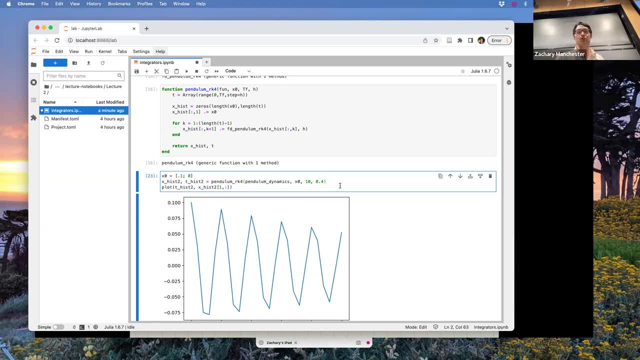 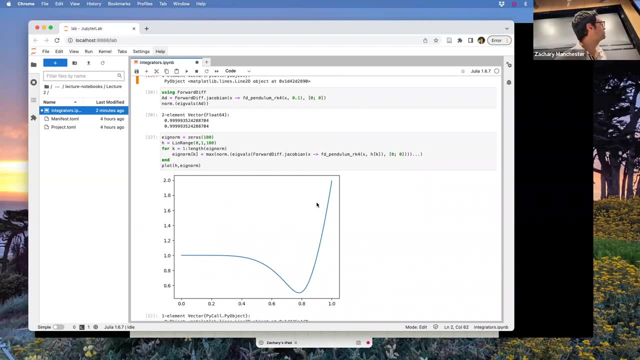 But you're, you're right, The Nyquist thing is going to pop up here eventually And these are kind of separate issues. Okay, Yeah, And like I don't know, I could get this to blow up by going out to like 0.9.. 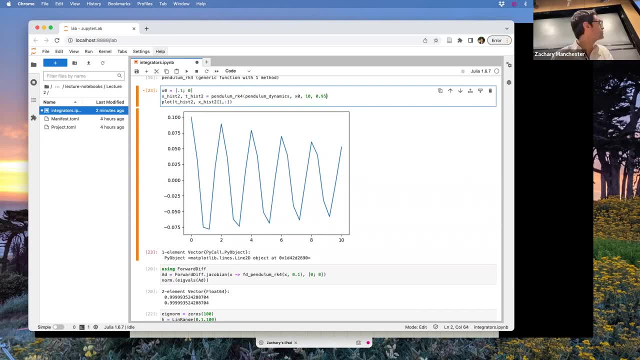 Maybe let's try that Think point. Let's say 0.95 or something. That's it. Clearly, Now it's blowing up and I'm also like way under sampling Also, The solutions look kind of garbagey. But imagine if I did cubic interpolation of this and actually like 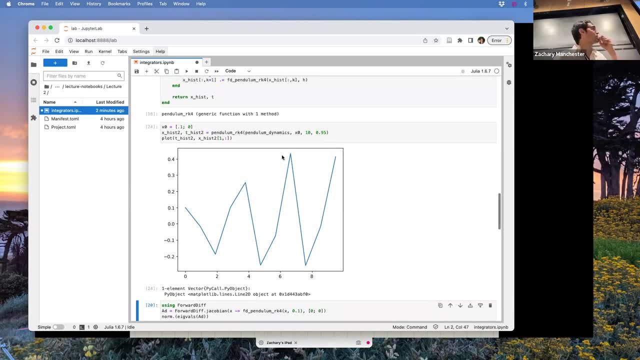 up, sampled it, it wouldn't be that bad. It's still kind of like saying we're not quite at like Nyquist, badness right. Okay, Any questions about this And I want to try anything else. Weird, This is kind of fun. 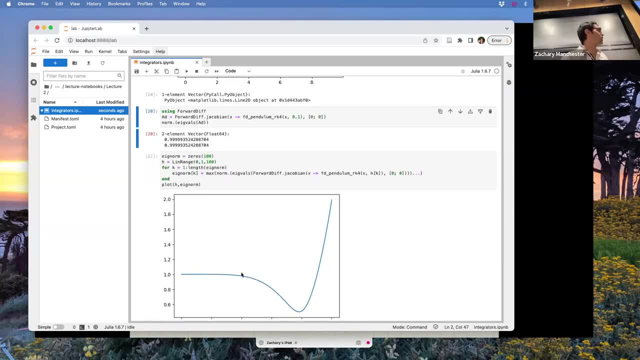 I think this is cool. So yeah, basically it's pretty easy to make this sort of plots and like the messages you know, obviously there's this whole like you want to take reasonably small time steps If your time steps are huge. 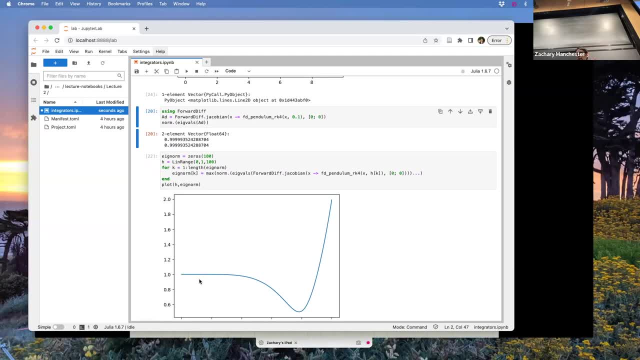 we all know bad things are going to happen. But there's also this sort of Error thing. It's a little more like insidious. That's a function of the exact way You're discretizing the dynamics and different Runge-Kutta rules. 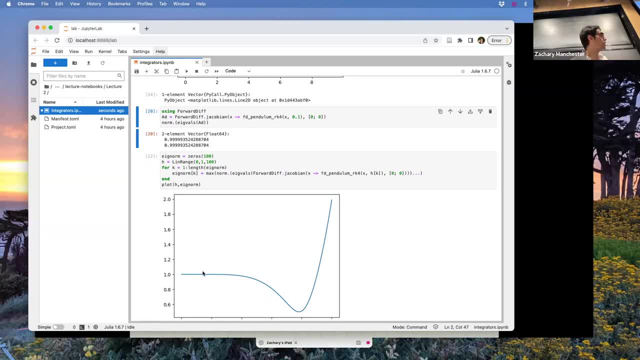 What different behavior in this kind of setting and generally. you know, everything's cool when the limit is H goes to zero. but we can't simulate it. H goes to zero, So we got to pick something finite. and here you know. 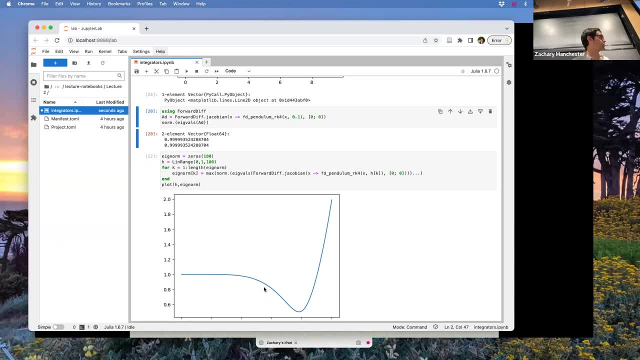 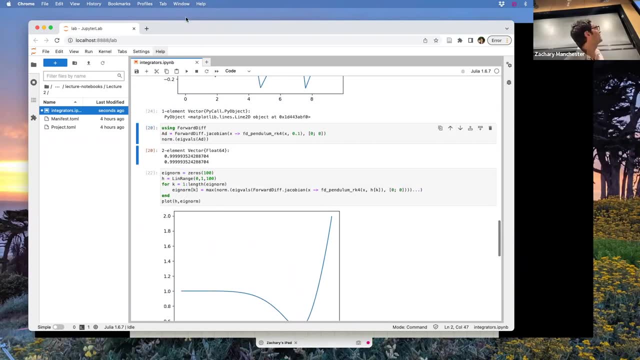 you're good for a pretty good range of pages with our K four. Eventually, it's going to start to do weird stuff, So you always have to worry about this. Okay, cool, What's this? Yeah, we're not going to do that yet. 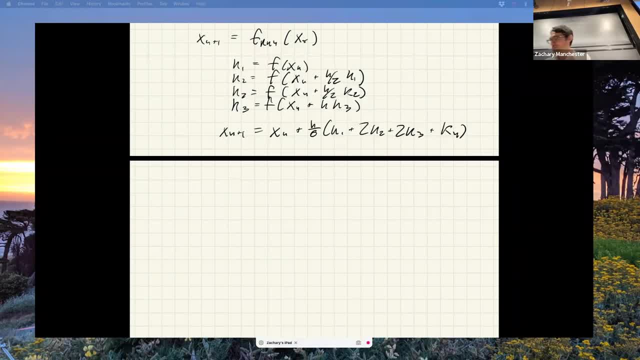 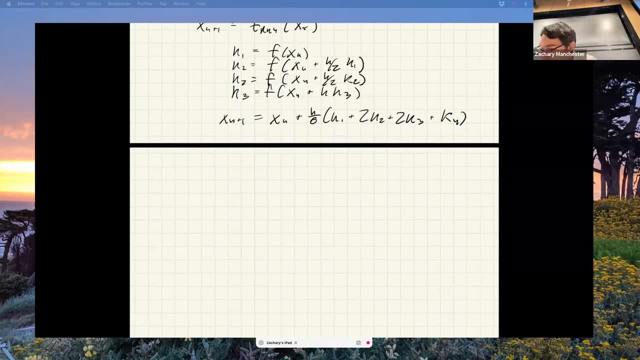 More to come. Okay, Cool, Let's keep trucking. Hopefully my iPad didn't die. Okay, Yay, Let's go live. Okay, so, So yeah, a couple takeaways. First one, the accuracy. I just said this. 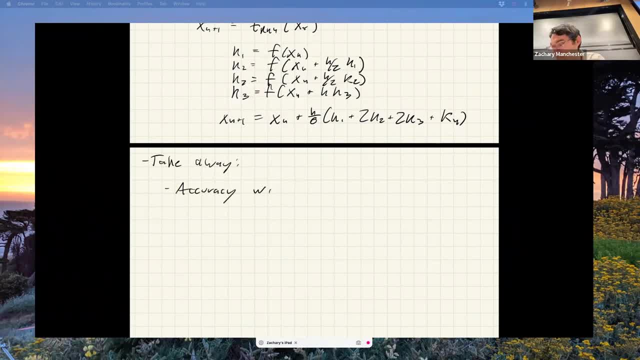 but you'll just have to trust You can try this yourself. You should try it yourself. Shouldn't believe me, right, I'm not. the accuracy When here is sort of way outweighs the additional computational cost. I mean that should have been kind of obvious from those plots. 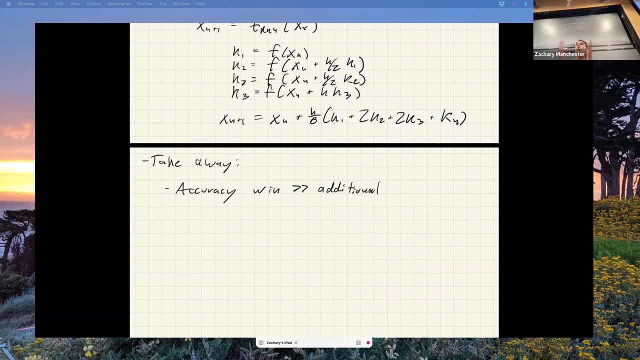 right, Like it's way more accurate, Even if you took like 4x the time stepped. you know size versus Euler, So then the computation cost would be the same. right, You get way better accuracy with this. Let's see what else. 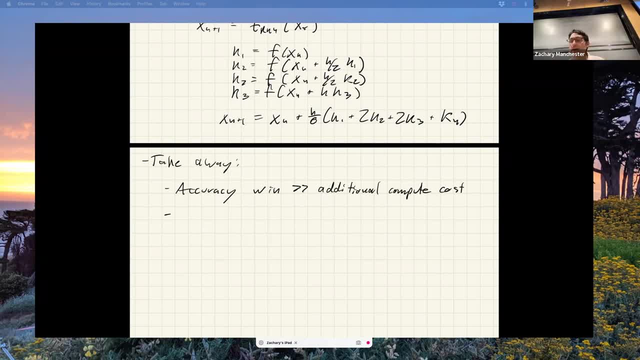 Yeah, So, and then again, this is like a, you know, reasonably sophisticated integrator, right? And even here weird stuff happens as a function of the step size, if I take bigger steps and stuff. So even with fancy integrators, 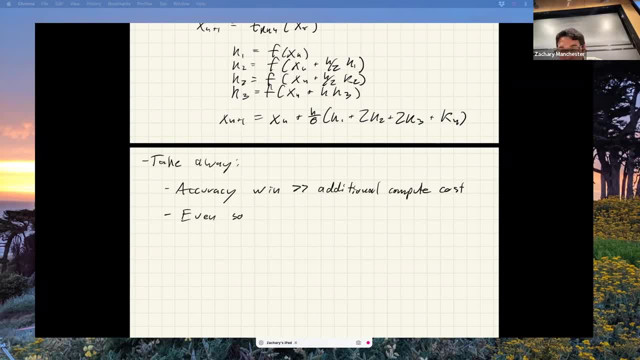 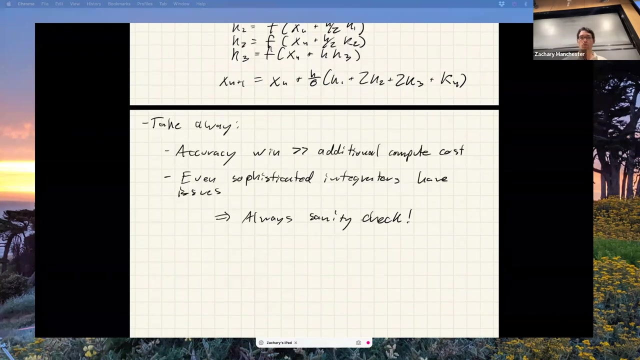 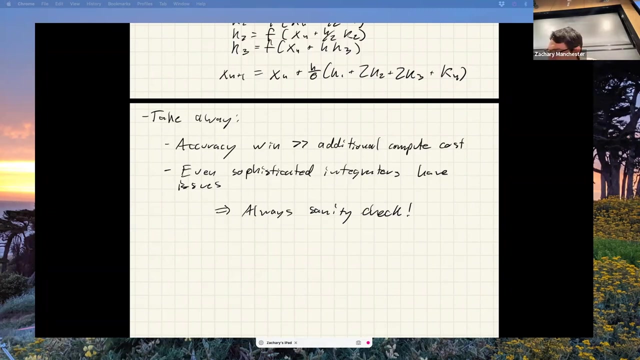 you can't trust them And you should always kind of be a little bit wary. So always do some sanity checking. Okay, cool, Any questions about any of that? Good, All right. So the next sort of like thing to talk about, then, is those. 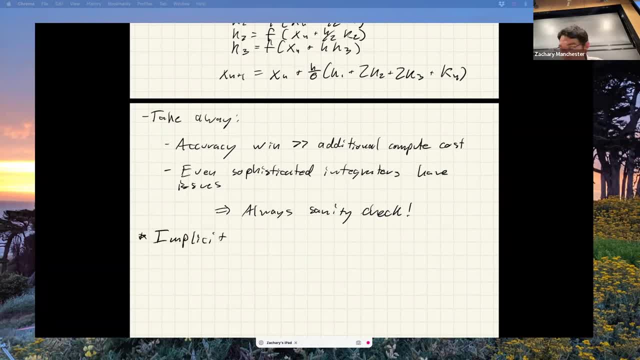 those were explicit. We're not going to talk about implicit discretizations, implicit form, whatever you call this. So here, what this looks like now is it's an implicit function, right, Rather than an explicit function. So now this FD looks like X K plus one X K U K. 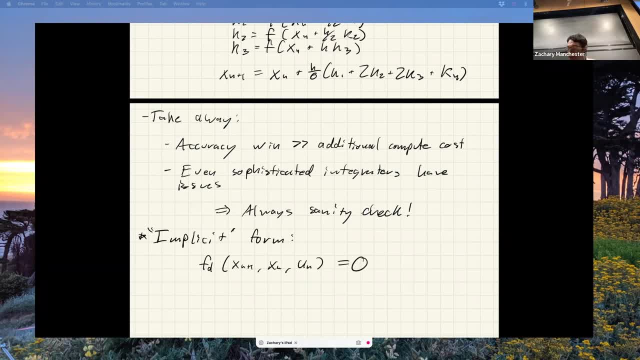 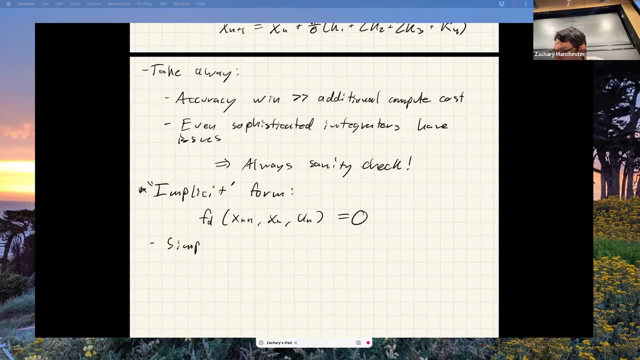 Equals zero. So maybe it makes more sense to make a concrete example of this to explain it. So the simplest version of this is called implicit Euler. It looks just like explicit oil that we already saw, except the F is evaluated at X, K plus one instead of. 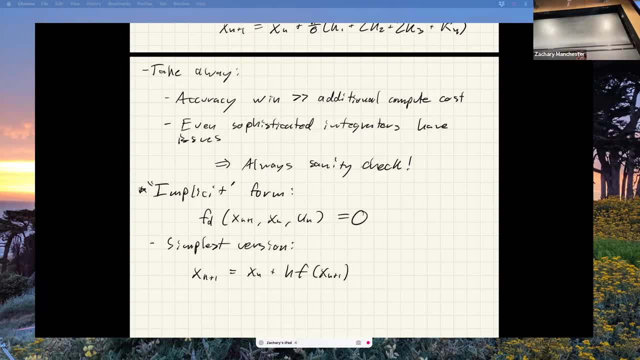 X, K, So it's called implicit Euler. Sometimes it's called backward Euler. So let's see, Yeah, and the main thing is red. This is at the future time. Just kind of weird. So anyone know how we actually do this in practice. 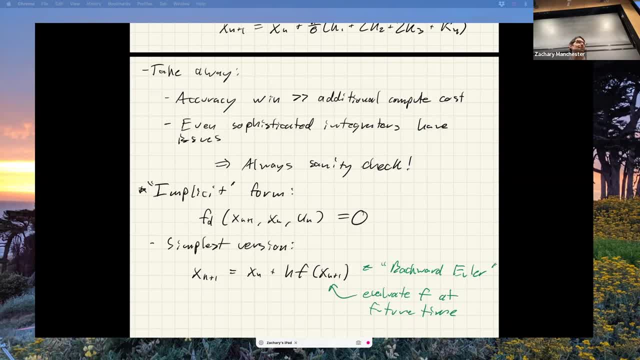 Yeah, just think. Yeah, it's a root finding problem. So I make a guess at X capable. So I know X, K and our UK, because that's what I'm doing to the system right now. So I plug those in and then I take a guess at X K plus. 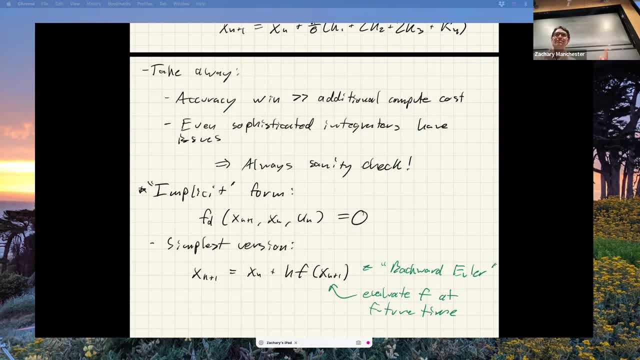 one And the simple same guess is just X K plus one as equals X K as the initial guess. You plug all those in to this equation, move everything to the left hand side, right, It's not going to be zero. So now you just solve a root finding problem in X K plus. 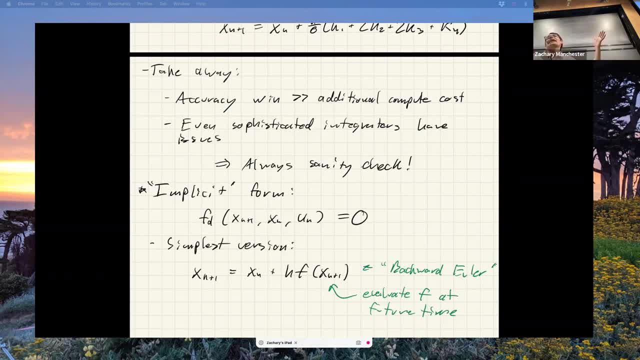 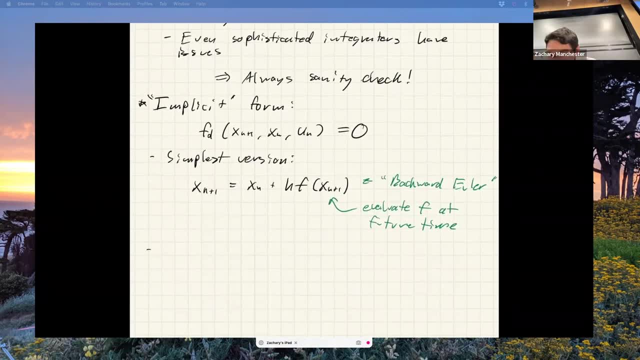 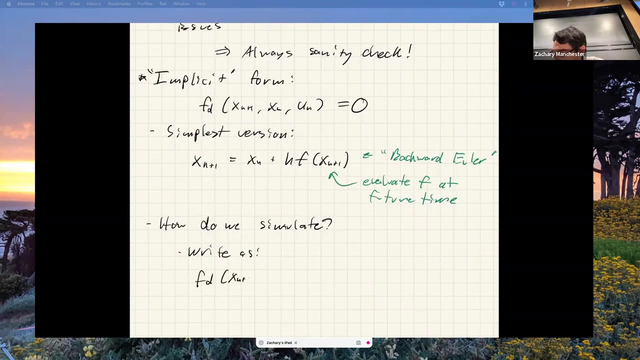 one until you drive the error to zero, And now you've got X, K plus one. That's how you actually do it right. Okay, so let's, let's do that story. So do this Right. We move all the stuff that I just wrote over. 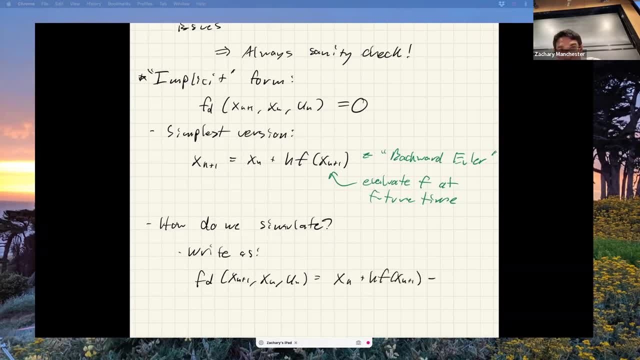 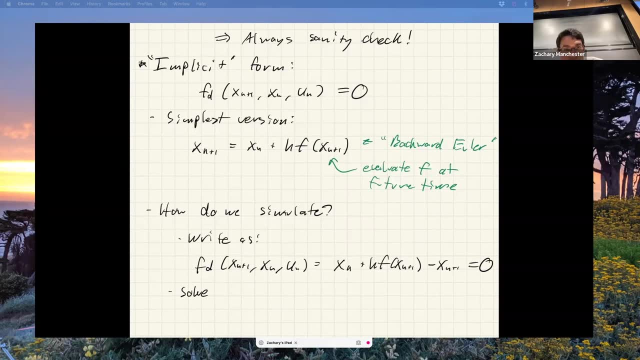 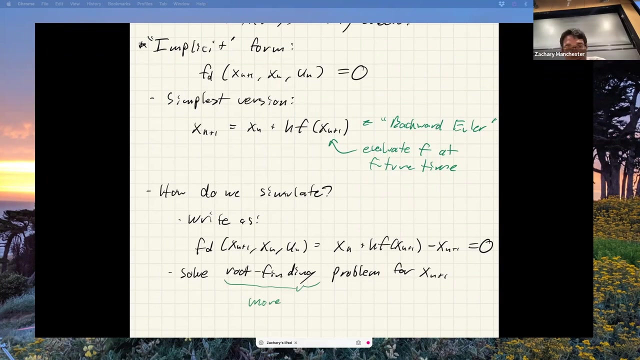 So it looks like this And then we solve a root finding problem. That's pretty terrible. Practice is one, So we're going to talk more about this next week When we talk about optimization. So probably a lot of you know how to do this. 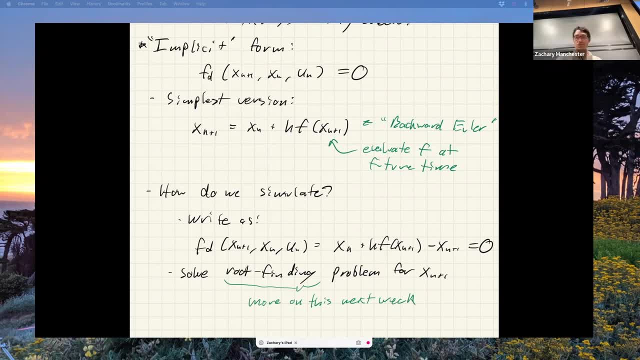 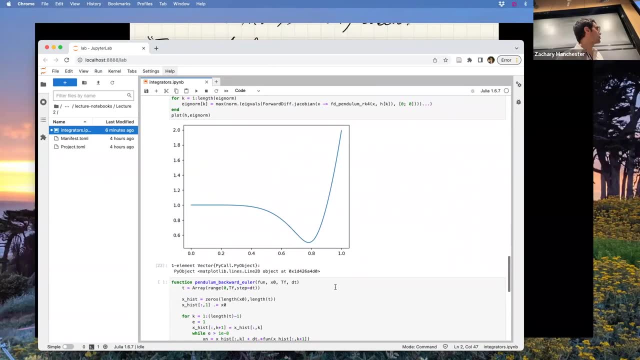 So we'll save it for next week. So what we're going to do is I'll just do it and I'll show you the code, and then next week we'll talk about how to be refining. Okay, So here it is: backward oiler. 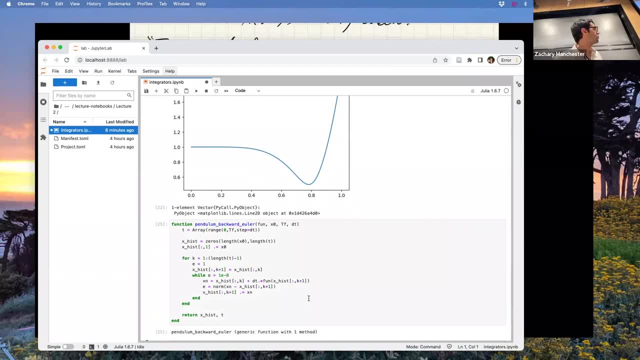 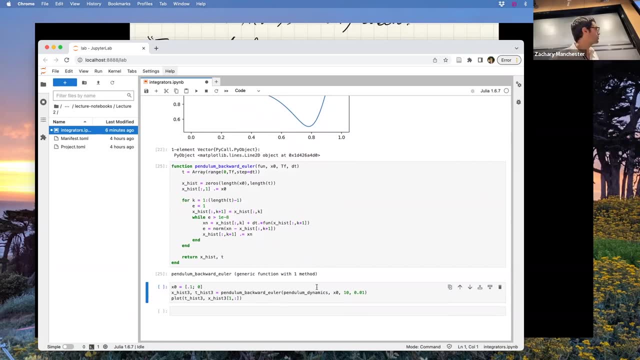 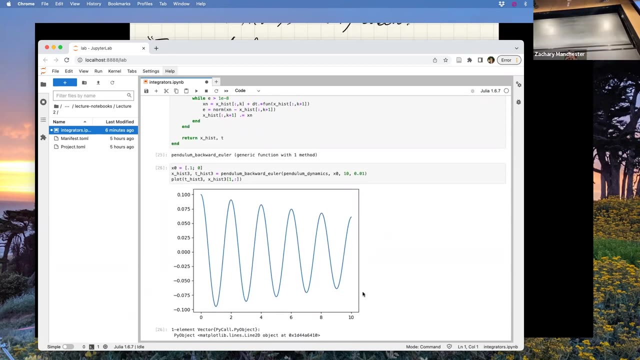 Yeah, This is, and let's plot The thing. So this is like 100 Hertz, Let's do it. I'll do 100 Hertz and see what happens, What's happening, What's going on thoughts. So first, 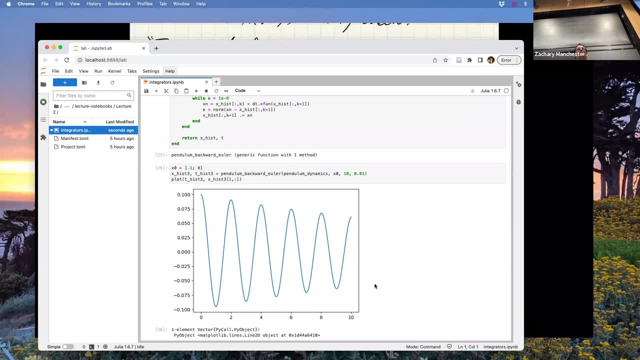 I just the obvious thing is that it's damped right, It's losing energy, which, again, it's not supposed to do right, It's supposed to be constant. So here, like the important messages, this has the exact opposite energy. 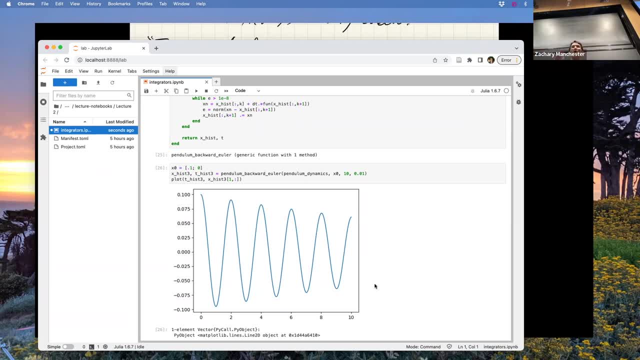 Behavior of explicit oiler, So explicitly is there. you're always overshooting because you're evaluating it at the XK and you get this energy blow up. It turns out with this guy, the implicit or backward oiler you're always evaluating at XK, plus one. 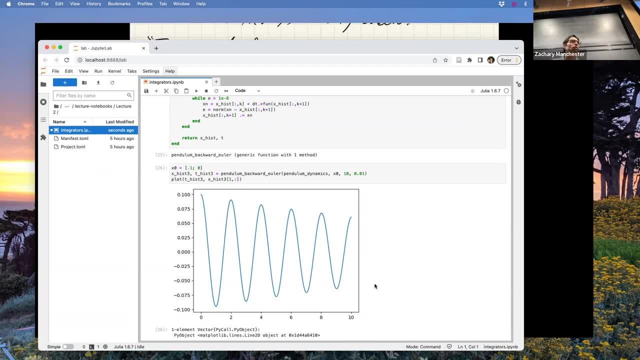 You're always under shooting, the true solution And so, therefore, you're always. you're always losing energy. You're always like. you get this artificial damping effect And again, just like the last case we saw, it doesn't matter how big. 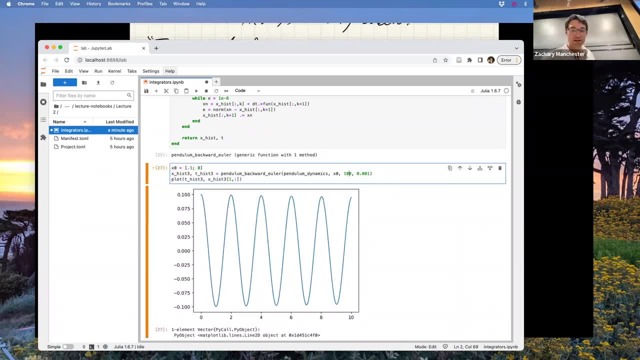 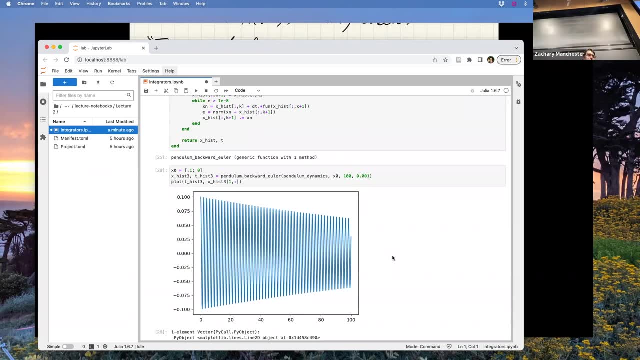 you know how how much I crank the time steps down, Like if I go out long enough. the same behavior is there right. Kind of interesting, Although, yeah, from a practical perspective I'm trying to make a simulator that doesn't look stupid. 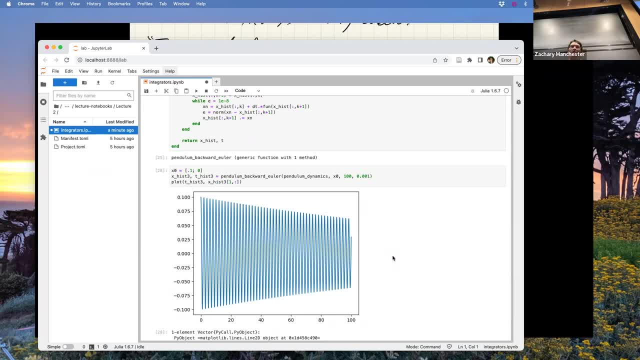 This behavior is preferable in a lot of ways to the blow up behavior, right? So it turns out that this implicit or backward oiler is actually, in spite of how seemingly dumb it is And the fact that has this, pretty nasty you know. 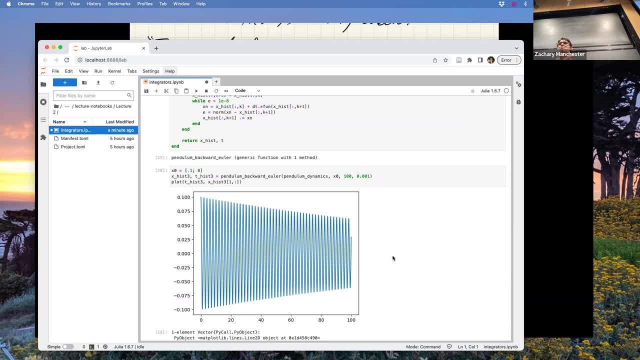 dampening behavior. This is actually super common. Like most of the, the robotic simulators do this. So the default integrator in Budroko is this. default integrator in pie bullet Is this? it's really really common, So beware. 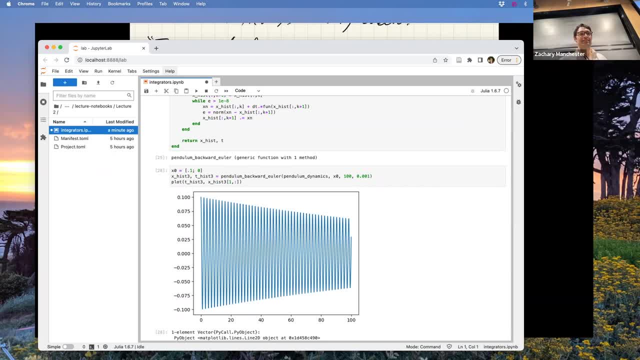 Yeah, So this is the exact opposite. in the error. Can you keep running both You know in an average time to get? that's not a bad idea. You're on the right track to something Cool, So actually that works What you just said. 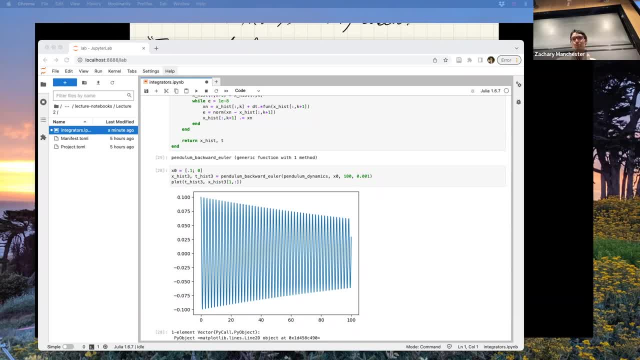 it turns out. if you do that out, what you get is something called the implicit midpoint Rule, which has actually been on your homeworks and it turns out it does exactly what you expect. So good, good intuition, It's a very good idea. 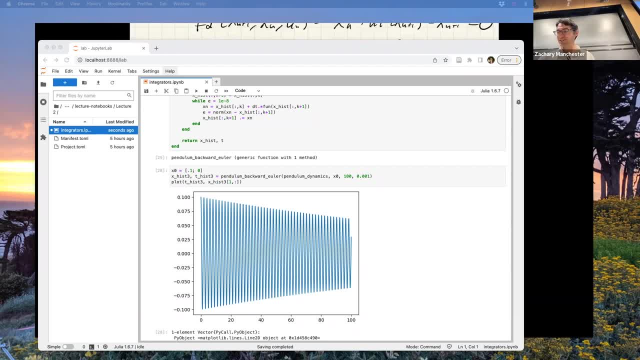 Yes, that does work out. It turns out you guys are really sharp. You guys are like: yeah, I like it. Okay, so cool that that was interesting. Where did this go? Let me get rid of this. We'll write down some stuff. 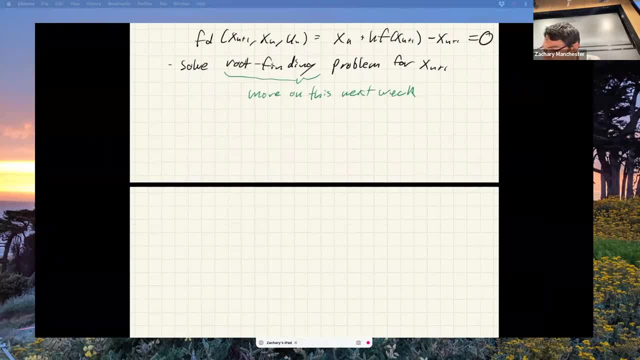 Okay. so what did we see this time? Opposite energy behavior. Here, right Discretization Adds damping And yeah, like I've just said out loud, this is unphysical, obviously, and wrong. But if you're running a simulator, 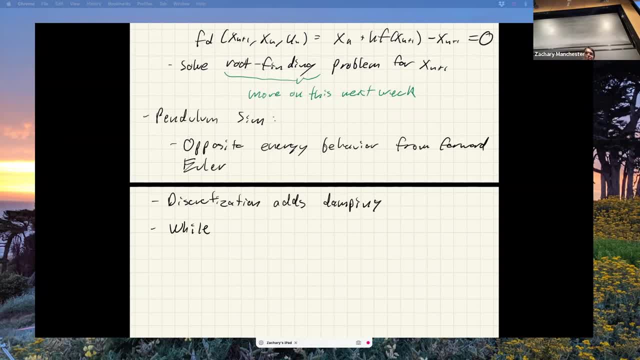 this looks sort of benign, Like if you're, if you're doing graphics right, you're playing a video game, This is benign and your video game character will still kind of look reasonable, Whereas the blow-up behavior will look stupid and make your 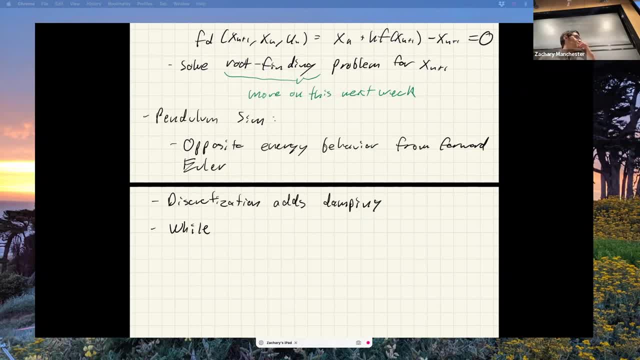 whole thing crash and be bad, right. So basically, like this has been historically the preferred simple integrator for things like video game engines, Many of the robotic simulators which historically have grown out of video game engines. because maybe not a great thing. 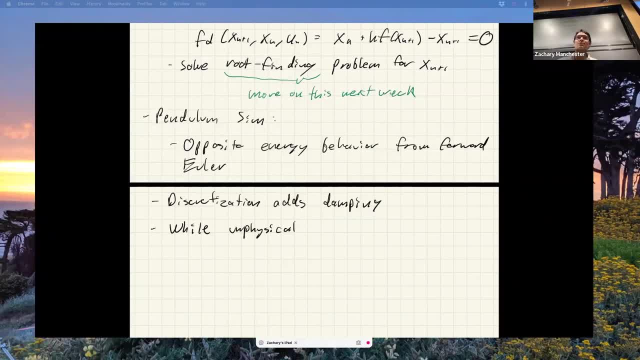 Yeah, So you have probably used this before, even if you didn't know it. If you've used any stock robotic simulator, Is the? is the directionality on the blow-up always the same for like periodic motion, Like, so the forward oiler? 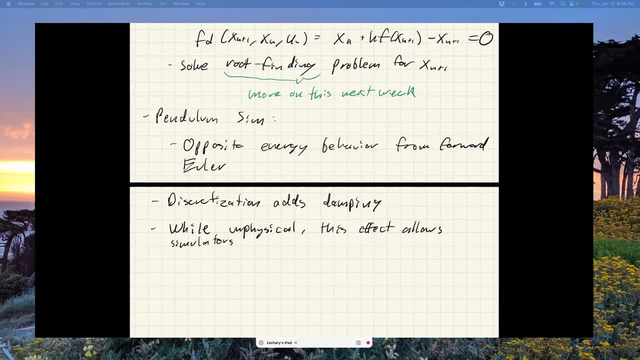 is always going to blow up and backward oiler is always going to damp. Yeah, it pretty much is. Yeah, So it turns out this is a general property of like oscillatory motion with either of these integrators and cartoon pictures: forward oiler always overshoots and oscillatory solution- and backward 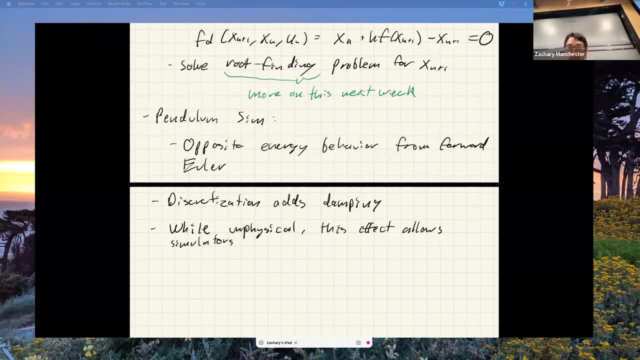 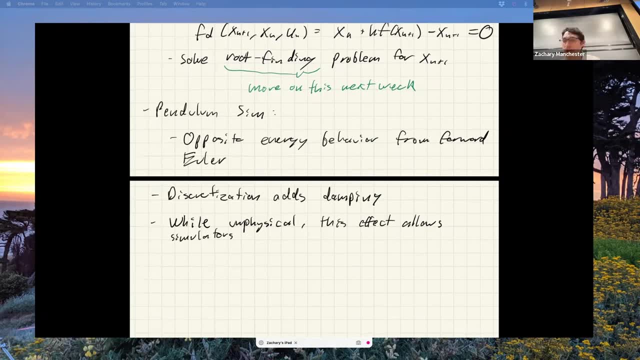 oiler always undershoots and oscillatory solution because they're fitting lines right And you can like prove this by looking at the next term in the Taylor expansion. you know like look at the line fitting basically like these things are like kind of sequence. 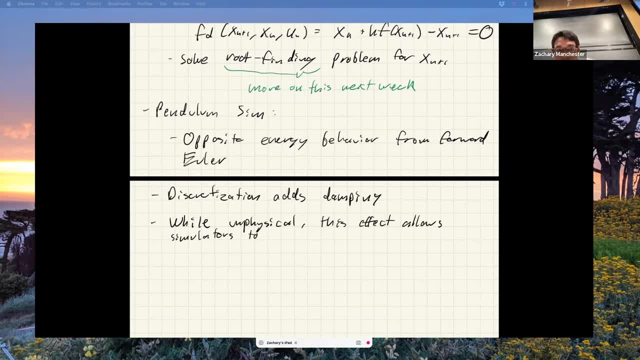 right, Let's see. So basically, the reason people like this and why it's using all these simulators is this: you know, the damping behavior means it's kind of always stable, So it means you can. you can take big time steps in the 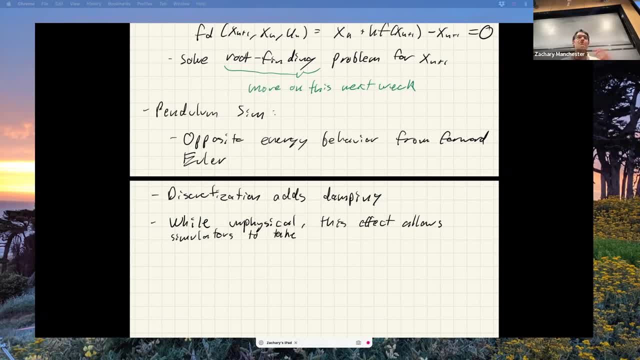 simulator and run the simulators really fast and it's cheap and all this good stuff, even if it's unphysical. the kind of unphysical behavior here is is like more benign right. So yeah, very common And sort of low fidelity. 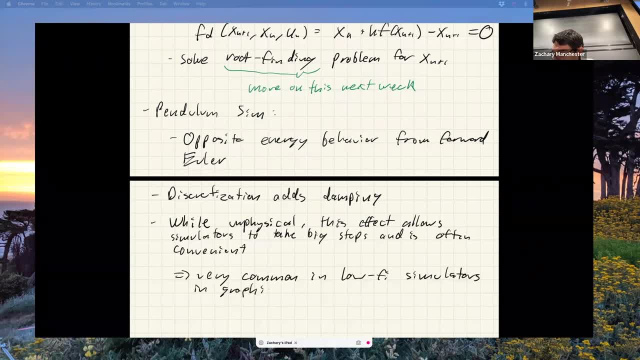 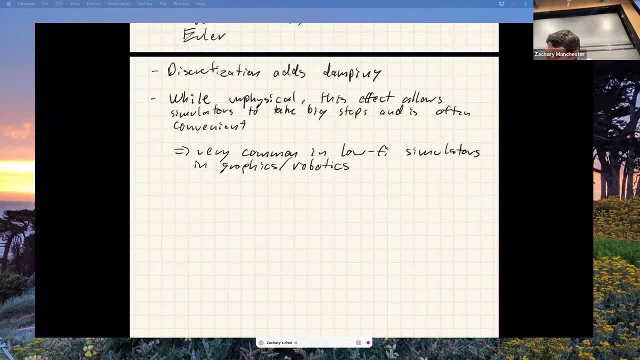 Simulators in graphics, game engines, blah blah blah, robotics- Okay cool, What else? So some more takeaway messages. Implicit methods in general are sort of- this is a very heuristic hand-wavy story so far, but these are often more stable than explicit methods. 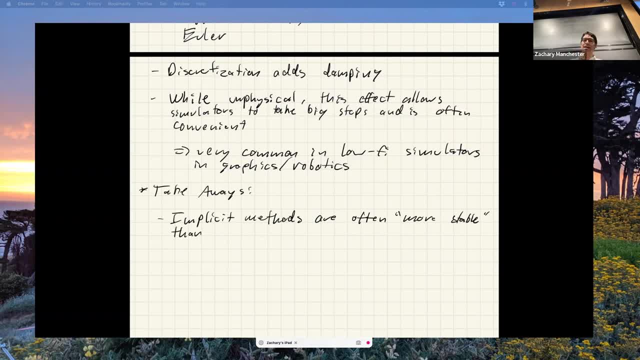 And there's a. there's a much more theoretically grounded version of the story where, basically, explicit methods can never be stable- all the time You can prove this- whereas implicit methods can. In fact, you can design implicit methods that provably always achieve like. 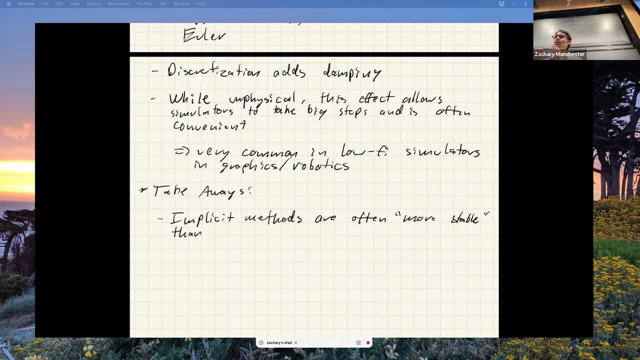 the correct energy behavior, which is cool Like you can make these always do the qualitatively right thing from an energy perspective. More to come on homework one, Yeah, So do you know about implicit versus explicit functions from math? So an explicit function is: y equals f of x. 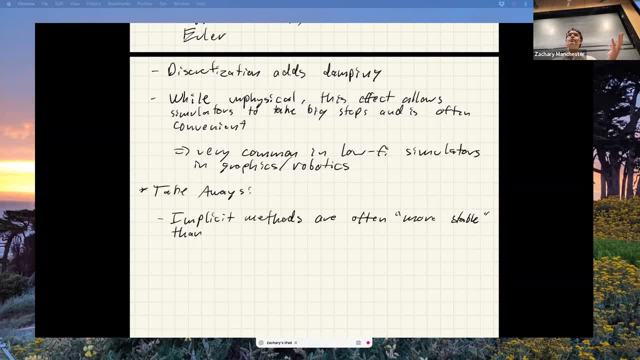 An implicit function is f of x comma. y equals zero. That's it, So it's just that right. So basically, the implicit ones are implicit functions of the state right. The explicit one is an: x equals one is an explicit function of: 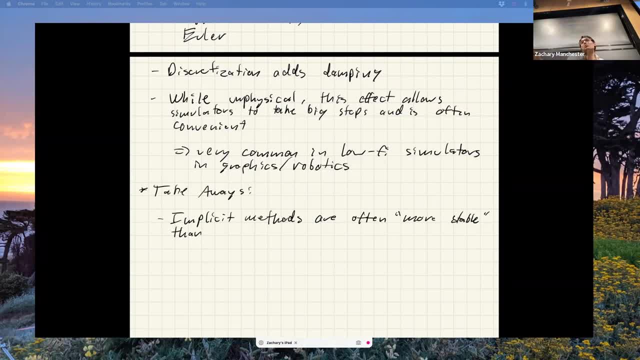 the current state. right, That's it. So basically the implicit versions. you have to solve a root finding problem to get the next step because it's buried inside this nonlinear function. Yeah, So implicit ones are more computationally expensive to run also. 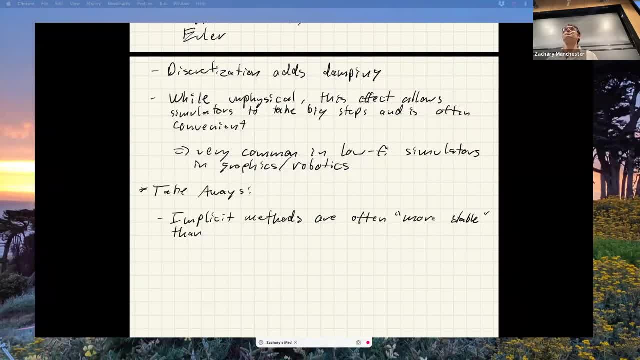 right, Yeah, I stable to mean that it's more like the simulation result is not a lot. Yeah, Like uh, no, I mean not accurate at all. right, It's qualitative. It's obviously not accurate right. 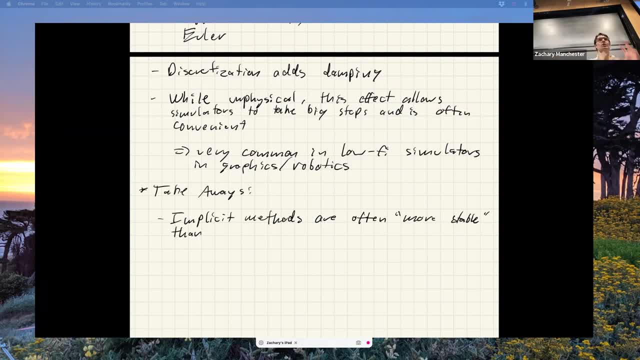 It's doing qualitatively the wrong thing, but it's not blowing up. Yeah, So stability. I mean very much this, this idea that the it's decaying towards zero, right It's, it's damped. 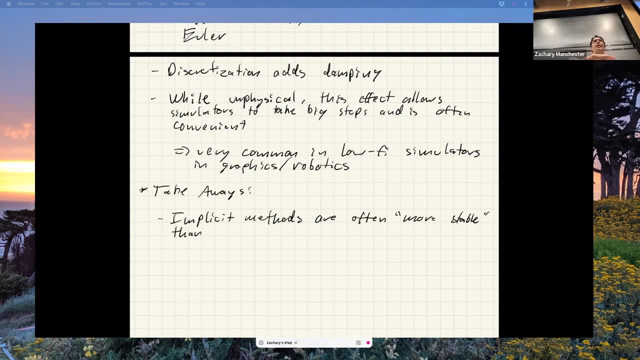 It's not going to blow up. I mean stable in the exact sense We've been talking about the last couple of lectures. right, I give values less than one, this kind of thing, right? Does that make sense? Yeah? 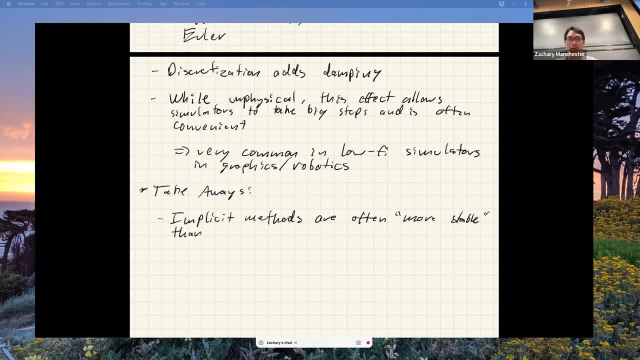 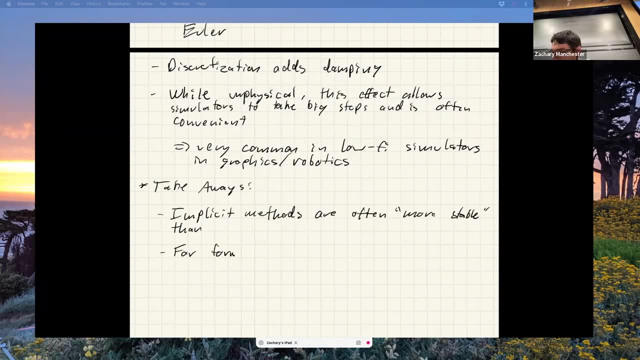 it doesn't mean more accurate. Okay, cool, Uh, okay. So yeah, a couple notes on this, though that aren't maybe obvious yet. for forward simulation, This should be maybe a little obvious. Um, the implicit stuff is more expensive. 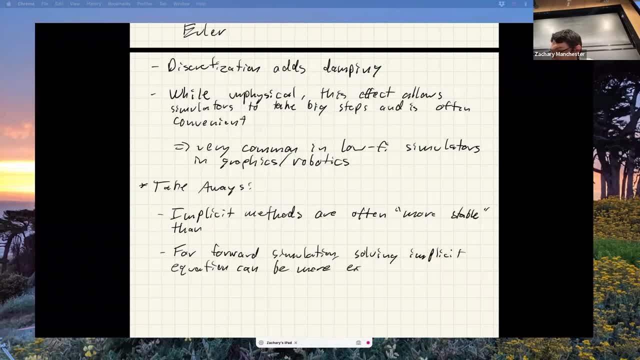 in general, but for a lot of control algorithms, um specifically, like direct methods or collocation methods, which you may have heard of, it turns out just the way those things work and the way they're set up. the implicit method is free and doesn't actually cost more. 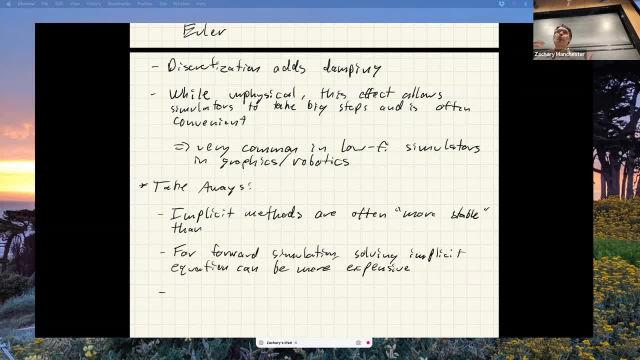 And so for a lot of these control methods we're going to talk about later, the implicit methods are preferred because of these nice stability properties and they are not more expensive in in in these algorithms, it turns out. So that's kind of what we're talking about them. 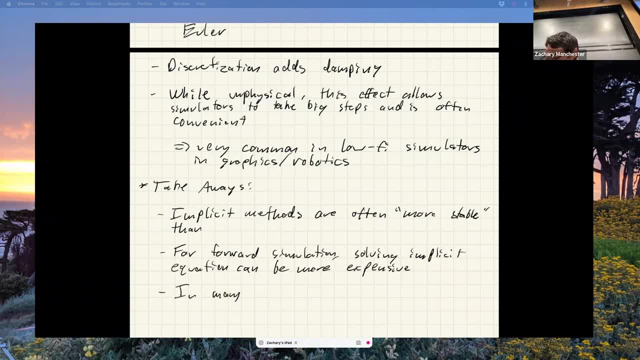 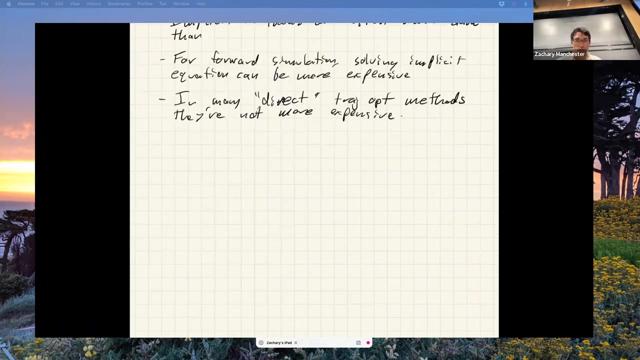 and these will come back later. Plus, they're also just common in general. So that's kind of fun, Okay, So in the last few minutes before we have to leave, we're going to talk about one last kind of little little topic that will be kind of important for us. 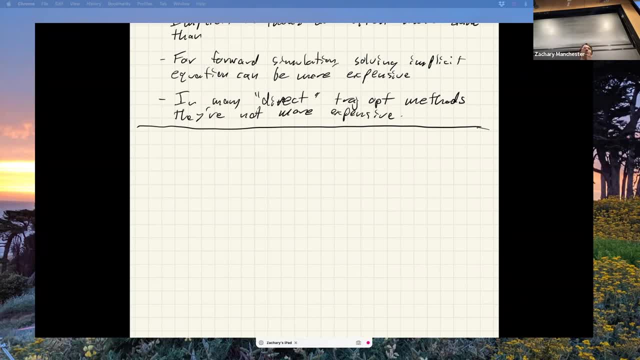 So we're not. we talked so far. we talked about discretizing dynamics and and discretizing state trajectories, right with like piecewise, linear or cubic splines, right with these RK methods. Now we're going to talk about discretizing controls. 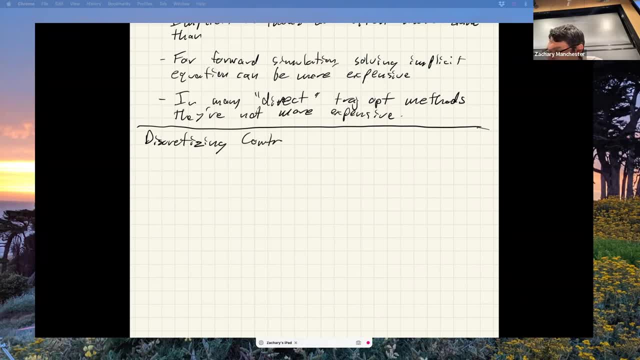 which is a little different, it turns out. So yeah, We also have to do U of D. Okay, So the simplest option is called a zero order hold. So this literally means UK equals UT equals UK for T, basically between TK and TK plus one. 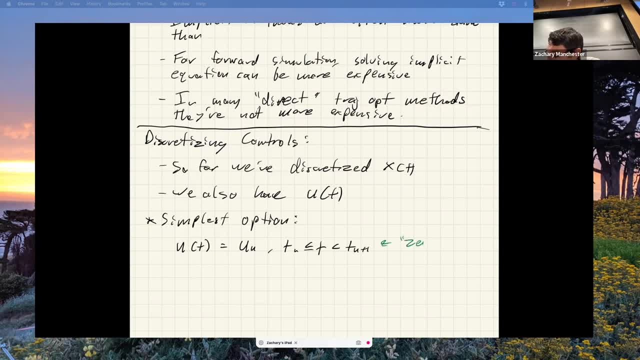 So this is called zero order hold And the cartoon picture of this is the following: So I have like T and I just do this kind of thing Makes sense. So it's piecewise constant And at the next time step I just stick it at whatever the next value is. 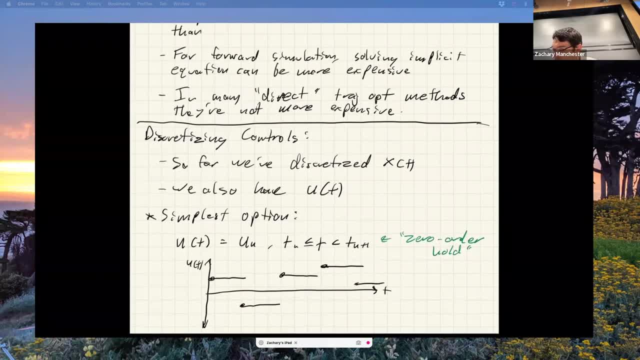 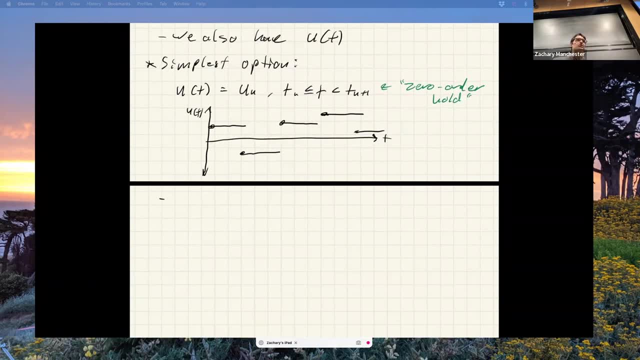 And it just hold it over the over the time interval right. Super easy, super straightforward. This is really really common, In fact, in pretty much all actual on hardware implementations. this is what is actually happening at the lowest level. 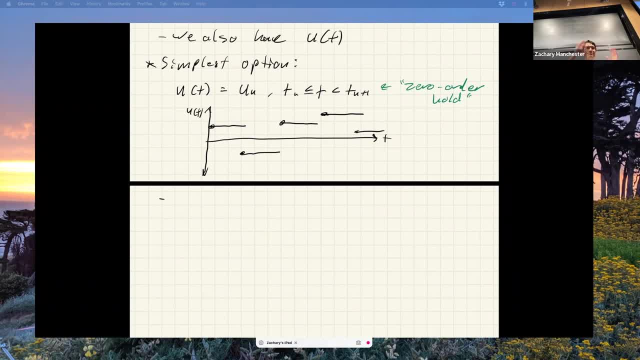 You have some you know DAC or whatever. That's like taking this you know signal from the computer and like just and actually spitting it out as a voltage on you know whatever, or current of your motors For the most part. 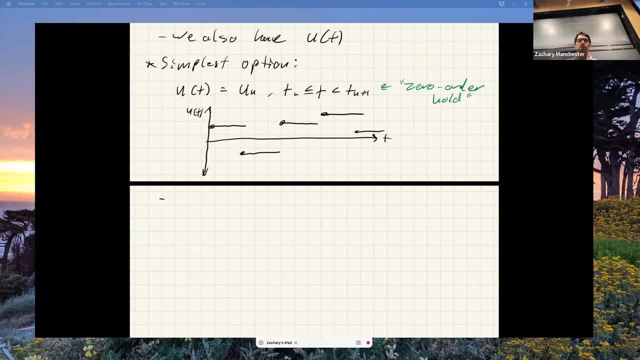 those are doing this at the lowest level, at whatever you know hundreds of Hertz or kilohertz Hertz rates, So it's also just easy to implement right. But when we're doing, say, offline optimization and this kind of thing, 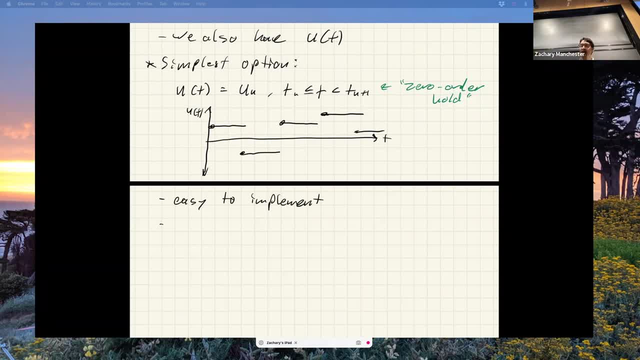 if I'm trying to capture some wiggly continuous signal accurately I have to take a lot of sample points, Like I have to take really small time steps to get a good approximation of my continuous signal with a zero or hold Right. So that's kind of the downside and why we maybe want to. 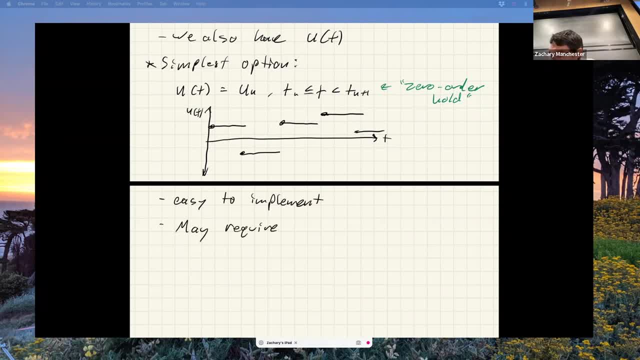 do other things. Basically, we may want to do other things because it'll let us take bigger time steps in our simulation or in our solver for our optimal control stuff. So and the, by the way, the lingo and controls for like time step very often is not. 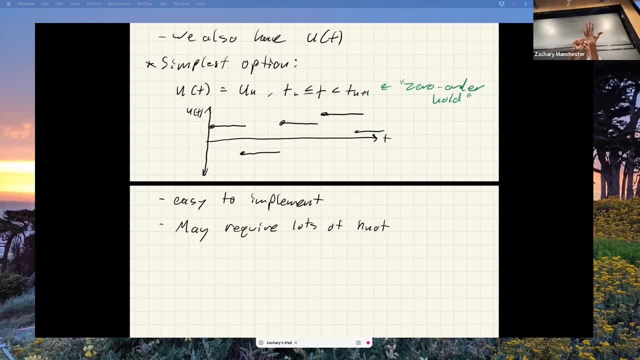 point. I don't know if anyone's heard this, but when I say not point, I mean basically, but I mean that the times, the discrete time steps- I think that comes- for that terminology comes from us- from splines, like they're not points of the control points right on the spline, or 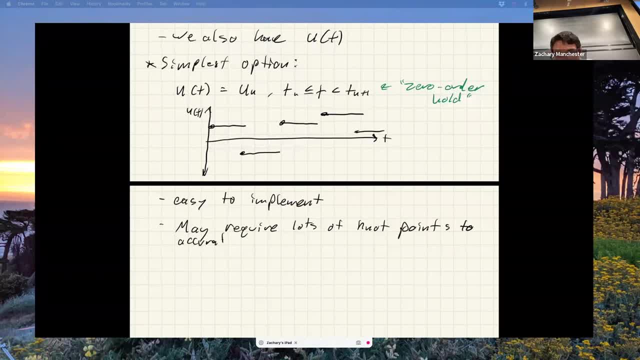 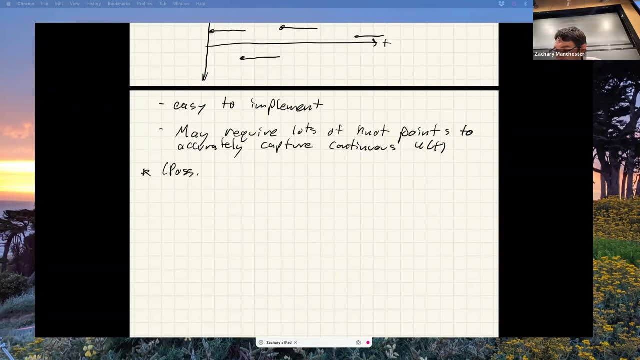 whatever. Okay. so then like another option, which is fancier, but I'm going to caveat this with: possibly Better option is what's called a zero order hold. So this one is just linear interpolation instead of hold it constant. So mathematically looks like this: 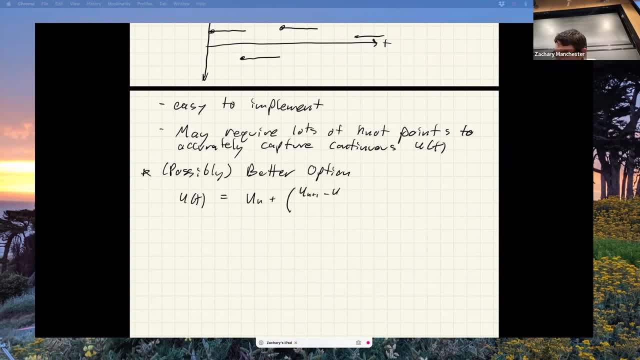 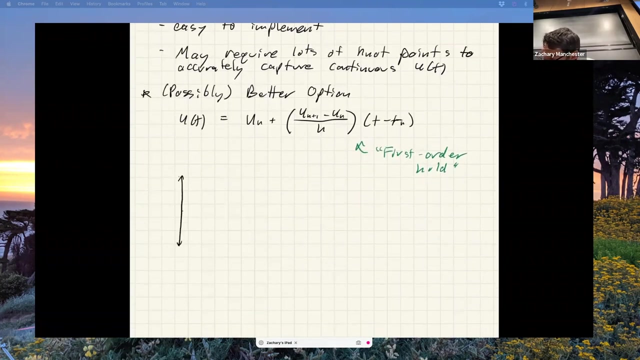 I'm going to basically take, you know, UK plus one, As you gave her aged times. So this is called First order Hold And the cartoon picture is something like this, So maybe I start here. I go like this: 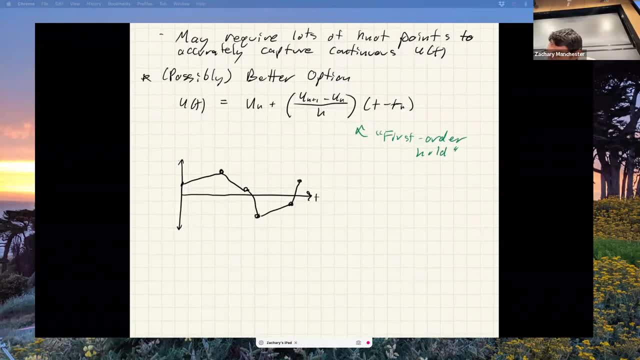 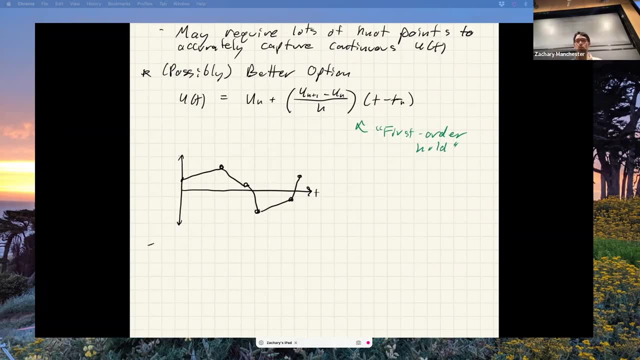 Get the idea. So the the reason you might do this right is this is now, you know, kind of interpolating maybe a little better and we might be able to Approximate a continuous U of T with fewer, not points like this. 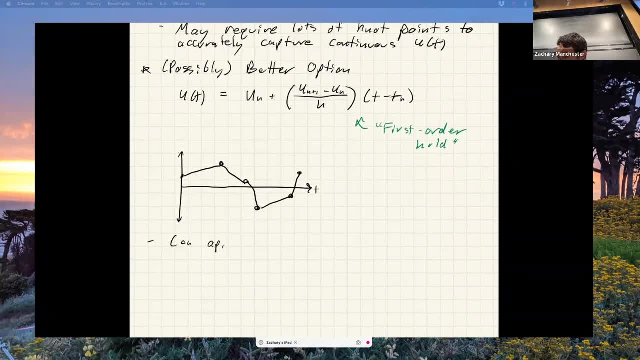 right. But oh yeah, I guess a couple of other comments right. This is basically, you know, almost no extra work over the zero order hold. So you know, computationally pretty easy also, And this is actually very common. 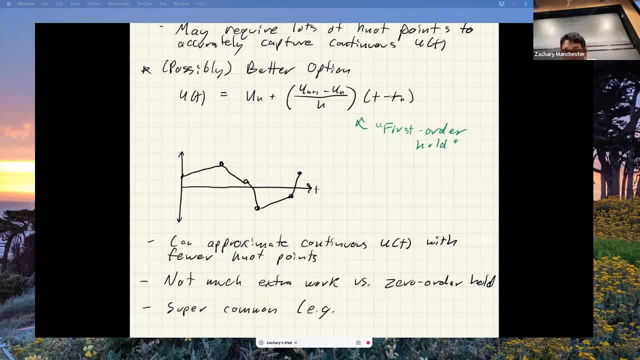 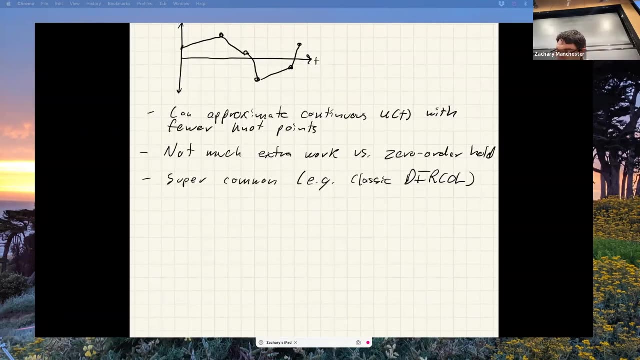 As just one example, the classic direct collocation method, which we'll talk about later, uses this. So let's say so, yeah, you, and I guess the sort of other options that you might think about- like the obvious game to play here. 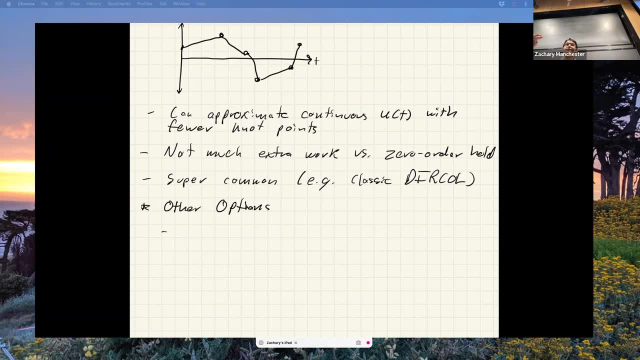 which is kind of the one we played with. the state right Is: you can keep doing this right. I went from zero to hold to first order linear interpolation. I can do arbitrary high order spline interpolation on these guys And this has been done. 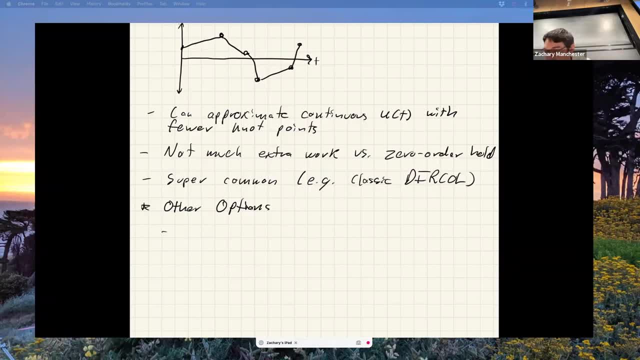 There's algorithms that do this, So you can do it And you would hope, right, that that would give you some nice advantage where you can take fewer and fewer now points with higher orders, which kind of does plan out with our runge kind of methods. 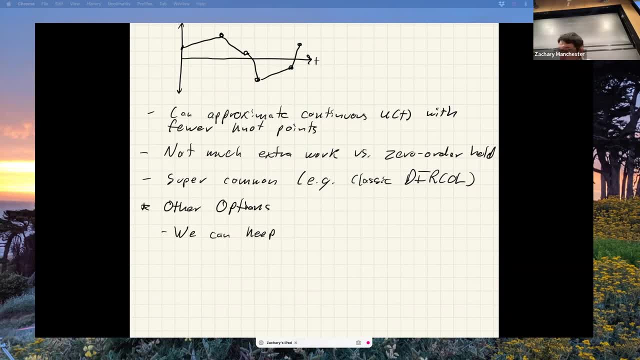 right, We said RK four with the cubic splines is dramatically better than an oiler which is doing the linear thing. Yeah, Yeah, Yeah, Yeah, Yeah, Yeah. um, but there's a big but here. so with the states, they're generally these smooth things right in. 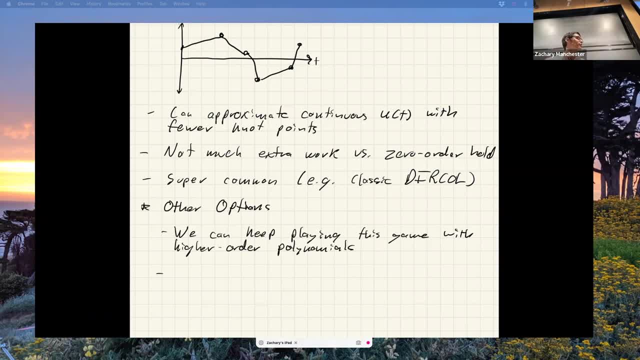 most cases modulo, like contact interactions with impacts or whatever. um. so it makes sense to use nice high order, smooth, polynomial for that. but controls, it turns out in many, many applications are just not smooth. uh, it's very, very common to have uh so-called bang bang solutions where 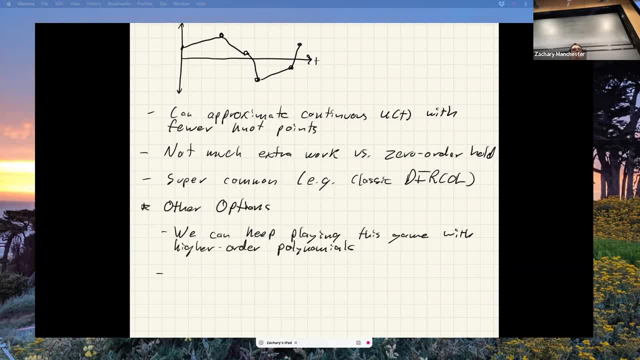 you're basically railing up against your torque limits and then like railing against your torque limits the other way right, full gas, full brakes. like that is very common in control. so in those situations the solutions, the u of t, are not smooth, so trying to fit a polynomial to them, a very high. 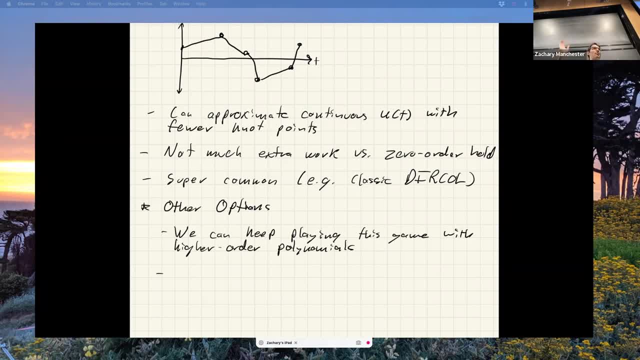 order. smooth polynomial doesn't really work. you get like the runga phenomenon kind of stuff. this kind of stuff happens. so it turns out that, because of just, the things you're trying to approximate are generally kind of gross and non-smooth. it's just not worth. 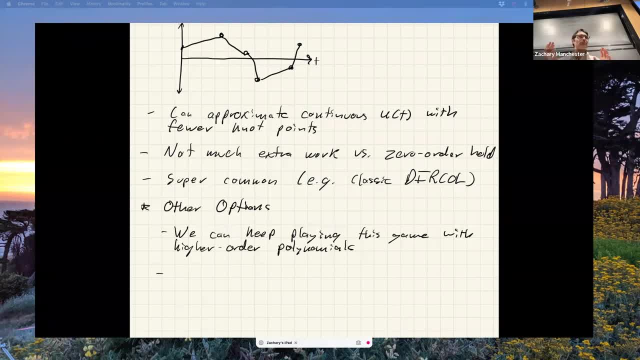 it, and so we usually use zero or hold and first order hold in most practical applications. there are exceptions to the rule, like in aerospace applications where you have like continuous low thrust or whatever. this game does work out favorably and maybe it does make sense there to.